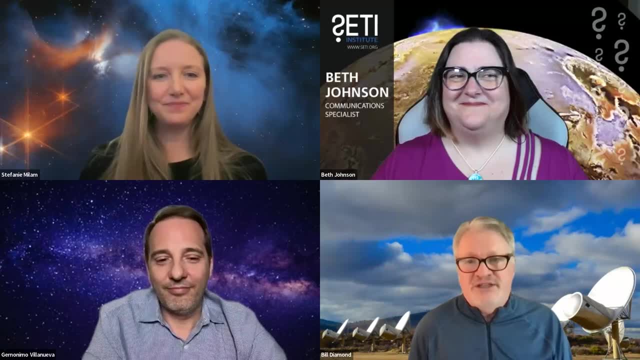 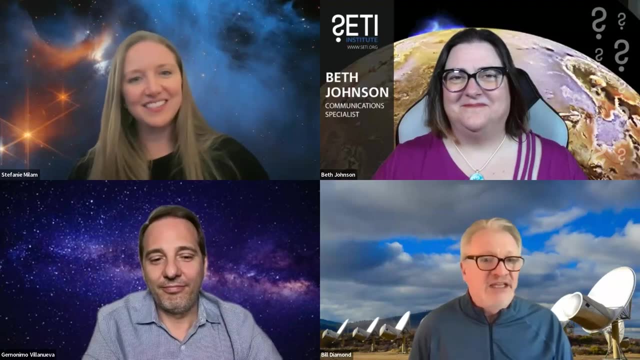 have you with us for this evening's SETI Talks. Tonight, we're joined by two scientists from NASA's Goddard Space Flight Center in Greenbelt, Maryland, to tell us more about this extraordinary telescope and the new discoveries and understandings that it will undoubtedly provide. Our guests will be. 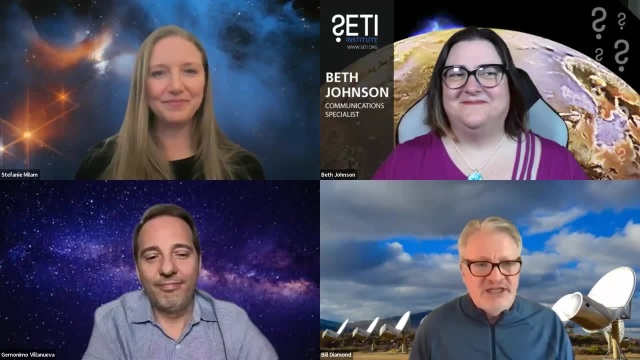 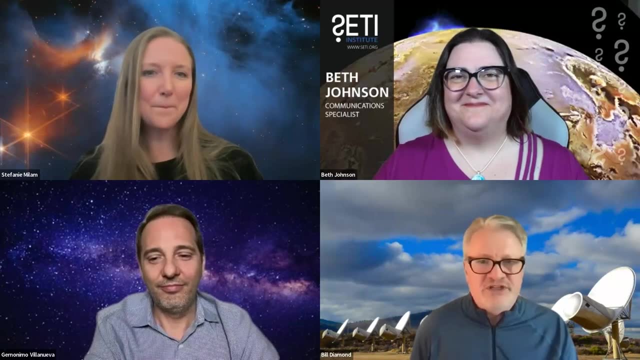 introduced by our own communications specialist, Bill Diamond, who is the CEO of the SETI Institute For our regular SETI Talks attendees and new guests joining us tonight. let me remind you that you can post questions using the Q&A feature at the bottom of your screen and we'll do our best to address as 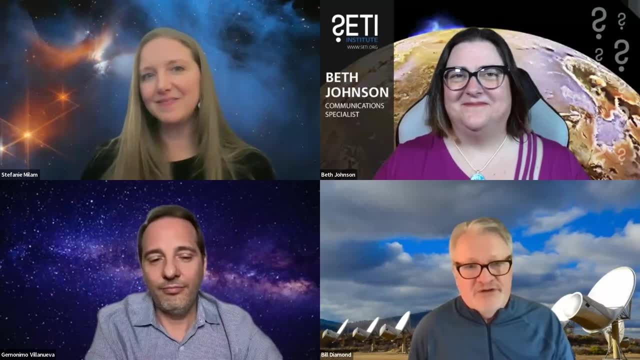 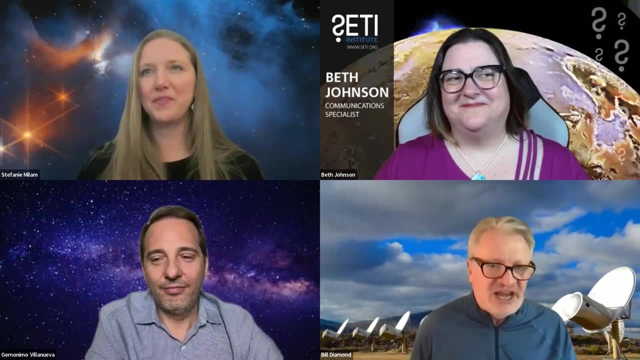 many as we can at the end of the panel discussion. I also want to remind you, as we've already seen folks doing: we love to know where you're joining us from, So please use the chat function and tell us where on this planet you are. or if you're on some other planet, let us know that as well. 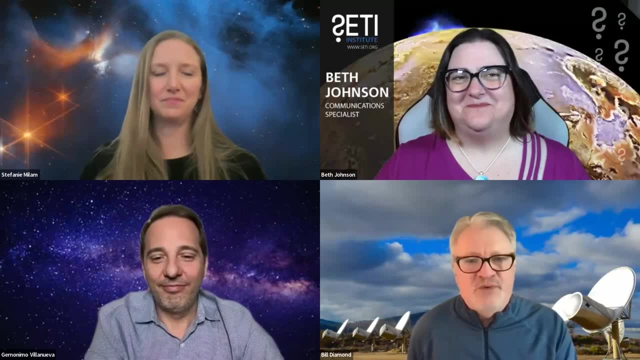 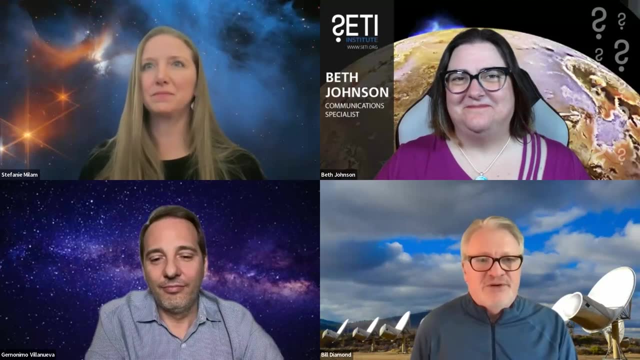 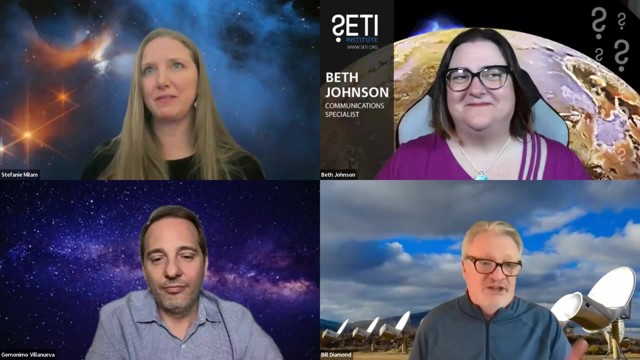 And whether you're in a place where you also happen to have watched the launch of the James Webb Space Telescope. So our SETI Talks lecture series is a production of the SETI Institute in Mountain View, California. It's made possible by the generous support of people like you, and you can. 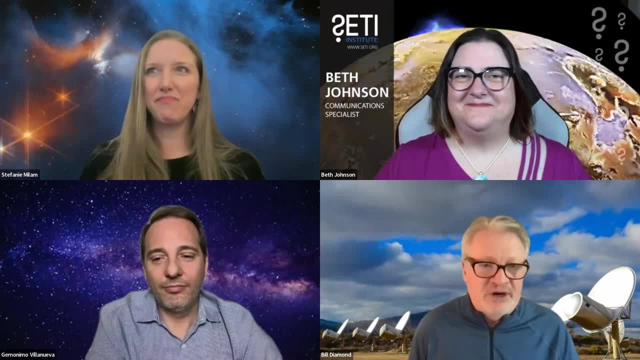 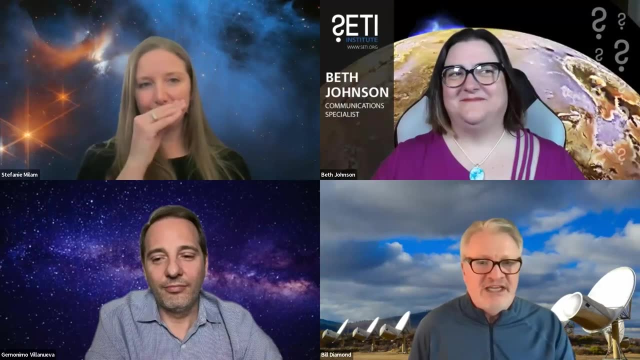 get involved and learn about our mission, support our work, sign up for our weekly newsletter. we call Journey and you can do all of this online at our website at wwwsetiorg. Tonight's talk is sponsored by the many donors and friends of the Institute who fund our outreach. 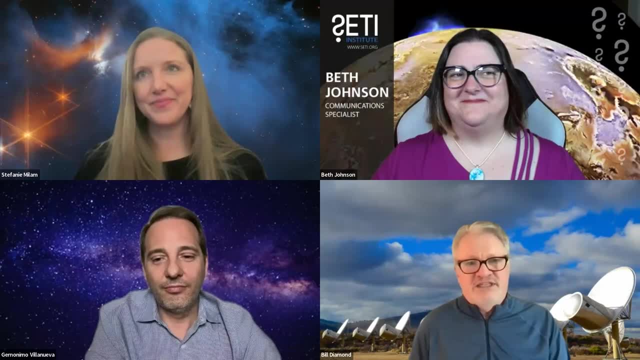 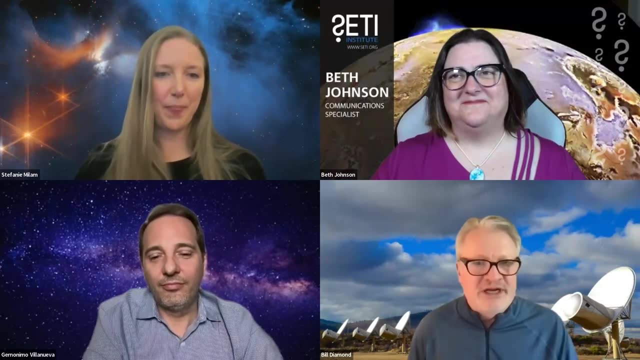 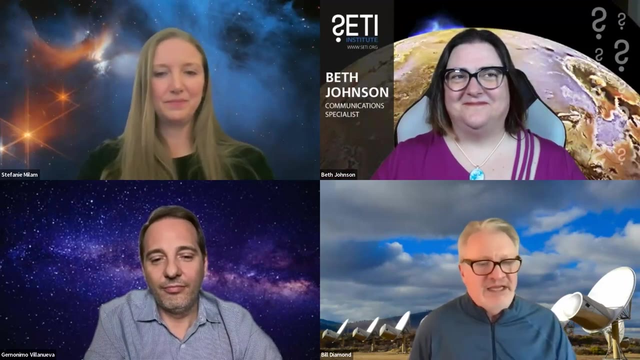 programs through their generous gifts. Their gift to us is a gift for all of you and we're very grateful for their support. If you'd like to personally sponsor a SETI Talk or learn more about how to sponsor our work, visit us at SETIorg or contact us by email at info at SETIorg and get 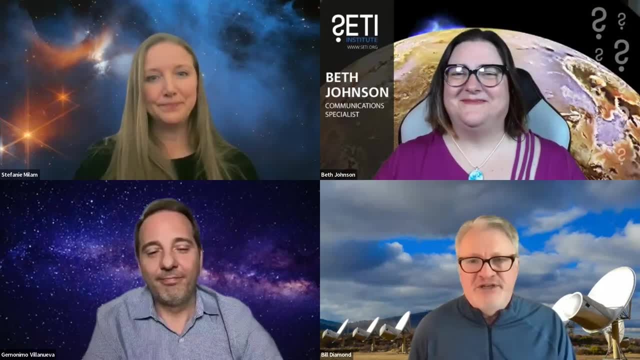 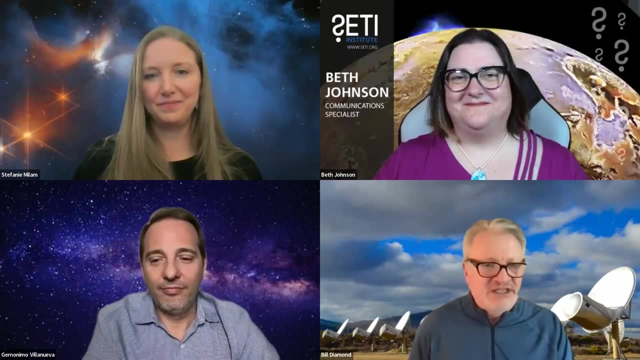 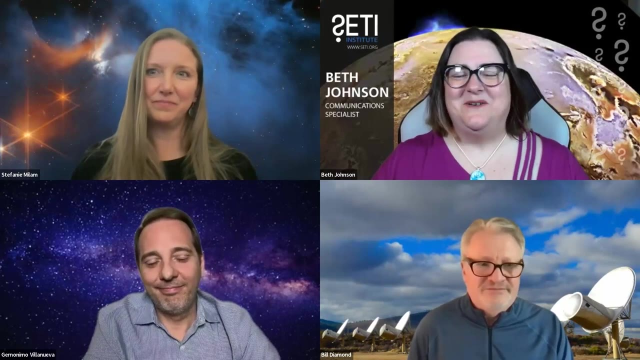 involved. So before turning the podium over to Beth, let me remind you to check the events calendar on our website for information about the SETI Talk. Thank you, Bill. Once again, welcome everyone. I'm Beth Johnson, a communications specialist here at the SETI Institute and your moderator for tonight. 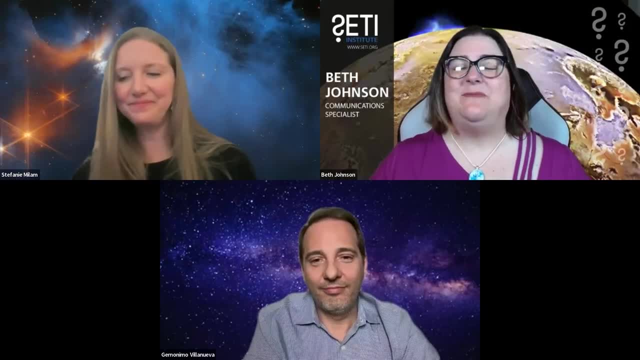 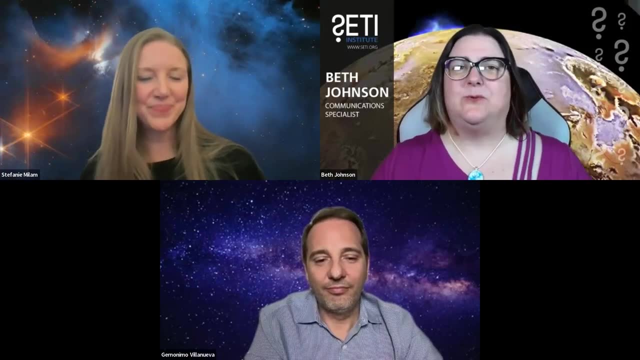 Again, please let us know where you are watching from in the chat and make sure you put your questions in the Q&A and we'll keep track of both of those. We'll leave the chat on for a few more minutes while you let us know where you're watching from and answer some of Bill's questions. 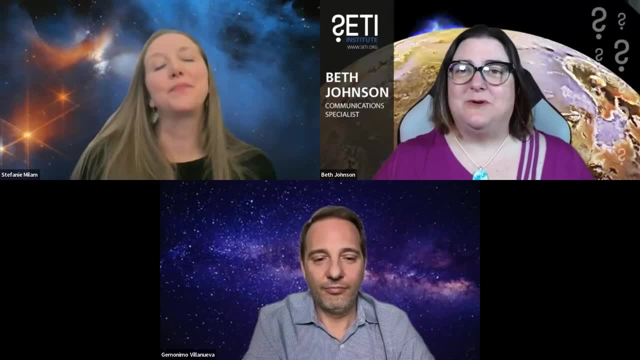 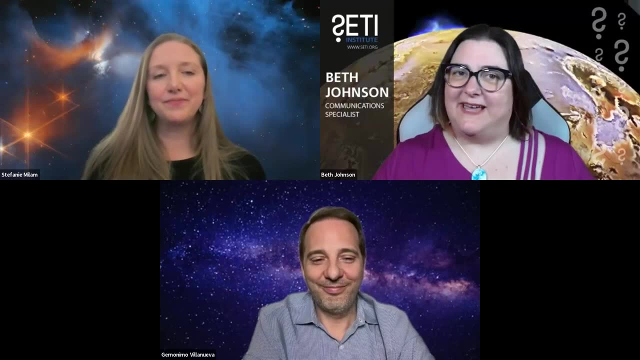 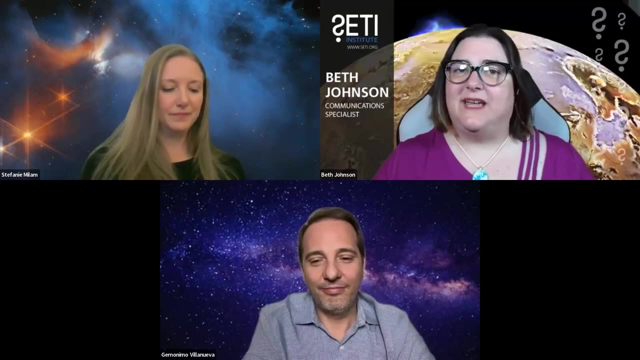 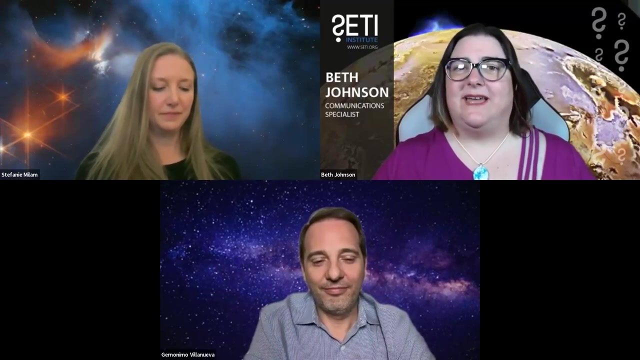 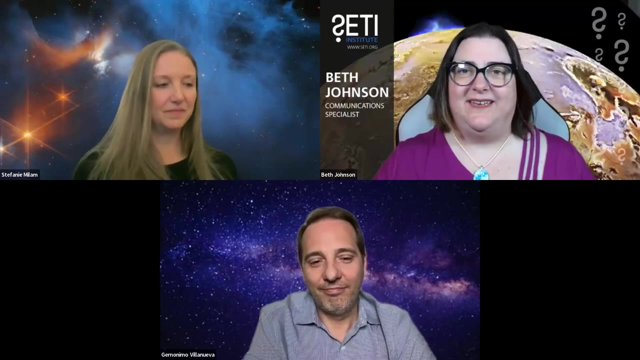 Lecture No 3: heat continues. Robert Jones Have a great day Recording The CCTV signs of life beyond Earth, and our two guests are at the forefront of the research. 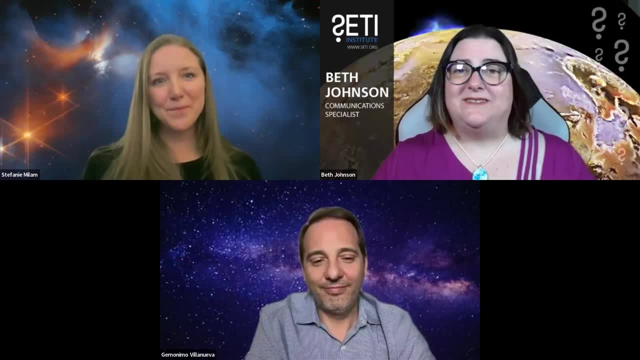 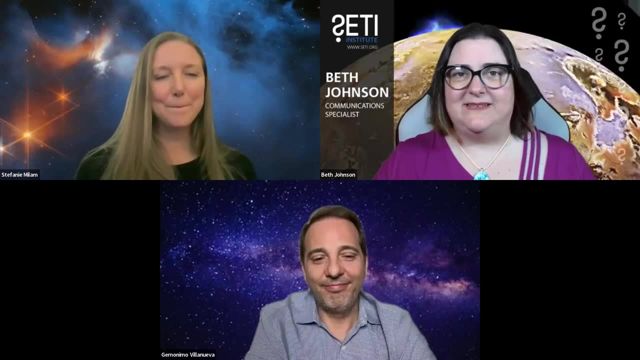 Geronimo Villanueva is a planetary scientist and astrobiologist at NASA Goddard Space Flight Center. He specializes in the search for organic molecules on Mars and on icy bodies. He is the principal investigator of the Planetary Spectrum Generator, co-PI of the Comet Interceptor. 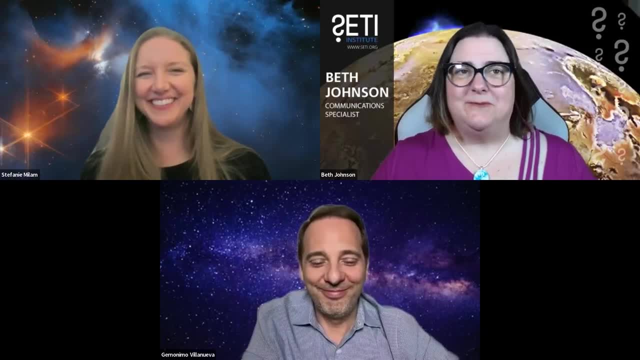 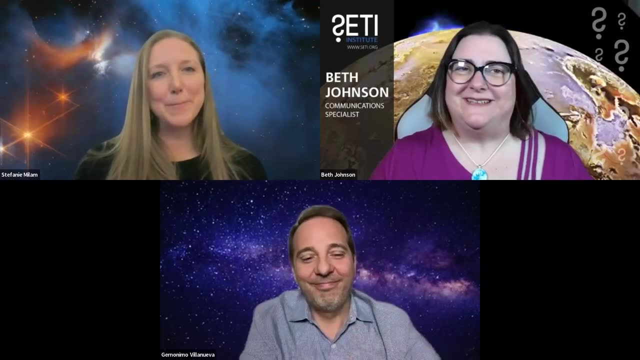 Mission, co-investigator of the ExoMars Trace Gas Orbiter Mission and leader for Mars and Ocean World Studies for the James Webb Space Telescope. Welcome, Geronimo, and thank you for joining us today. Thank you, Beth. 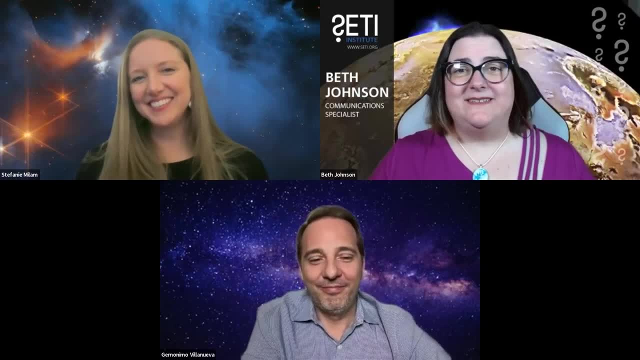 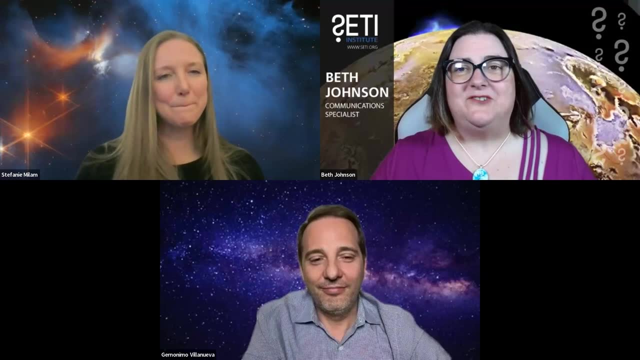 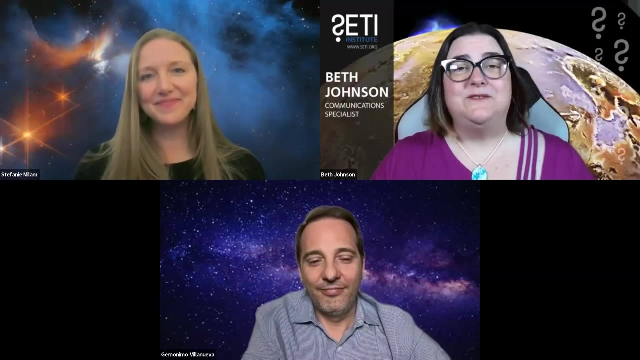 Also joining us is Stephanie Milam, who is a planetary scientist and astrochemist who has made significant contributions to the study of comets and the early solar system. She received her PhD in chemistry from the University of Arizona, moved here to SETI as a research scientist and postdoc at NASA Ames and went on to work at NASA's Goddard. 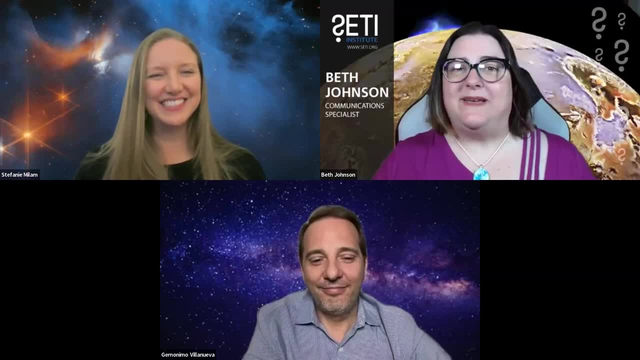 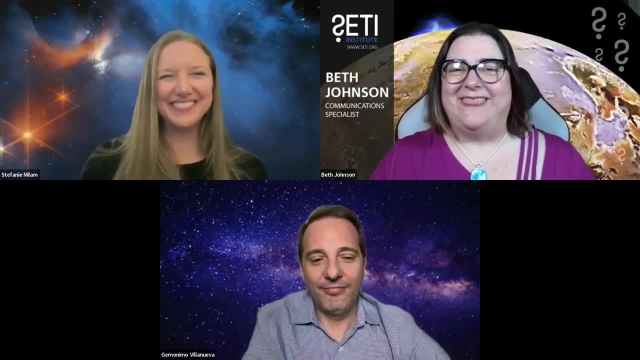 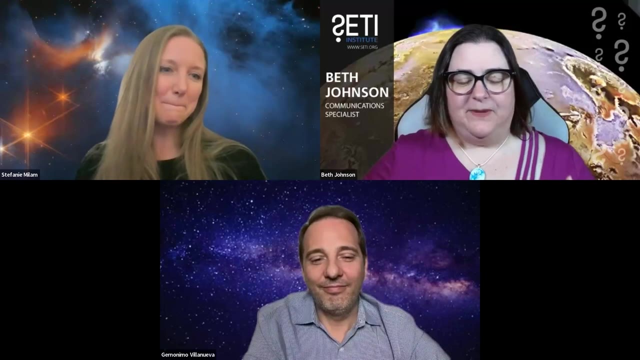 Space Flight Center Milam uses space and ground-based telescopes to observe and analyze comets, Providing insights into their chemical compositions and origins. Thank you for joining us, Stephanie. Thanks so much for having me. So now that we have met both of you, we've we discussed this. 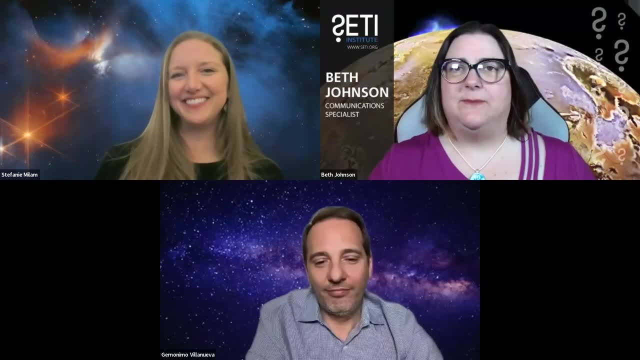 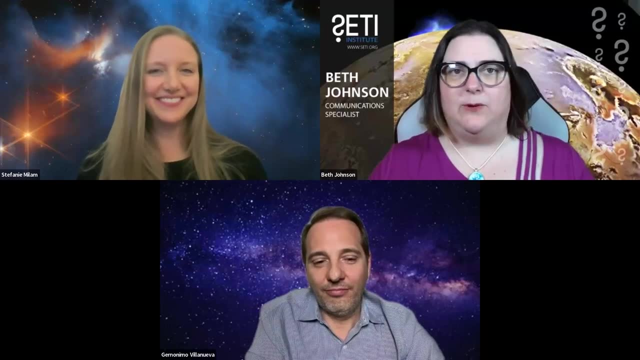 We want you to each give us sort of like a five-minute breakdown of some of the things that we're going to talk about tonight. Stephanie, I believe you are going to start and you're going to talk to us about James Webb and why it's important and what it's doing. 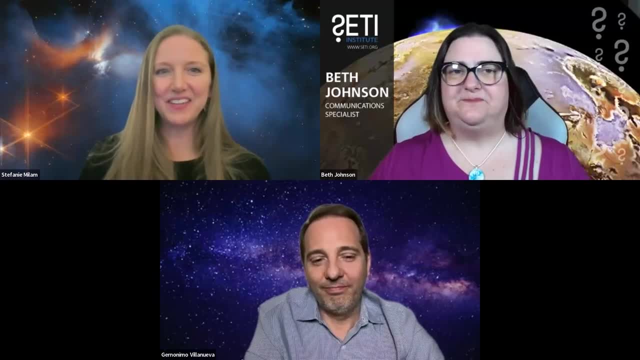 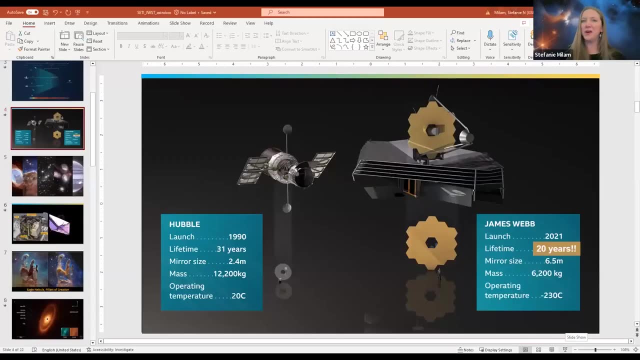 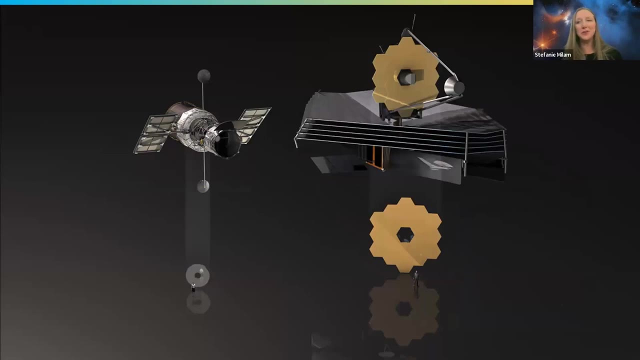 So why don't you go ahead and share your screen and kick that off? All right, let's make sure I can do this properly. So one of the things about the James Webb Space Telescope that most people already know, or hopefully know, is that it's it's dubbed the successor to the Hubble Space Telescope. 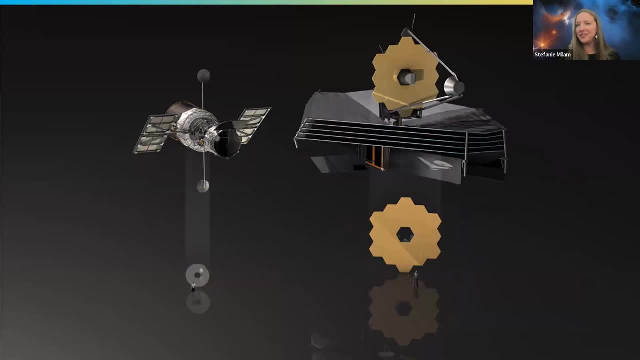 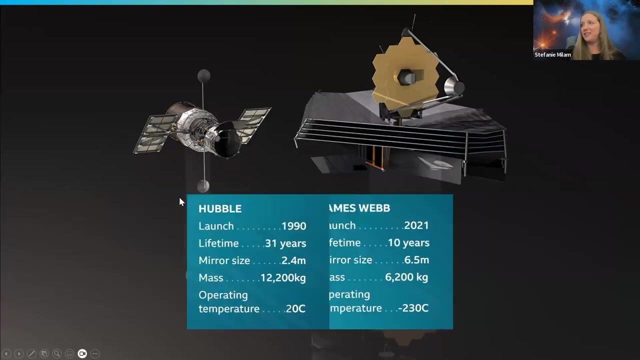 And some key things that are really really different and such that it's not actually a successor. One is: it is an infrared space telescope. We we have a large, 6.5 meter diameter telescope that is coated in gold, which is extremely 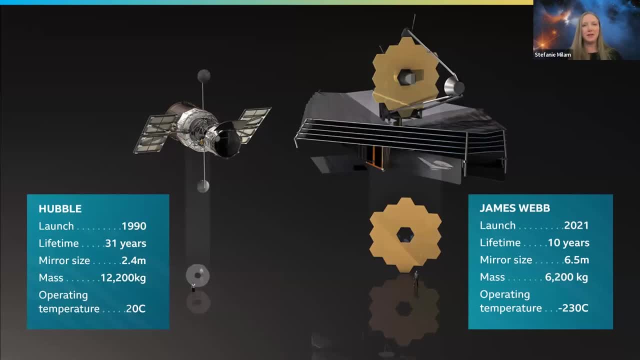 reflective at infrared wavelengths And it's an exceptionally massive space telescope, such that we had to fold it up like origami to launch it. We are hoping to have the success that the Hubble Space Telescope had, with Hubble already operating over 30 years. 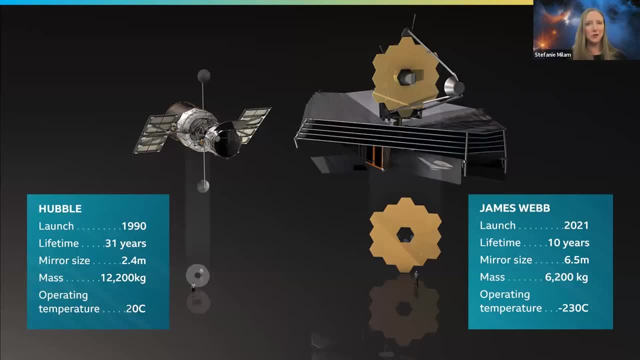 Now, we had such a beautiful launch Christmas of 2021, that we now believe that we have an operational lifetime of over 20 years, which is absolutely significant for the next generation of astronomers, astrophysicists and planetary scientists to be able to use. 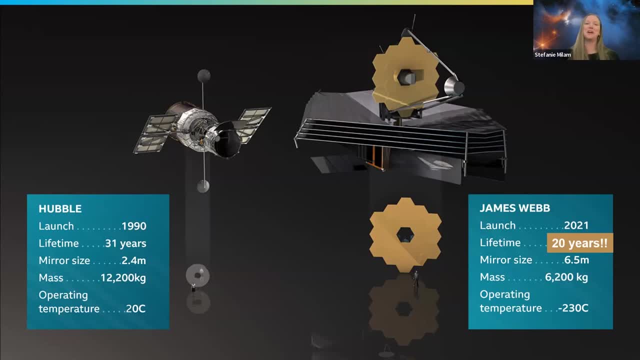 this telescope the way that you know. I had dreamed of and got the opportunity to use the Hubble Space Telescope and now getting my fingers wet with the James Webb Space Telescope. I also like to point out one of my favorite facts about the observatory is that, even though it's this big, it stands, you know, three stories high. the sun shields as big as a tennis court. it's only half the mass of the Hubble Space Telescope. 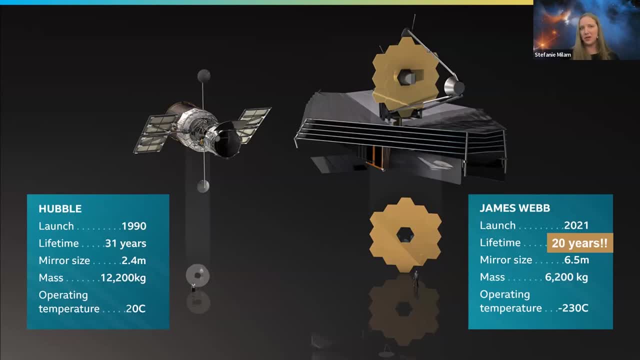 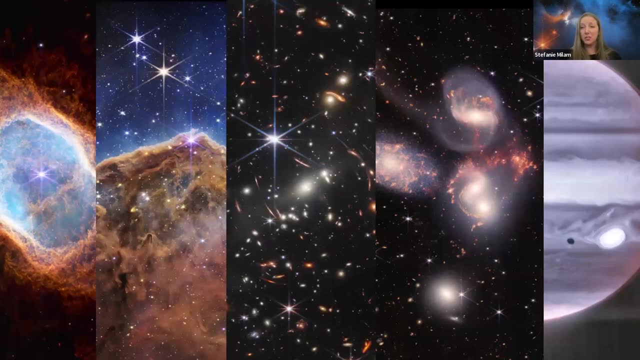 So a lot of innovation and technology went into building this observatory, And a lot of that was actually such that we could study not only the first galaxies and stars of the universe- which is what drove the design of the observatory- but also to study 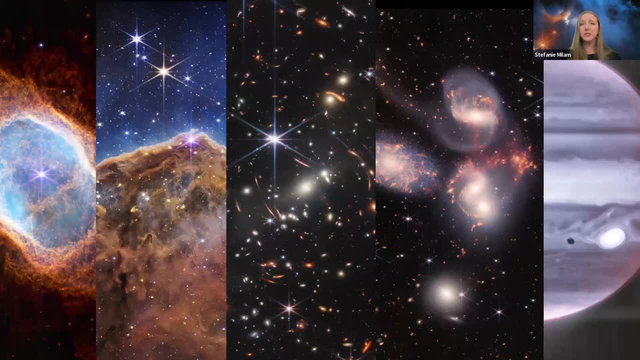 And a lot of that was actually such that we could study not only the first galaxies and stars of the universe, which is what drove the design of the observatory, but also to study Star stellar evolution all the way from the birth of stars to the death of stars, to the birth of planets, to now planets orbiting other stars, but even objects in our own solar system. 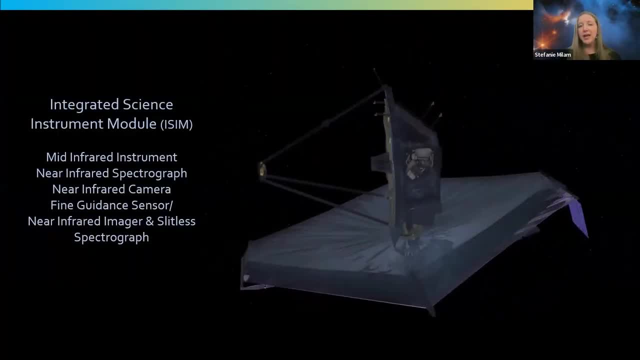 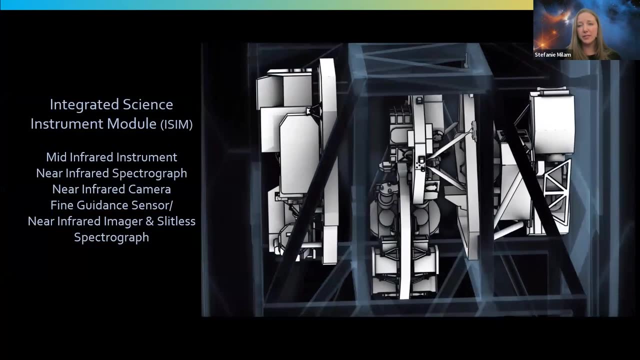 So the heart of the telescope is the most critical component, And I want to emphasize that we have science instruments that were designed to primarily study the first stars and galaxies, but when JWST was first drawn, on the back of a napkin at a bar, So the heart of the telescope is the most critical component, And I want to emphasize that we have science instruments that were designed to primarily study the first stars and galaxies, but when JWST was first drawn, on the back of a napkin at a bar, 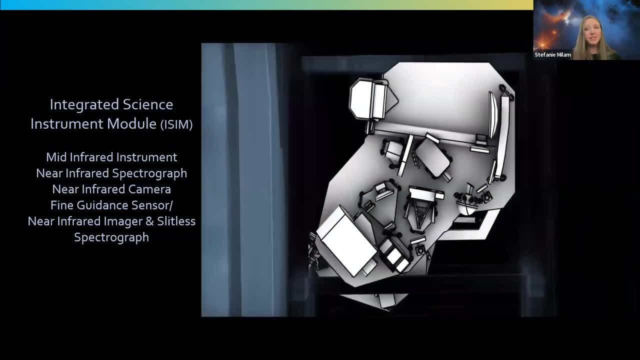 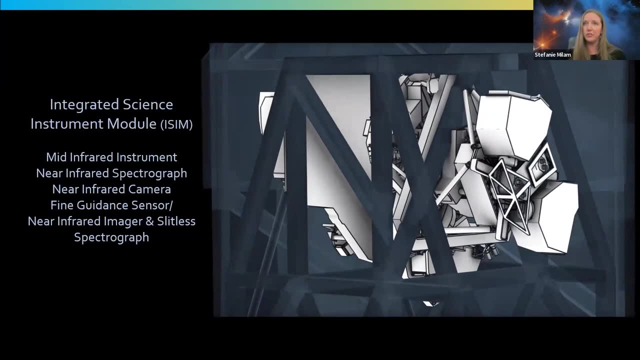 planets around other stars weren't a known thing, So a lot of technology and innovation had to go into implementing the detection and characterization of planets around other stars. So even though we have this fantastic suite in our heart of our telescope to just to study these distant galaxies, we also are now designed and optimized to study planets around other stars. 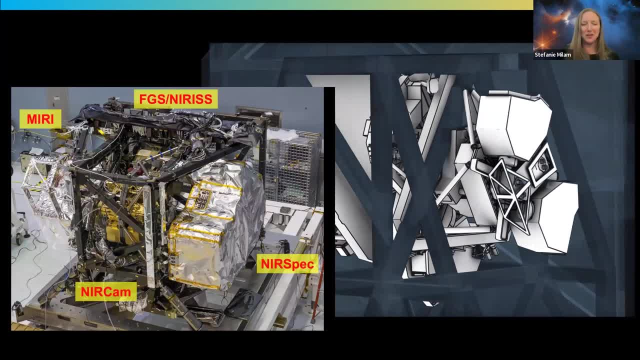 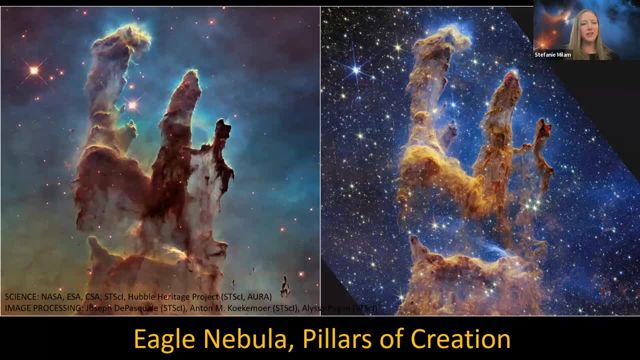 And it's a complete jumbled mess whenever you look at the instruments themselves. But we put them in a nice tight package so that we could fit onto our rocket, And you've seen a number of the images that have already come through, the comparisons of what we can do at infrared wavelengths compared to what we had with the Hubble Space Telescope at optical or visible wavelengths. So this is my favorite, most critical. 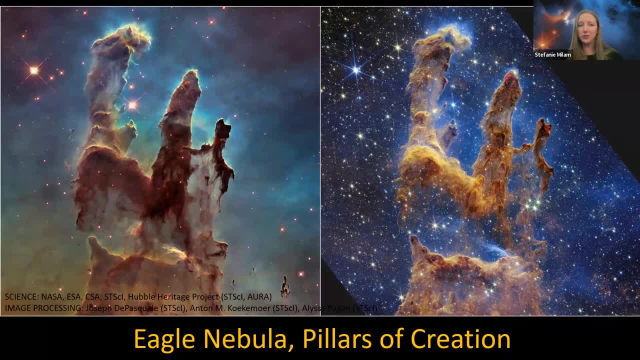 comparison that I've seen to date, and that is of the Pillars of Creation, showing you, on the left hand side, the Hubble Space Telescope version at optical wavelengths, and then the infrared version from the James Webb Space Telescope, revealing new planets that are actually being born throughout star formation, in these giant clouds of gas and dust. 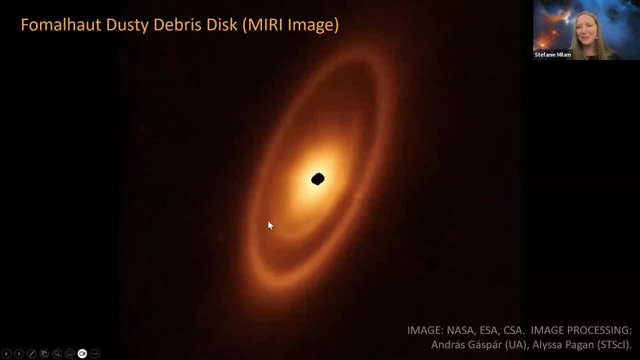 But not only can we see inside of these clouds, we can also now see planets being born, And we released this beautiful image last week, or the week before the Fomalhaut debris disk. So this is the first time we've actually seen an asteroid belt in another planetary system. 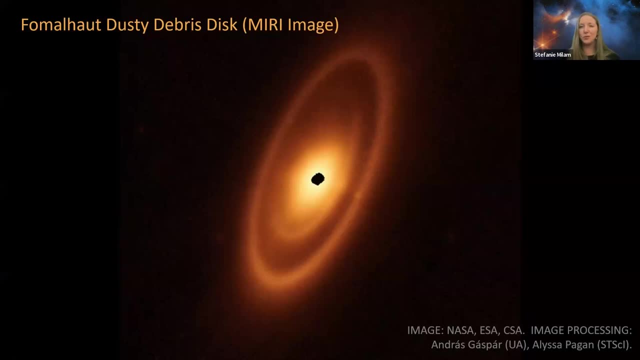 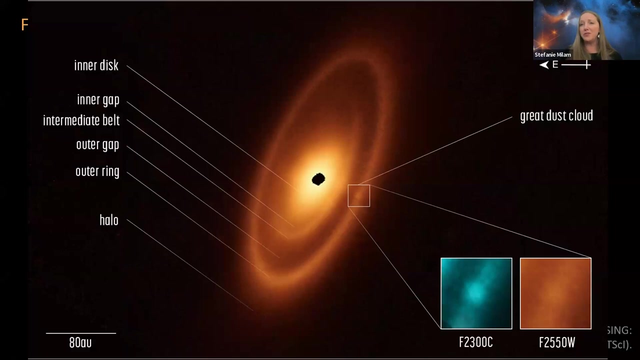 With this type of resolution, such that we can now dig in deeper with the James Webb Space Telescope data and see if there's actual planet formation occurring. We really want to know what these planets are made of. Do they look like our own? What are the intricate details of the asteroid belt or the Kuiper belt, of these fantastic disks? 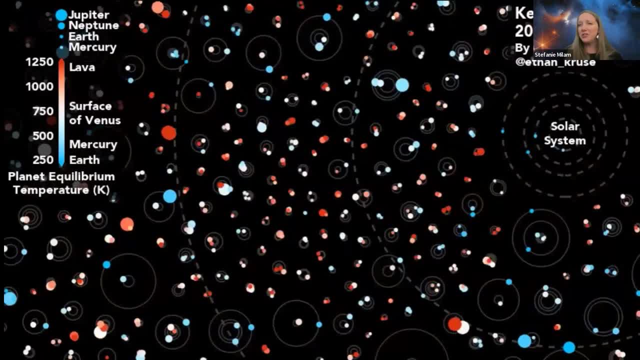 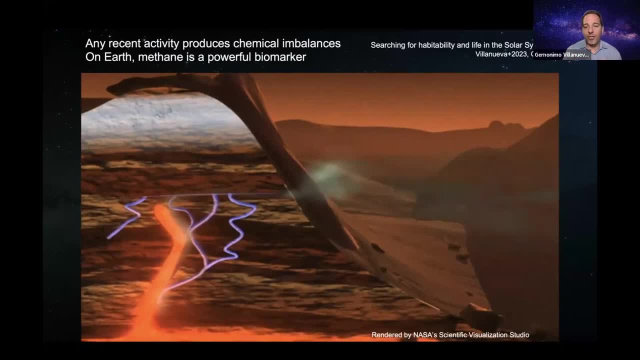 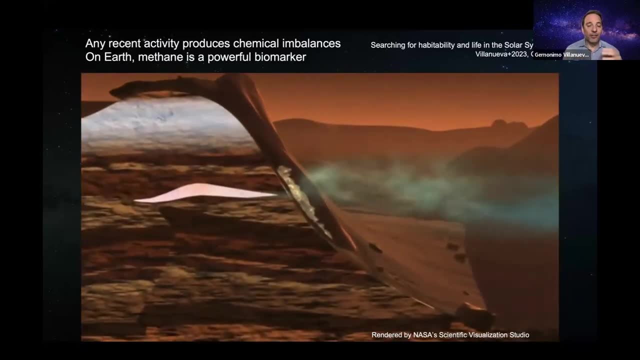 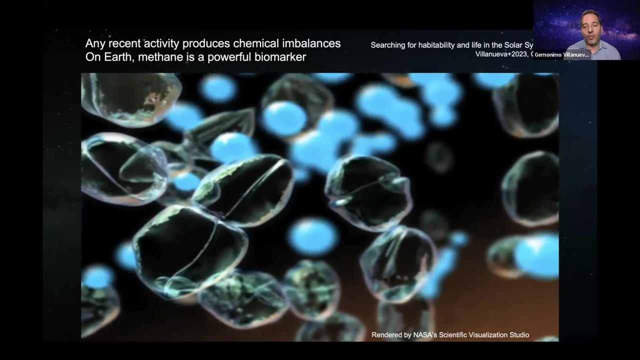 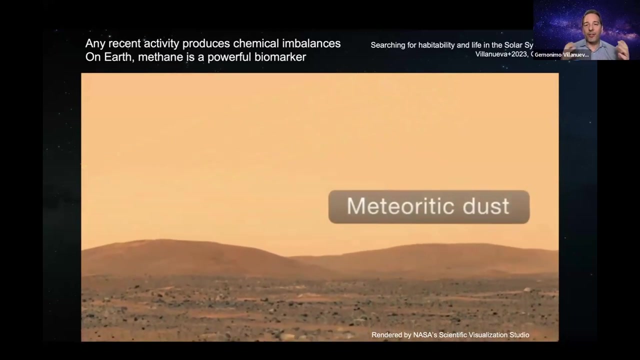 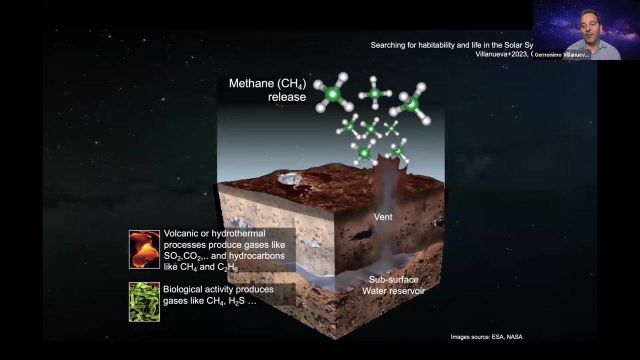 is that we've been able to detect to date- which is over 5,000 years ago- planet. So either of the three things are interesting. That's why we look for them using telescopes. So this is the right hypothesis. You know, this is what we astronomers are looking. 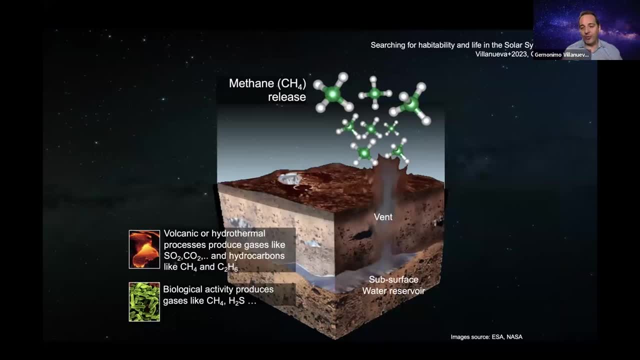 for And we want to see, is that molecule on Mars? And we use all the powerful telescopes, we can think of looking for that molecule. And you're thinking: how do we can look at this molecule from afar? I mean, you may know, some of you may have some knowledge of spectroscopy, but 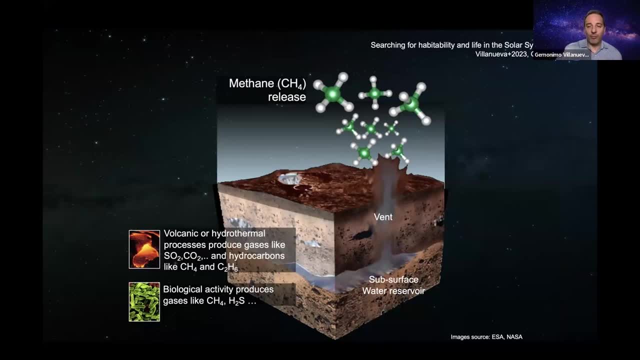 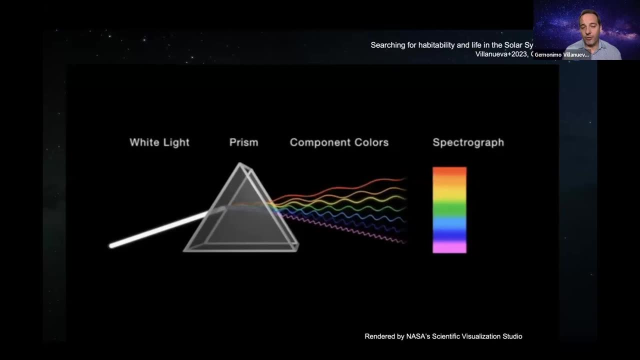 most of the astronomers are actually dealing all the time with spectroscopy, And what the process is is that when you have light- the light, you recognize the colors. you have a prism, a dispersion instrument, a spectrometer, as Stephanie was mentioning- you break the light. 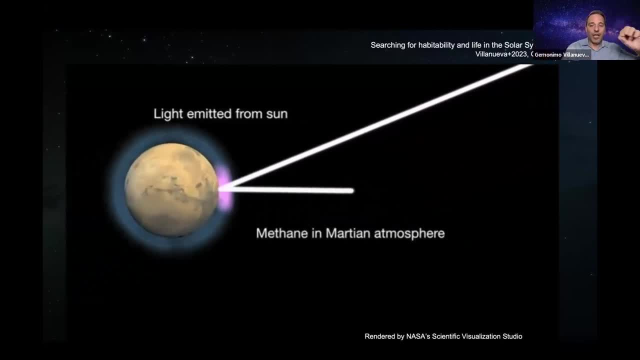 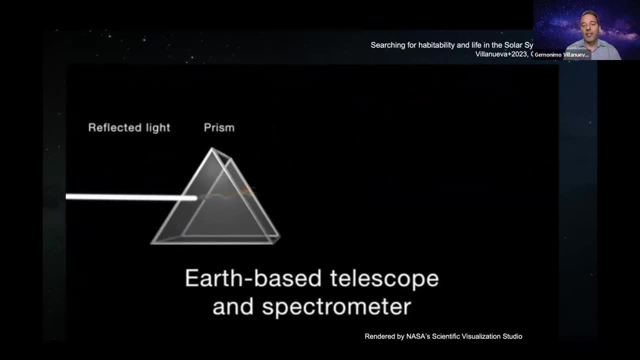 into this color component. So if you have the light of sun shining on Mars, as it goes from Mars gets reflected on the surface. if there's methane gas on the surface and you can look at that light, you will see the classical colors of the sun and then you will see holes on that. 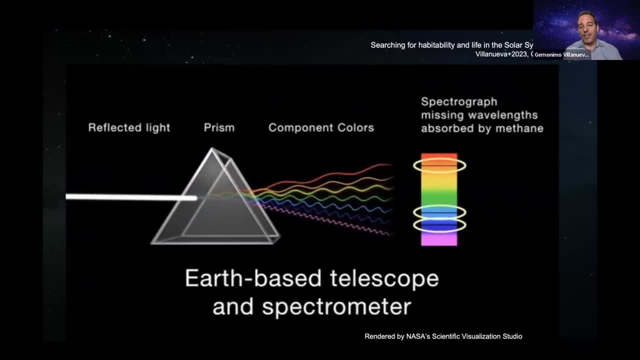 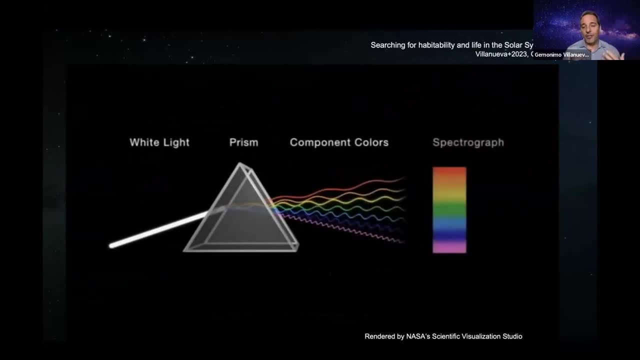 light of the reflected light. Those holes indicate that it's a signature of a gas there. So a lot of our work is on that And we're looking for that And we're looking for that And we're looking for those fingerprints, those very finite, And the better the spectrometer, the better that prism. 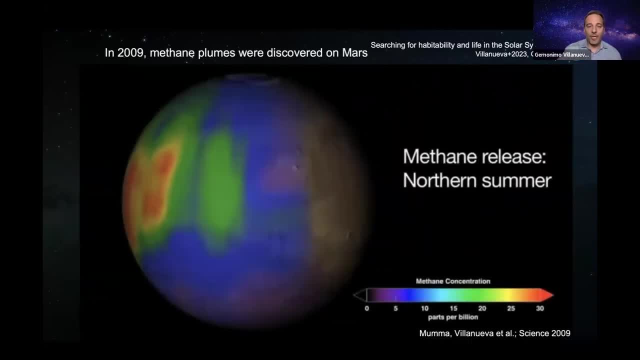 the more precise you can identify those specific signatures. The interesting thing is that in 2009,, using ground-based telescopes, we detected that, And it was a very difficult endeavor. We spent years working on the data, And the challenge is when you measure a gas like methane from a planet. 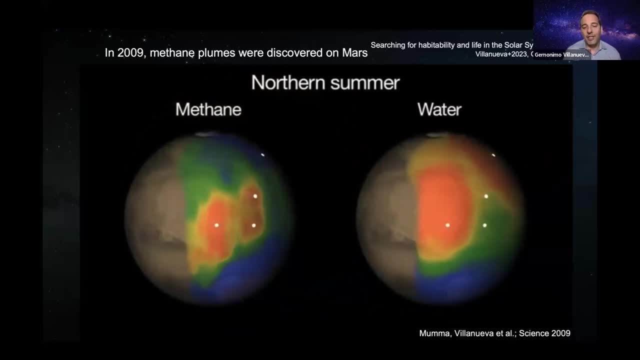 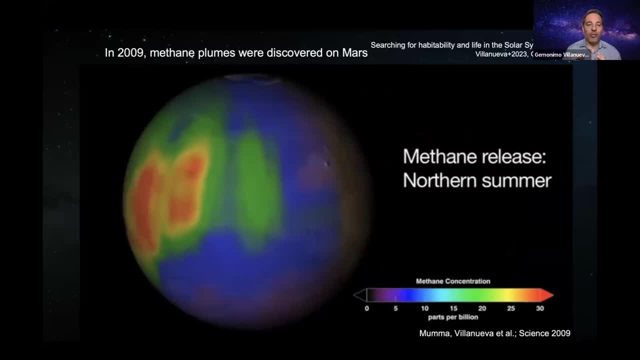 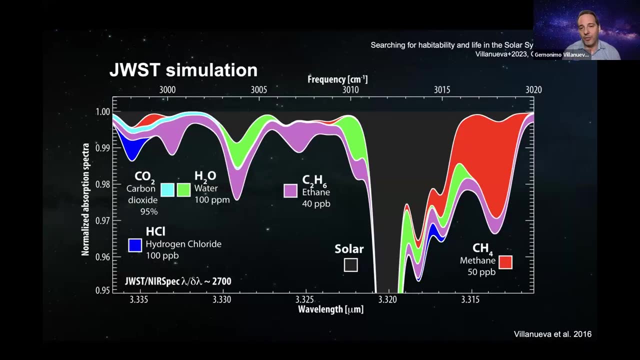 want You can do all your tricks. you want You can do all the things we did, but you're never sure that you remove all the telluric components right. So a lot of the value of having a space telescope. you don't have to worry about that. And this is a simulation we did of how the signature 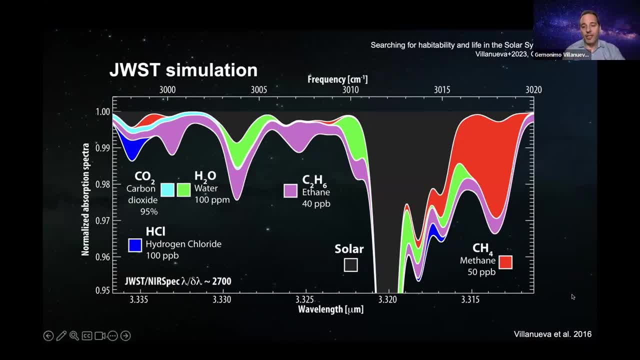 of methane on Mars would look with something like James Webb And you can see, here are colors- We can say the x-axis colors- And you can see you can lose a bleep there And that bleep will be the signature of methane. And this is what we trained the telescope to do. The main idea was: 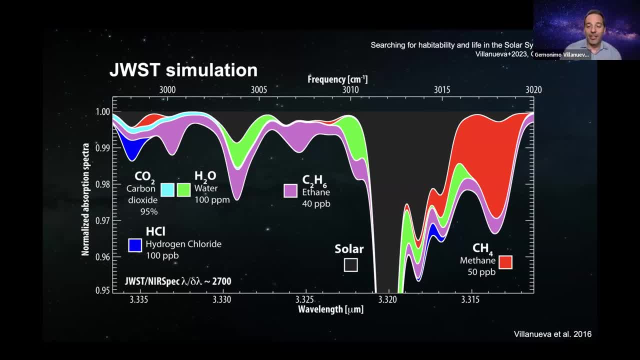 to: OK, can we look at that signature? And we got the data. And we got the data And we got the data in September And of course I kind of mentioned that yet We didn't publish that. But we are looking for that. That is the driver of what our program is about. But this is just to. 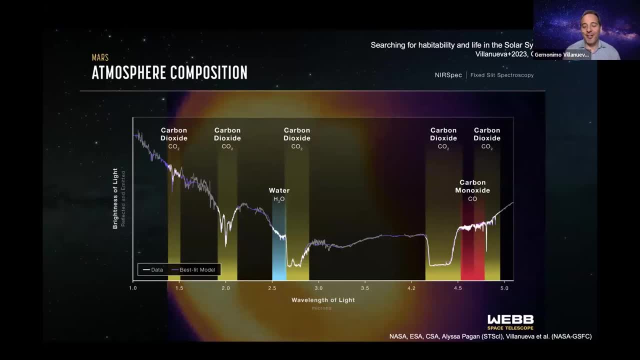 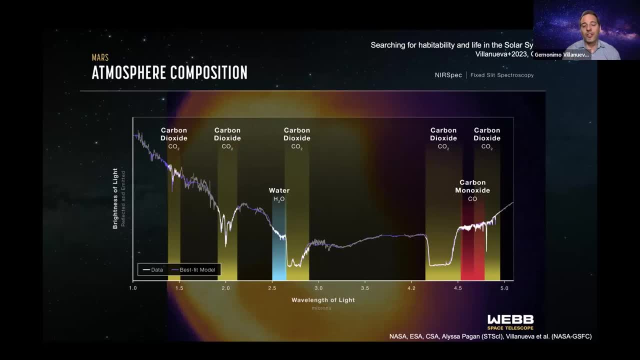 for that And we are looking for that, And we are looking for that, And we are looking for that ats 3.3.. And this is where we are looking for the methane signature. There's nothing obvious here, But you know we are assuming and doing all our значит to make sure. 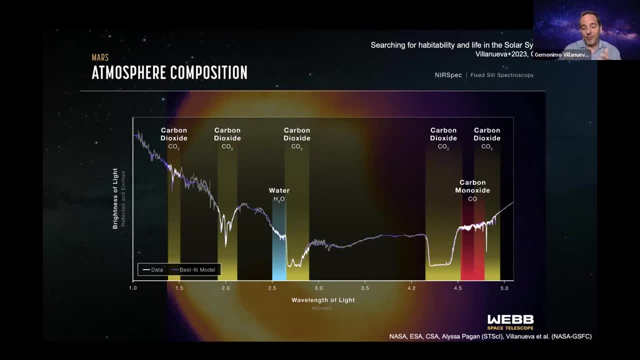 we see it or not, That's the main driver of this work And we hope it's going to be published within a few months. That's a memory work of our thing. But let's go back to the solar system And I think 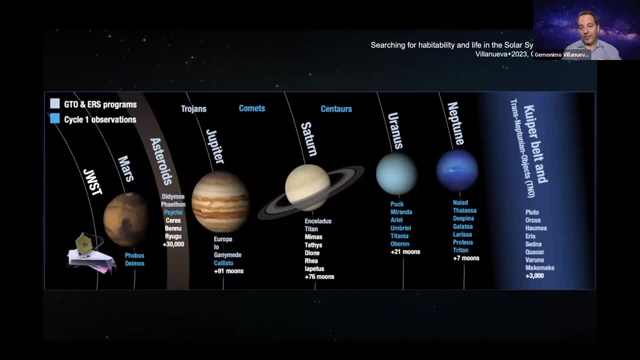 I wanted to focus on the other. If you asked me, when we look forward these things, there are two moons which are super relevant, And that's Titan and—sorry, Titan and Enceladus and Europa. the europa and salas are very interesting because we think there's a subsurface ocean and we think 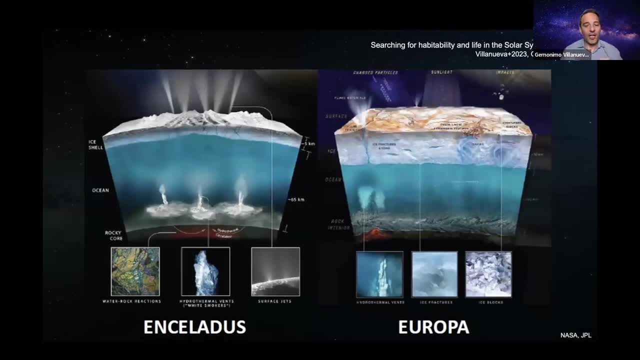 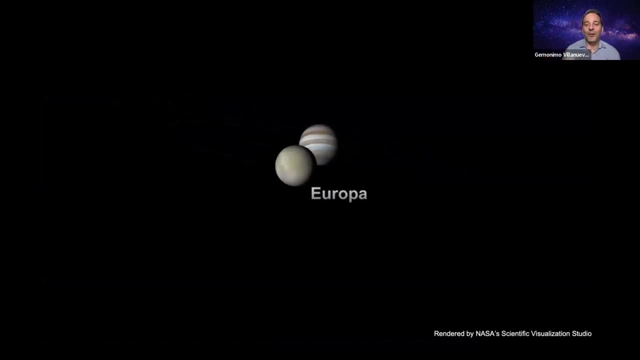 that those are fantastic places for possible life, other thermal bands and stuff, and you can use james webb to study them, you know, and look for signatures below those oceans and you know this is what our running hypothesis. actually, we created this movie with stephanie like in 2016, many years ago, and the 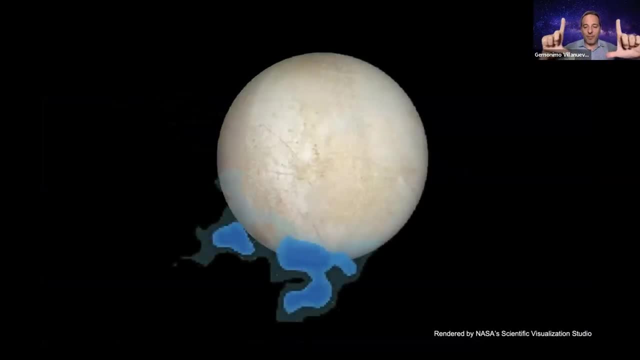 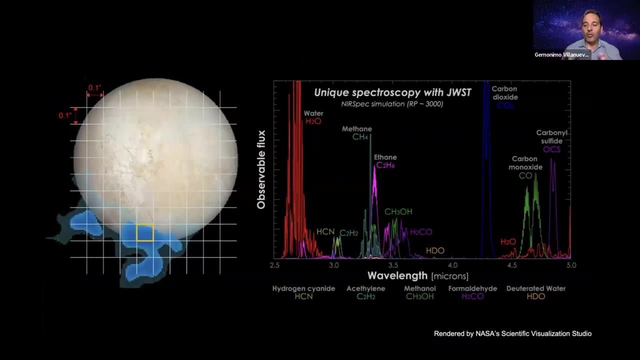 idea is that you point to europa and then you have this special instrument that can, you know, make a little grid and we can get, for every of those pixels, a full spectrum. we can get all the colors and then the same signatures. we're talking about the building blocks of life and the figures we're 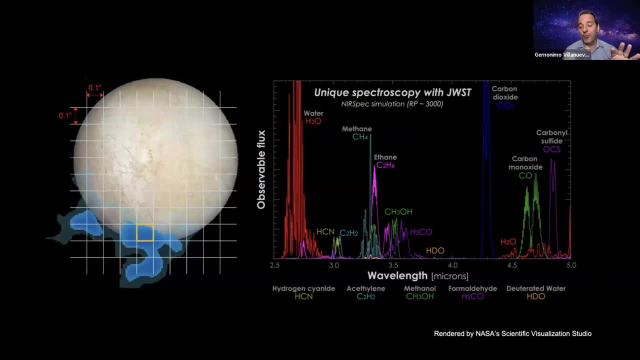 talking about, you know, habitability and things like that. we can search on that room so and also we can study the surface. so that is the main driver with. again, paper is gonna be soon published. we actually work with people from seti on this, so exciting data sets and it will probably, we hope. 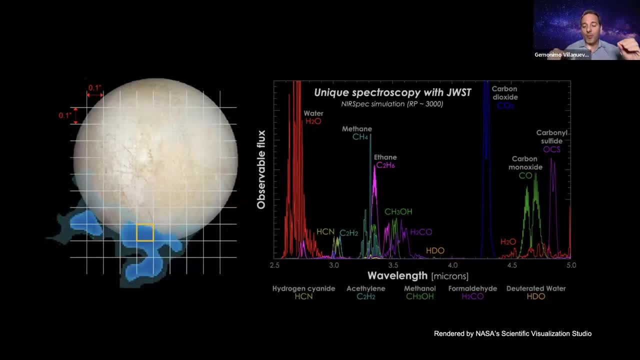 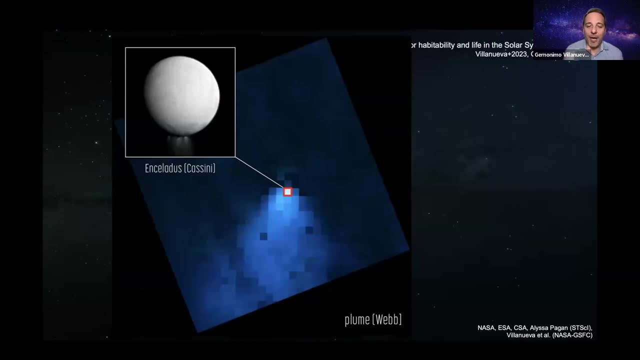 within one, a few weeks, we're gonna get the results out. but again, just web. this is the simulation. we will see what we get with with james webb. but luckily, yesterday actually we published the installed results and those are fascinating. you know, we we did the same thing i was showing you for for europa. we point in there. 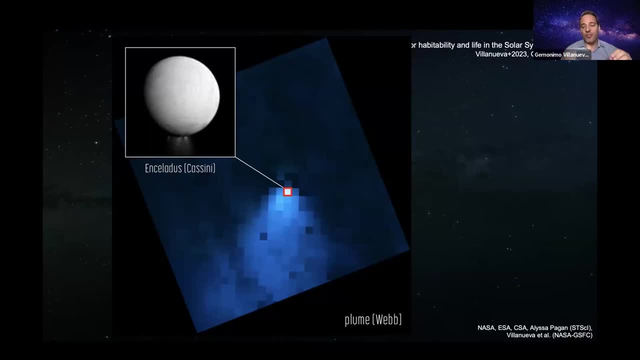 we hoping to see something, but we did not suspect, and just to give you a sense of what we saw, which is super remarkable, this is the size of the moon, this is the, the small moon, and this is what the images we had before you can see, there's a little bit of a, a plume, therekon Mago. 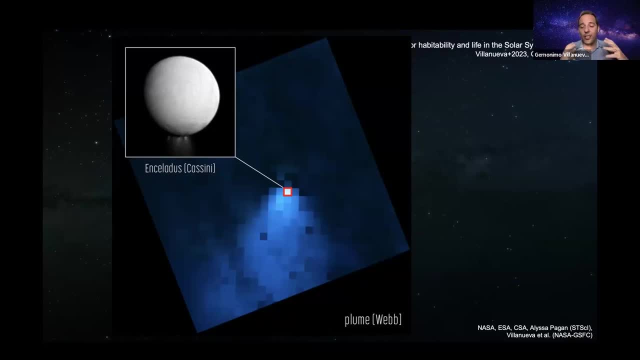 there There were some measurements. flying Cassini managed to fly around and take all these beautiful images, But now with GENsWeb we can actually do a zoom out and we can actually see the mass extension of that plume And we can actually measure the composition of that plume. 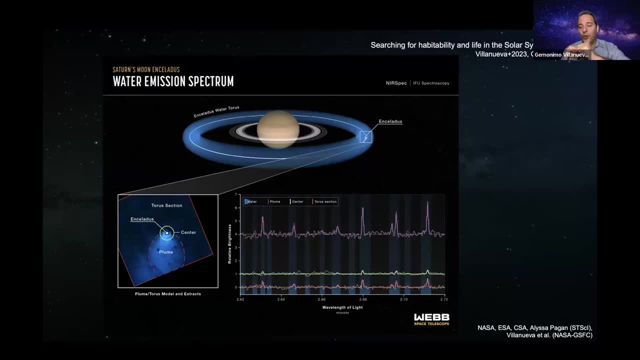 I mean not only that we can actually see the plume, but we can also see the torus of water that, as the moon flies around Saturn, it leaves a cloud of water, and we can measure that with GENsWeb and we can go all these spectral signatures there, Just to show you what is. 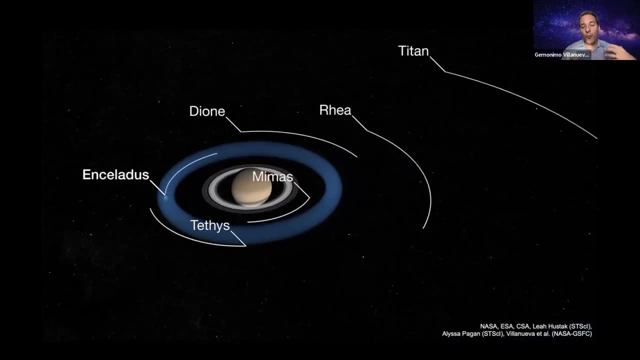 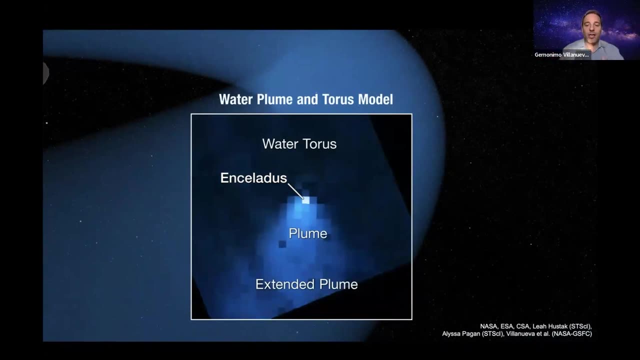 the geometry of what we did, So you can see all the moons going around, What we saw. we saw the torus of water. It was fascinating. But we also see this conical plume of water. We can actually model that plume of water very nicely And then we can see that massive release of water And 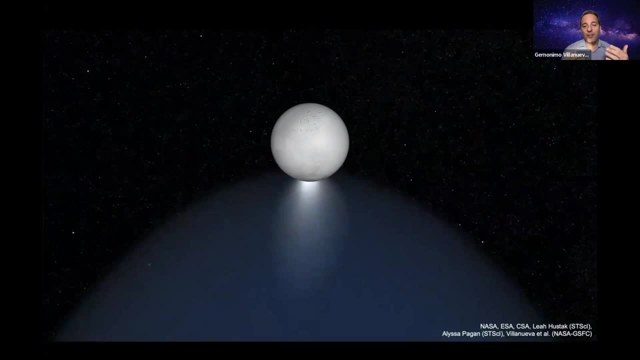 interestingly, that release of water. tell us about that. there is maybe a way to connect to the subsurface ocean, and it's been going on. So that is the main things that we're coming out with, And then we're going to go to the next slide. So that is the main things that we're coming. out with And then we're going to go to the next slide. So that is the main things that we're coming out with And then we're going to go to the next slide. So that is the main things that we have And, of course, you know we we're now going to go for the questions. we're going to 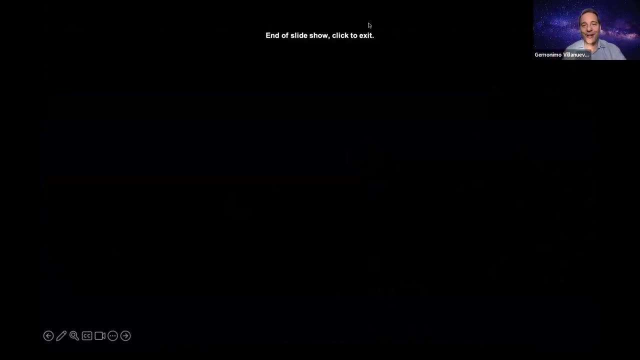 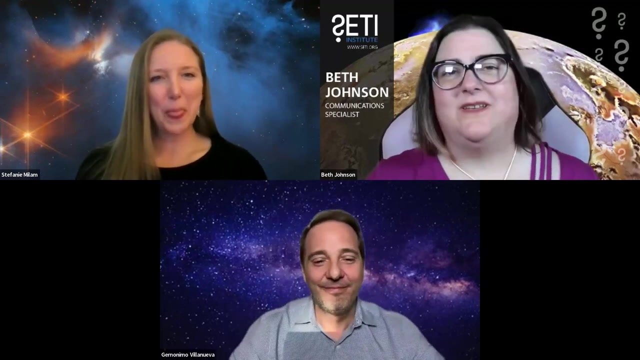 go on and see what you know what, how we interpret this result are we getting now? Thank you so much. I'm very excited by the new work that has come out from both of you, So we're going to talk about that Definitely. 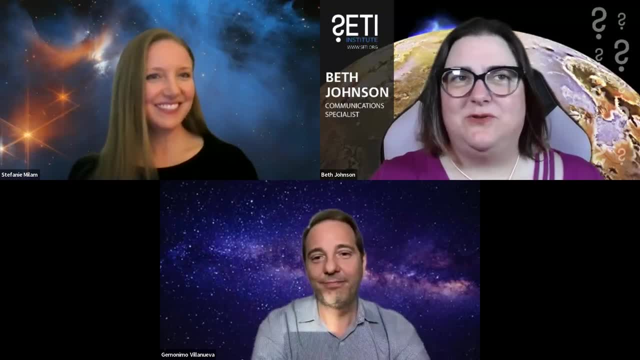 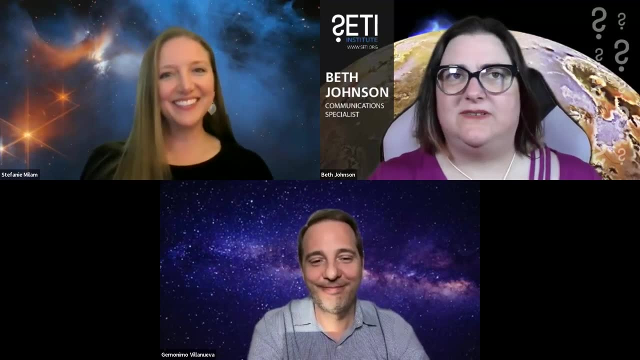 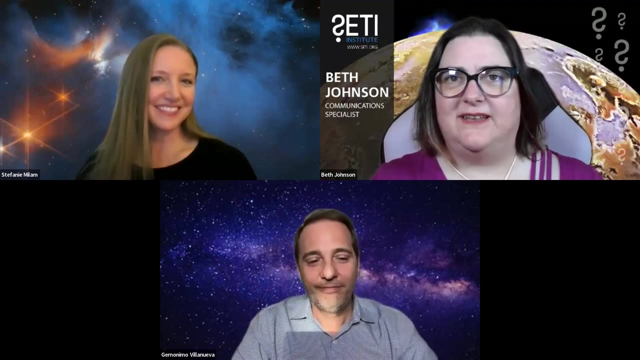 But first I kind of want to, I kind of want our audience to get to know you guys a little bit. So tell us about how you both became scientists. What got you into science? What got you into this particular type of science, Geronimo, go ahead and start and just kind of tell us your. 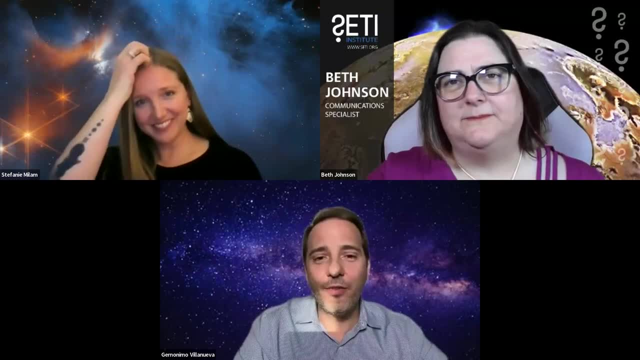 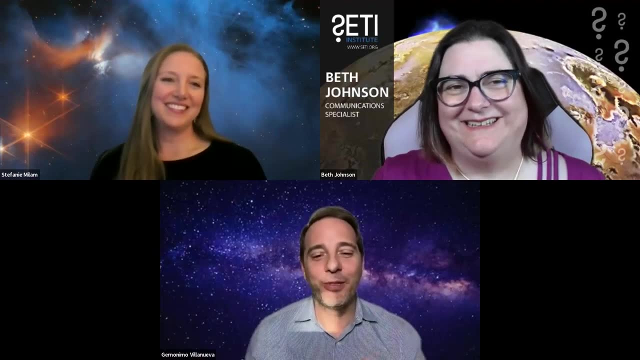 story. Yeah, so well. I am originally from Argentina. I was when I, you know, for me NASA was impossible. I mean so far away, it's unachievable. I was good with computers, so I. 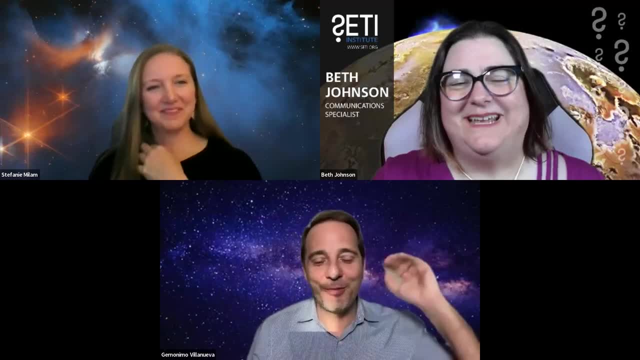 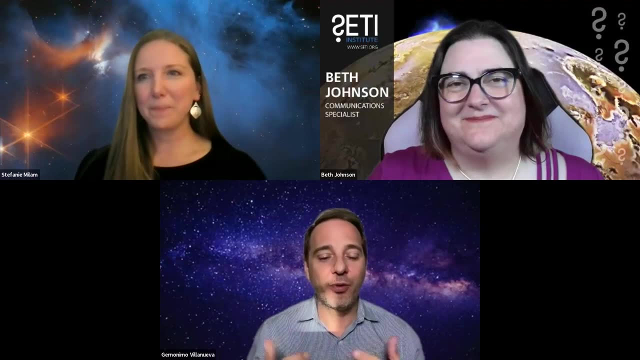 was like computers. I was hoping to become the Bill Gates of Argentina. That was my big motivation. so, and then I was lucky that I was studying engineering and I got lucky that I had good professors to, you know, direct me into research and I did a. you know, we started the Ocean Hole. 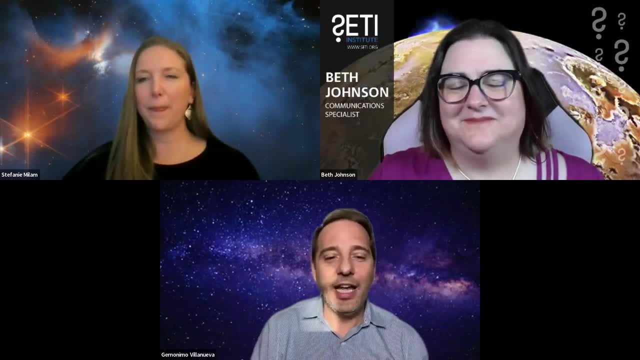 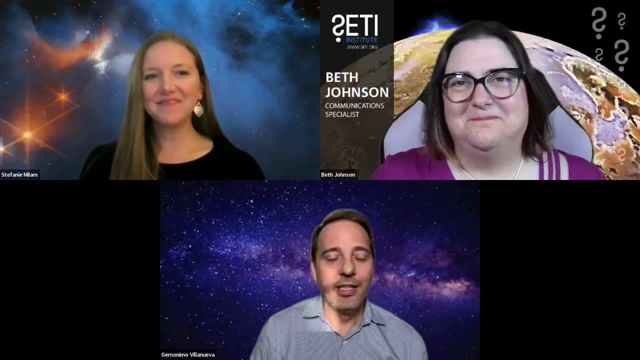 in Argentina. We are in the border of the Ocean Hole over there and we embarked on that. and then I went to Germany to do the same thing, for the start the northern thing, and then I, when I went to Germany, obviously it went to a good research place. I really opened a lot of doors and that 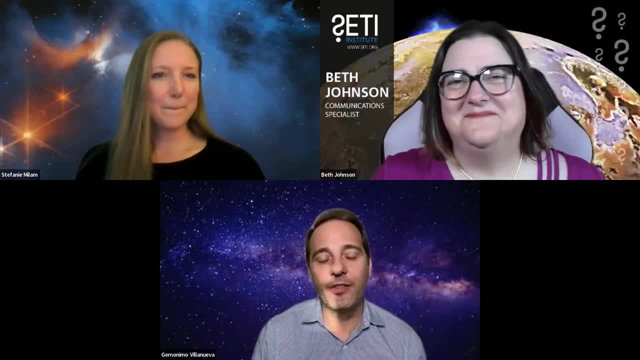 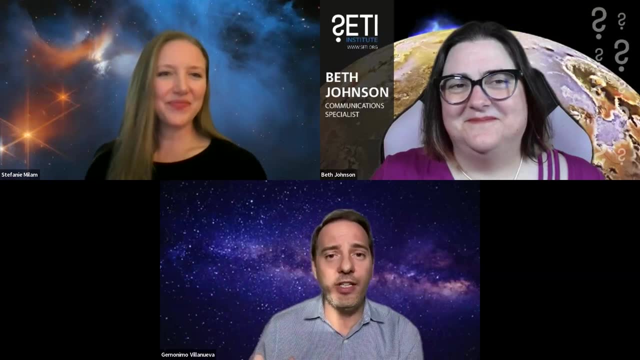 really opened my mind Professionally personally. it was an amazing experience. and then from there, of course, I went deeper into research and allowed me to open many doors. and then I connected with NASA, at the time working on SOFIA, and then from there I came to the US at NASA Goddard, and I've been 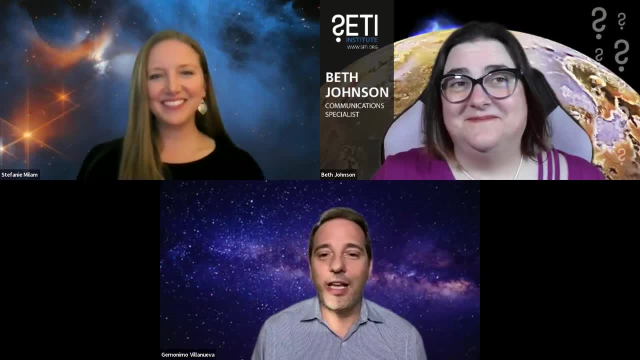 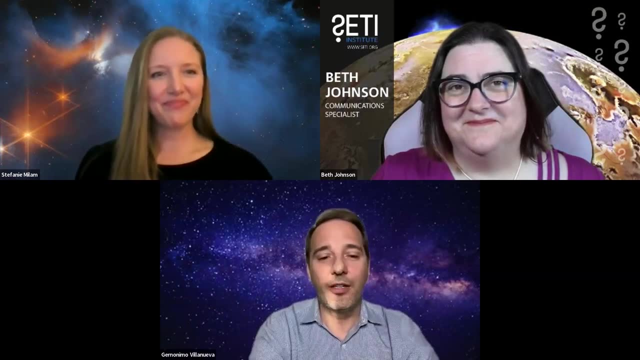 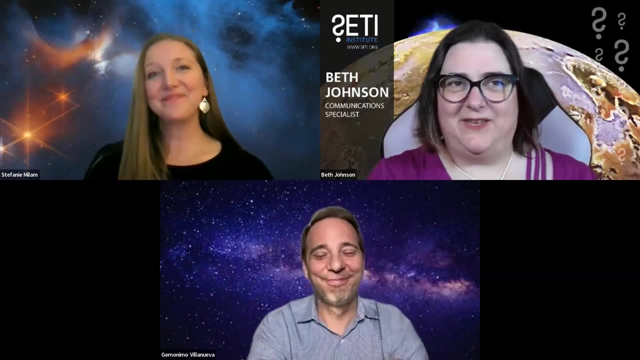 there for 18 years, so Goddard really allowed me to explore these things. You know, we can involve in missions like ExoMars, We can involve in James Webb, so it's really a privilege to be working in a place like Goddard. yeah, Stephanie, you know Geronimo from before tonight. This is not a high. 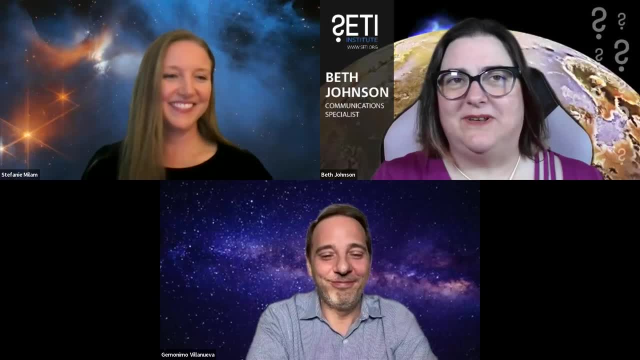 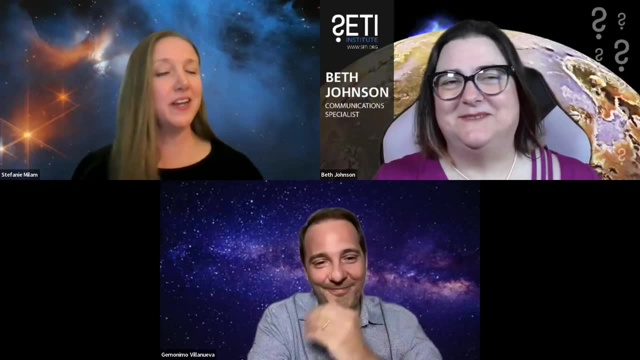 you've met for the first time, so tell us about your own career Path and how you ended up working with Geronimo on some of on some things earlier. So my story is is very different. Actually, anybody, anybody you talk to at that's- that's a. 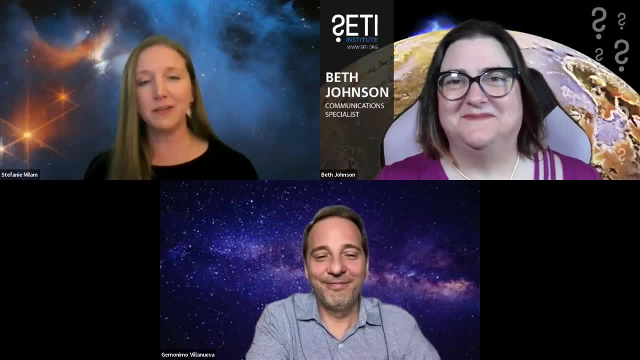 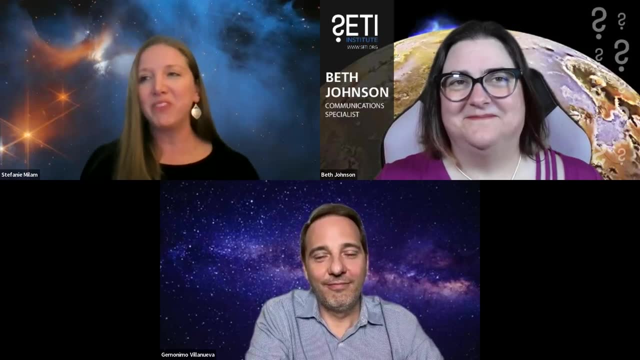 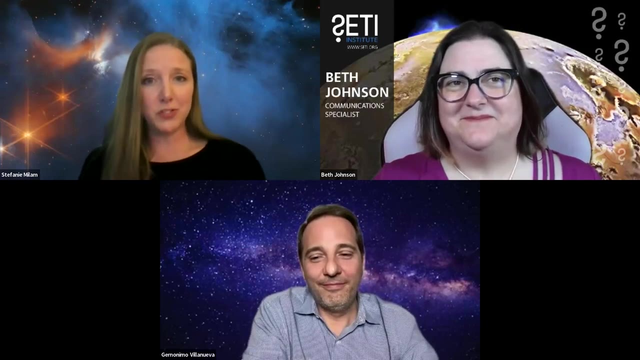 NASA scientist. they will have a completely different story with how they became involved with working at at any NASA center or how what their story is. So I love hearing everyone's stories and it's really quite a journey. So I I grew up in Texas. I grew up in Houston. 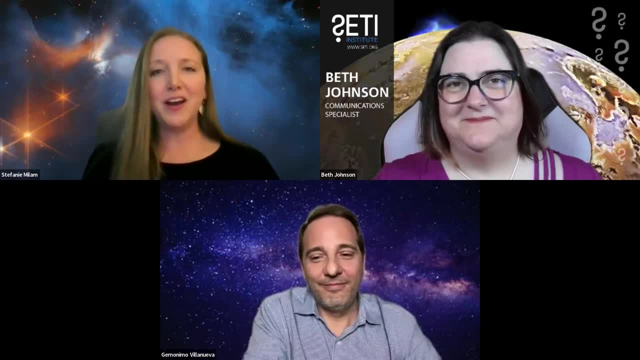 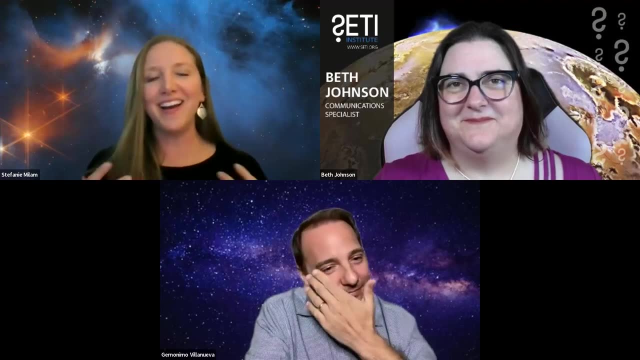 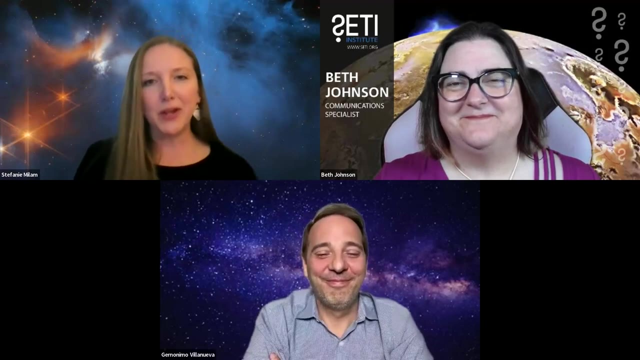 Texas. I was born and raised here in the state of Texas And when I was very young- I was about six years old- I had a summer field trip down to Johnson Space Center And I came home just wide-eyed and excited and I told my mom I was going to work for NASA one day and be an astronaut, or I was. 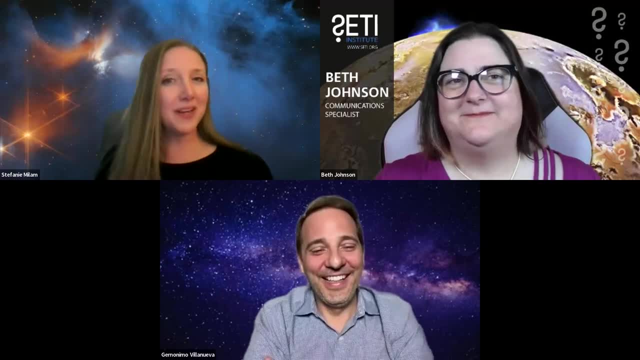 going to be a ballerina And the dancing's carried through. it got me actually through college. I even had a dance scholarship, But I decided that I wasn't going to be a dancer for that long because I was already kind of, you know, a few years old, But I was going to wear my 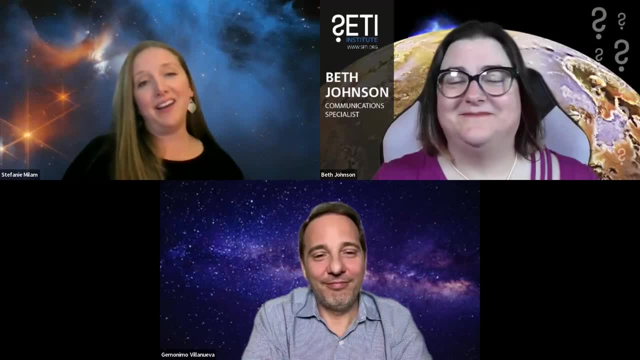 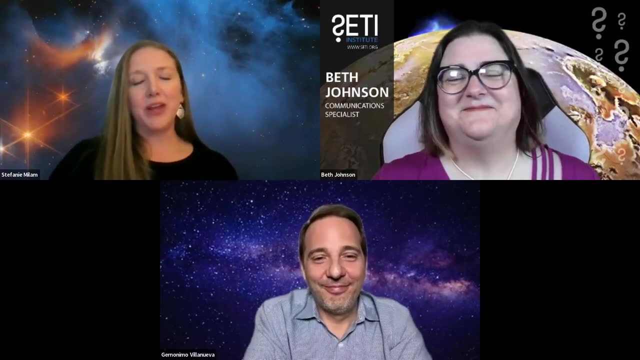 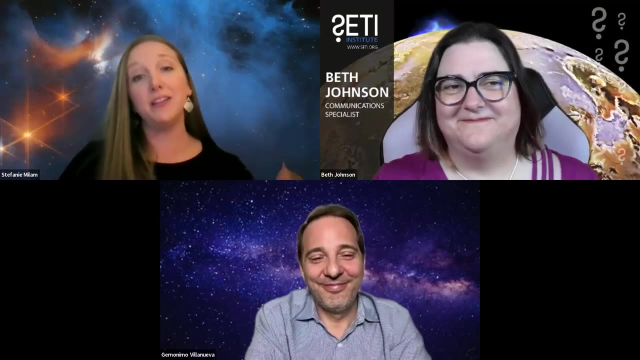 a dance scholarship But I decided that I wasn't going to be a professional ballerina, I was going to become a scientist. And I never got another growth spurt to quite meet the- you know, you must be this tall to ride this ride- requirement to be a pilot for the space shuttle which now 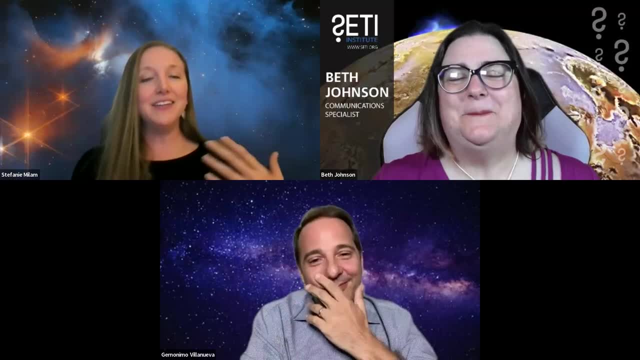 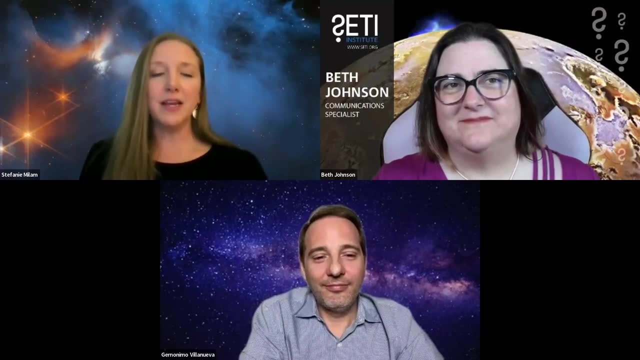 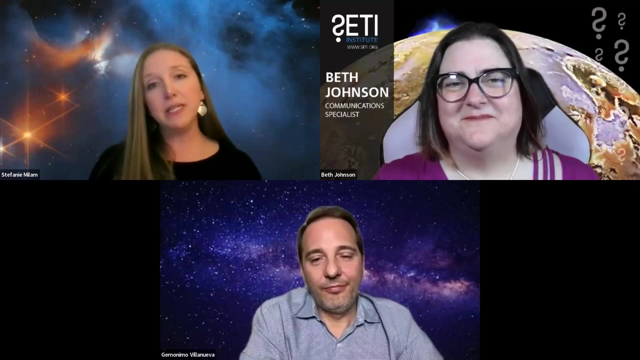 I'm dating myself, But I knew the only other way to become an astronaut was to be a mission specialist, And that meant I needed to become a scientist, And I was very good at chemistry And I also thought it was an applicable skill for an astronaut working on the space station. 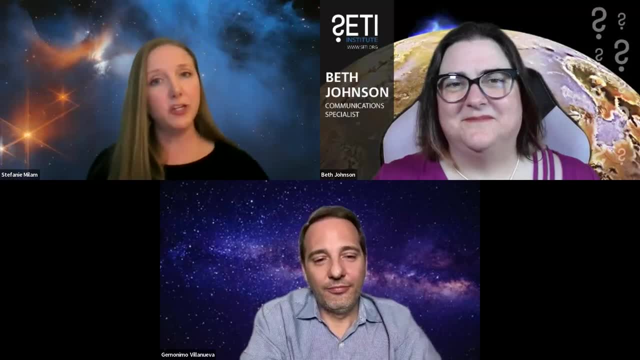 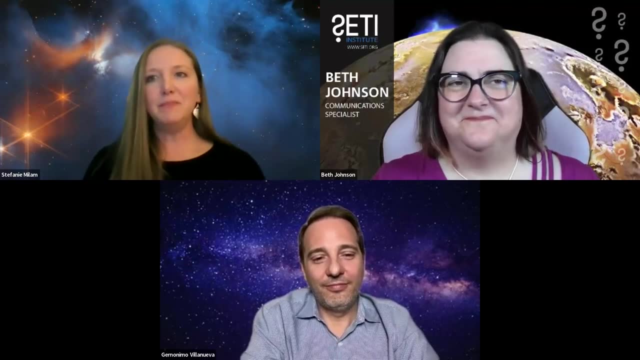 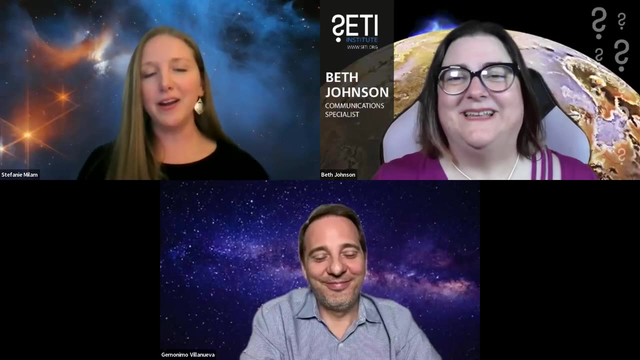 or if I would ever go to another destination, having the skill set to, you know, be able to run experiments and troubleshoot things in real time. And so I pursued chemistry, And after a number of years in college of washing glassware in an environmental lab, I was able to do a 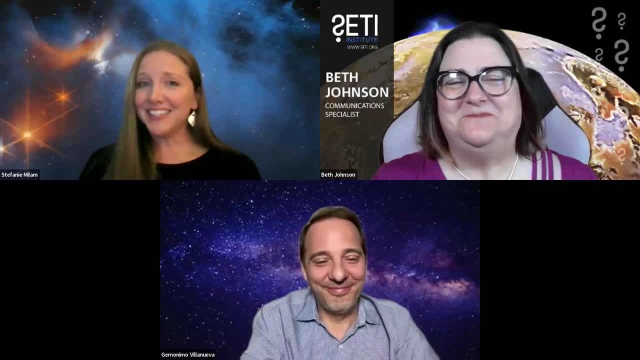 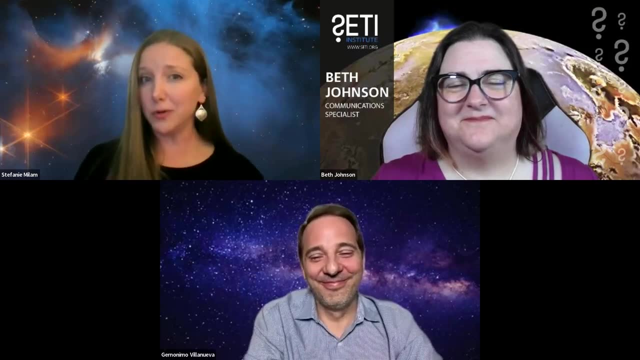 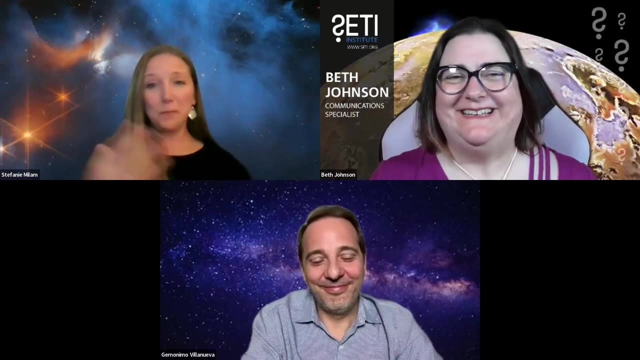 laboratory And also as an assistant winemaker, I decided that I didn't want to do any more dishwashing ever again. I've actually vowed to never own a house now without a dishwasher- an automatic dishwasher or a significant other. that's the dishwasher, And she told me to pursue. 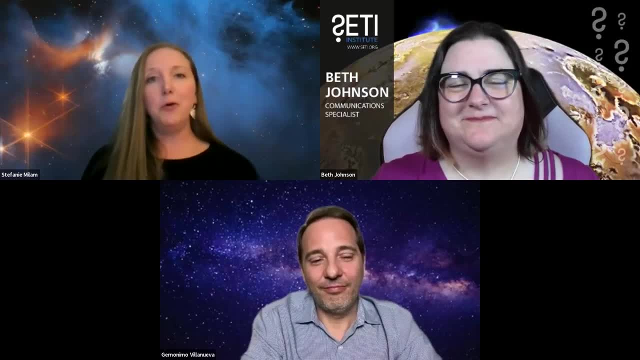 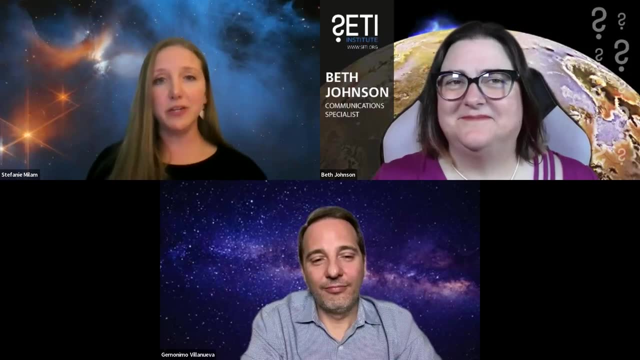 astrochemistry, And so then my whole career grew from, you know, working in a room washing glassware, to now using telescopes and studying chemistry across the world, And so I was able to do a number of different things, And I was able to do a number of different things, And so I was 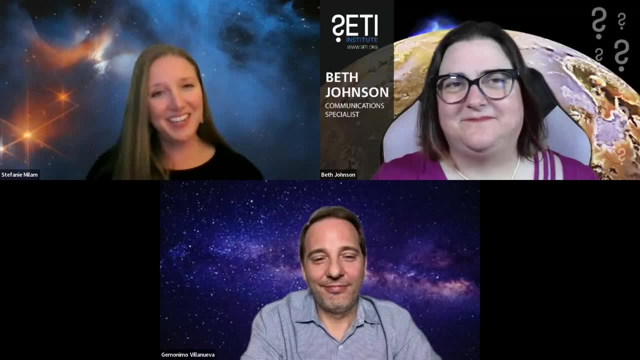 able to do a number of different things. And I was able to do a number of different things And I also learned how to run some experiments across the entire universe. That led me coming to study and NASA Ames, where I did my postdoc, and learn how to run some experiments that were relevant to 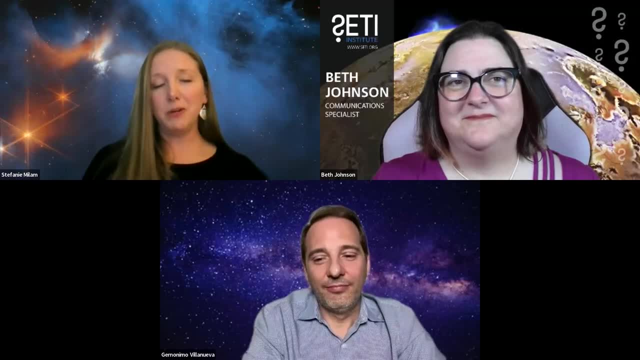 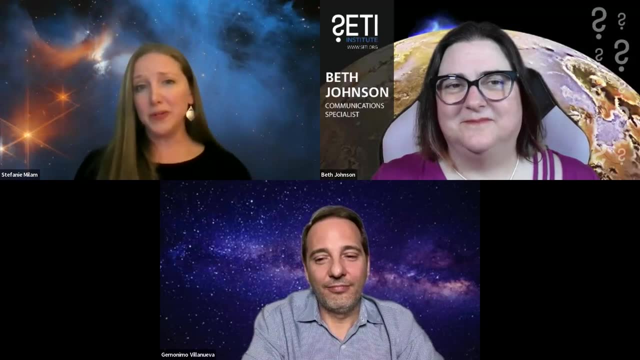 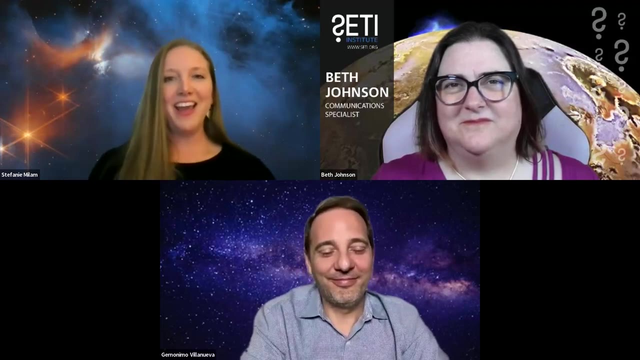 the observation, the observations that I was doing in grad school And that led me to becoming a scientist at Goddard Space Flight Center and working with Geronimo. I actually met him, though, when I was a graduate student working in radio astronomy, And my 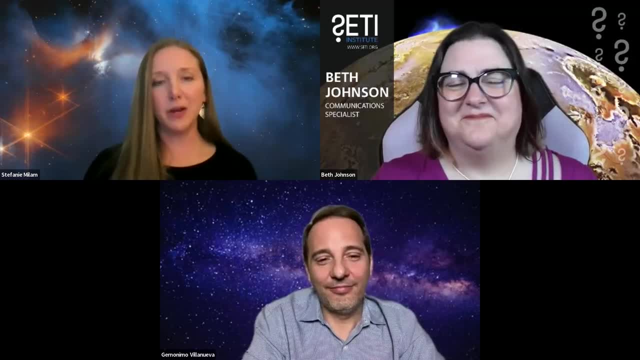 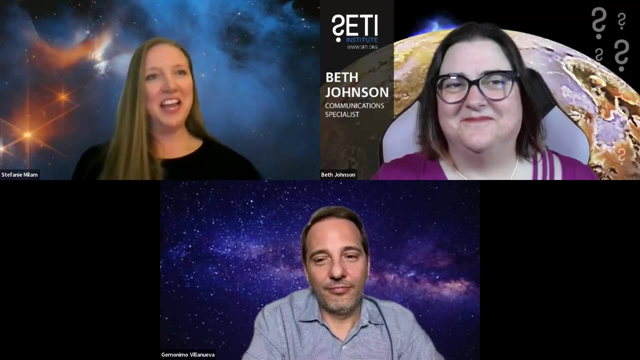 supervisor when I was a graduate student was the director of a couple of radio telescopes in Arizona, one of which we were testing some instrumentation on that Geronimo happened to be working on during his thesis And he had an interest in planetary science And so when he was coming to visit 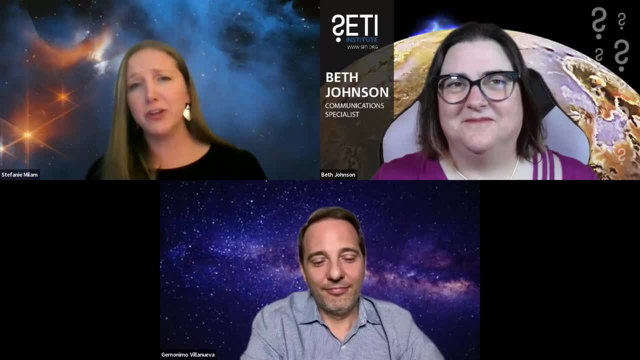 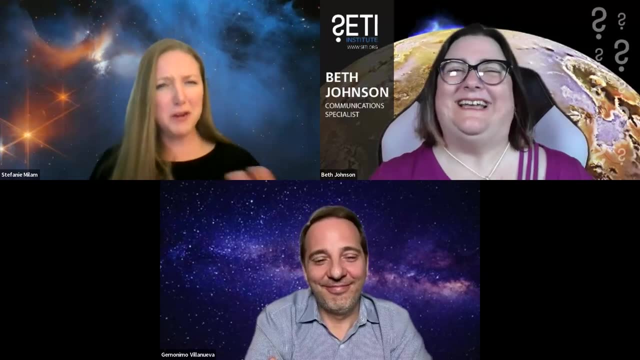 I was told to host him and take him to the telescope and make sure that everything worked. And I was really kind of upset about it because I was a graduate student and I had my own work to do. I don't want to be shuffling around visiting scientists, you know. 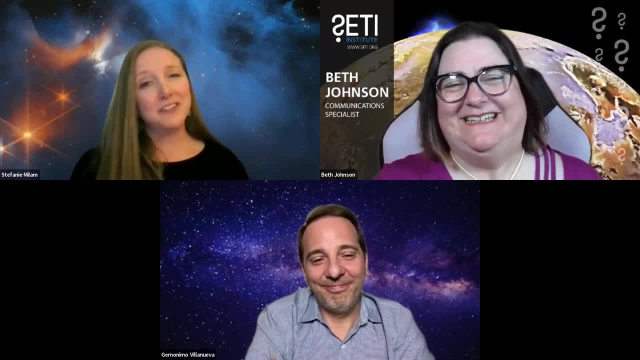 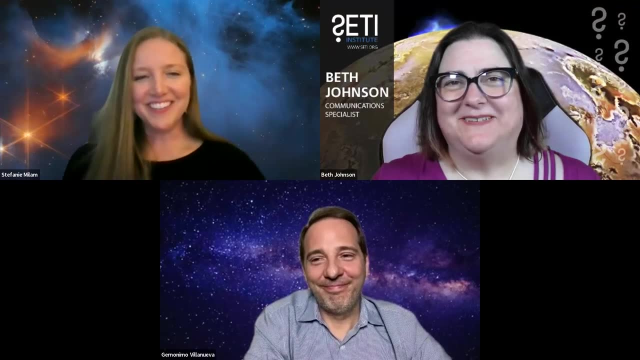 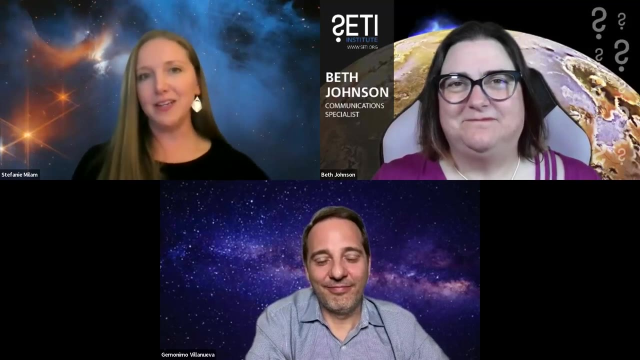 we had staff for that. But we actually started collaborating all the way back then in grad school. So we've worked together, dare I say, almost 20 years now. So it's been a very long time. And when I came to Goddard and got to, you know, rekindle that collaboration and then the science. 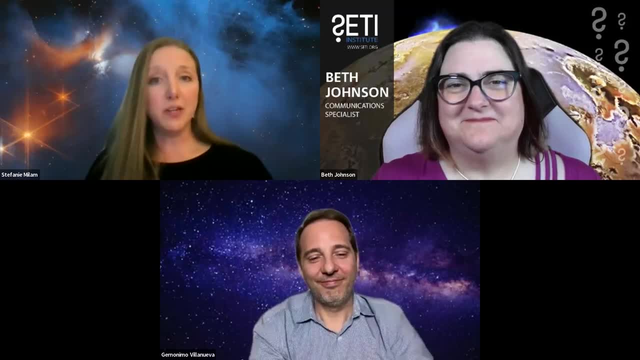 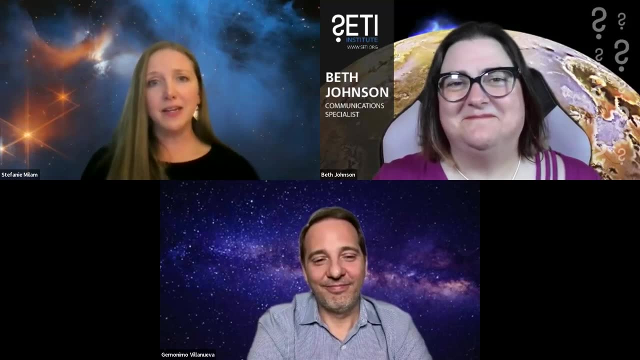 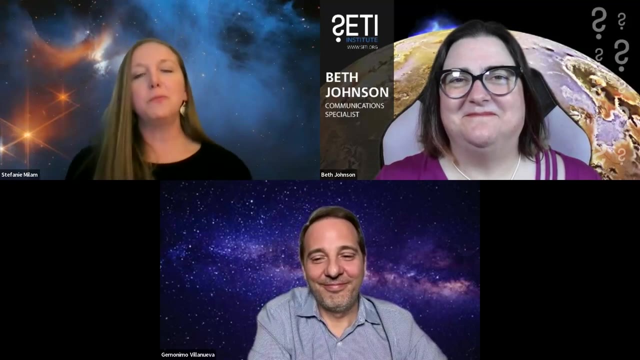 it was absolutely fantastic And when I started working on the James Webb Space Telescope, Geronimo was absolutely essential in supporting the science cases that I needed, because I don't study Mars, I study comets- And he really helped make sure that the telescope. 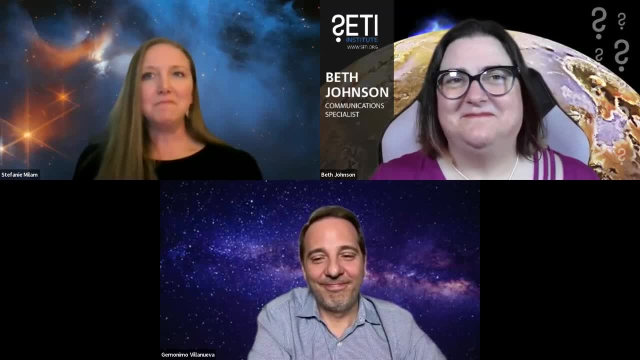 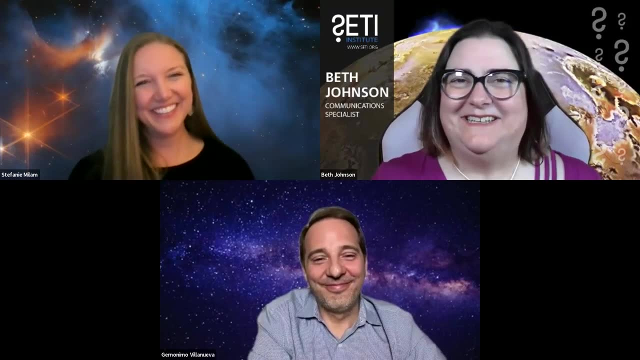 was doing the things that we'd hoped it would do and basically made my job a lot easier, And I didn't have to figure out how to study Mars. So, Geronimo, do you have a side of that story that you'd like to share with us? 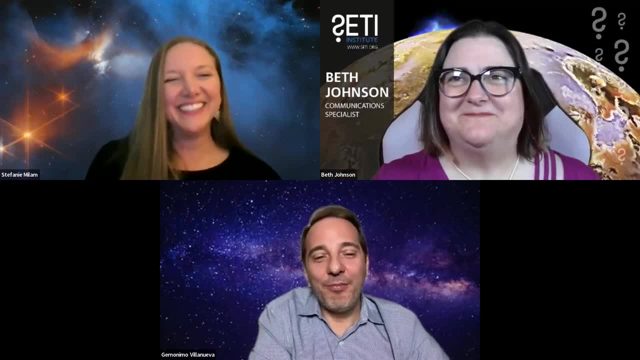 Well, I mean it was, I mean she was definitely a client. but I have to say I remember when I came, so I came from Germany, I was, I think, one of my, you know, one of my first. 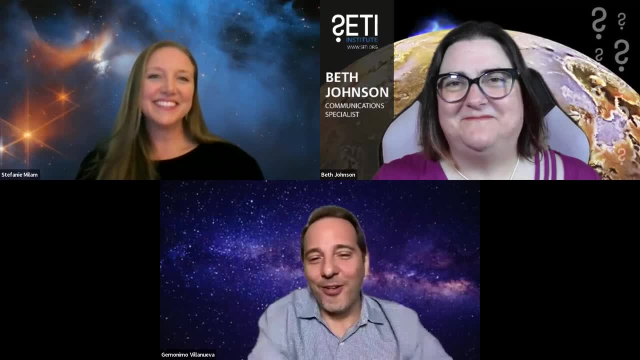 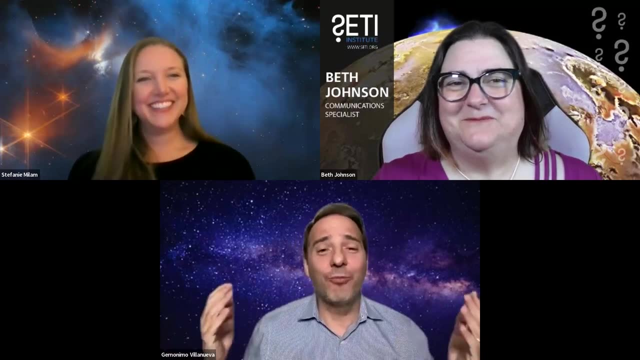 trips to the US. I was excited, you know, go to Arizona. you know all excited about going there with my little instrument. And I arrived there And then I said, Oh, you know, there's another comment. I saw, oh again, wow, fascinating find of someone who does comets. And then I snuck to. 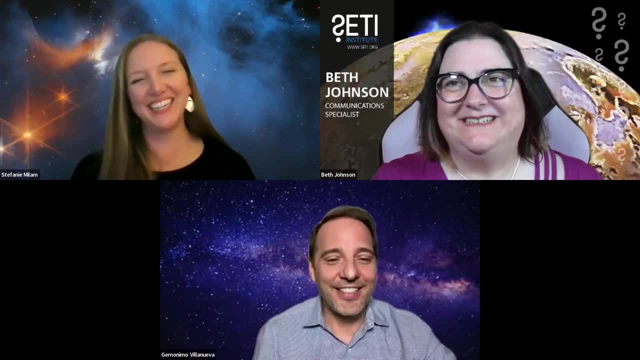 her office and she's like: what do you want? It's like: okay, this is not going to be very friendly. I mean, I think America is not very friendly. So yeah, that was, that was that way, But yeah. 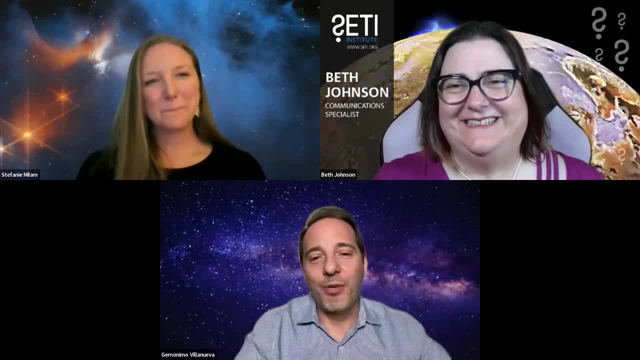 then we work together because we have a lot of work to do. So, yeah, that was that way, But yeah, then we work together because we have a lot of work to do of overlapping projects, So it's really great. This is probably just what has been fascinating. 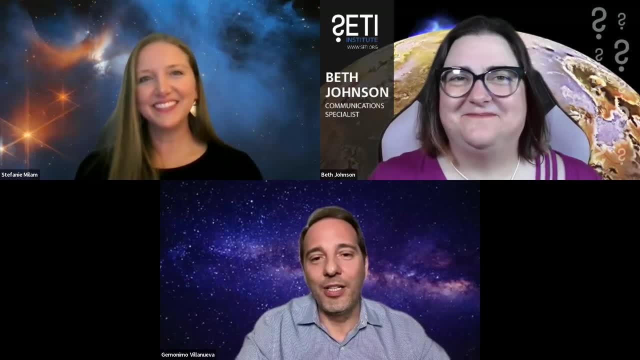 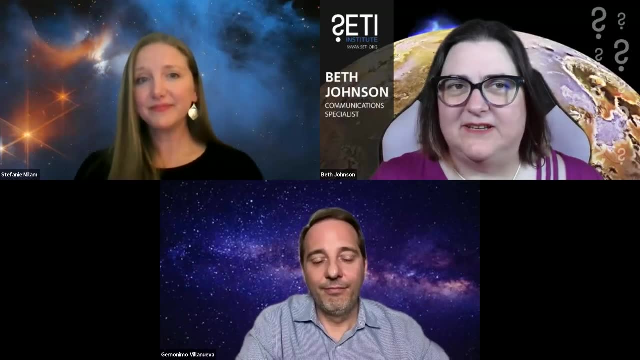 for the both of us. this telescope is, you know, really opening a new area for astronomy. So why? how did you guys become involved in JWST? You both end up at NASA Goddard. now you're both working on JWST research. I know that that's sort of a an overarching question for a lot of people. 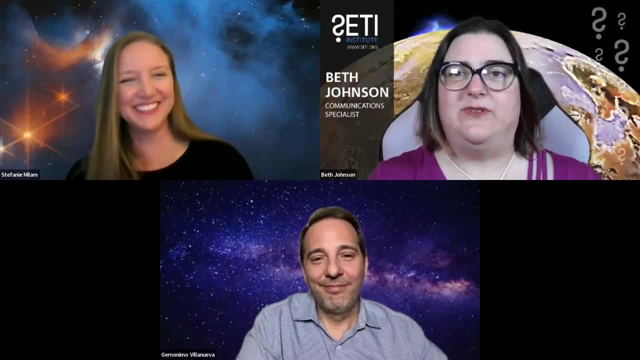 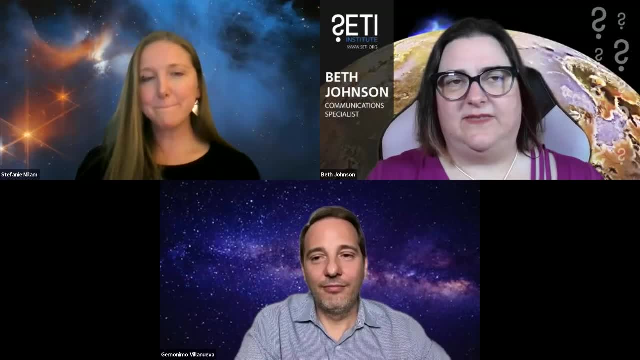 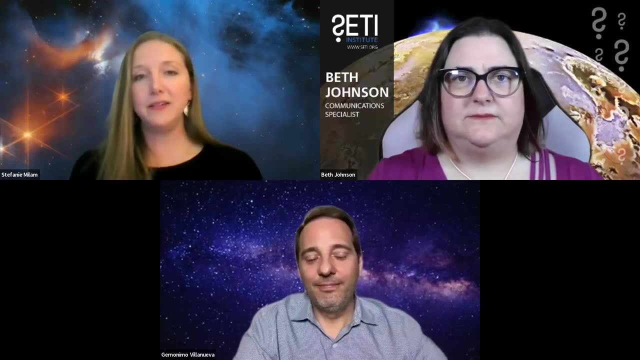 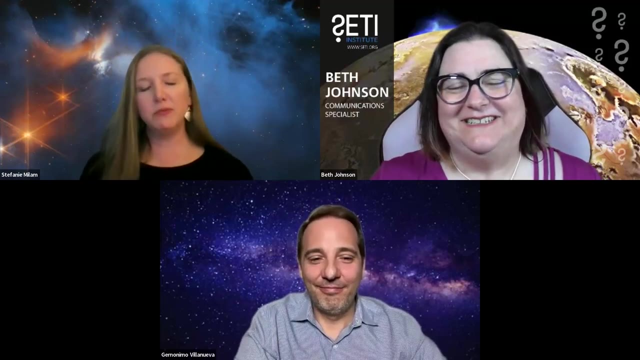 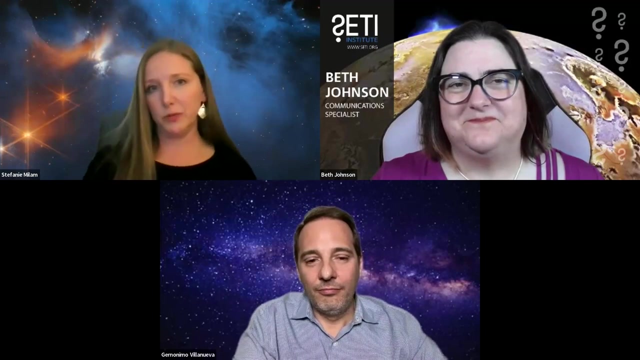 Because of JWST. Because of JWST. But how did you guys end up in this particular research, working on this space telescope? So I actually drug Geronimo into it. So I'll start. When the James Webb Space Telescope had its big replan in 2011,- 2012,, the project science team was sort of taking an interim. 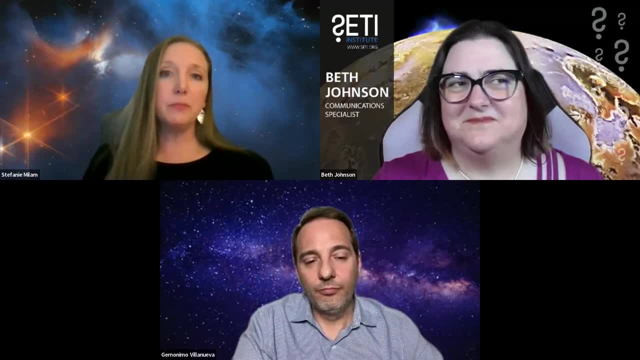 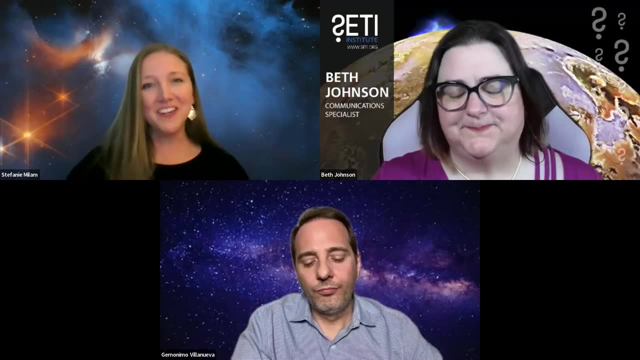 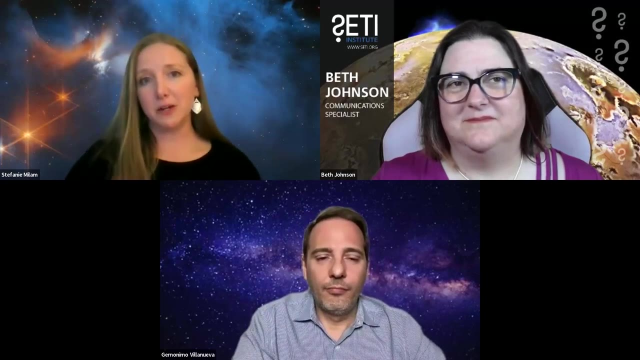 self reflective look of. you know all the things that we're promising the entire world that this telescope is going to do now, with a lot more scrutiny and a lot more pressure, to stay on budget, to stay on schedule. And they realized that there wasn't a planetary scientist on board. 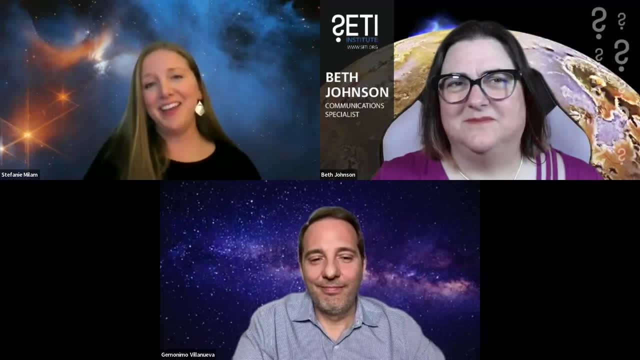 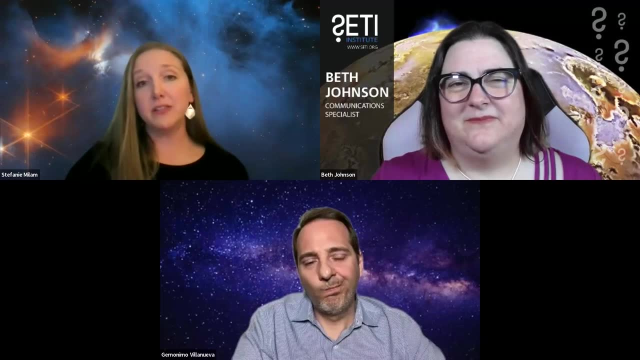 Solar System science is far more challenging than almost any other component operationally for the Space Telescope, Mostly because objects in the space telescope are not going to be able to move in the same way that they move in the solar system. They move with respect to the background. 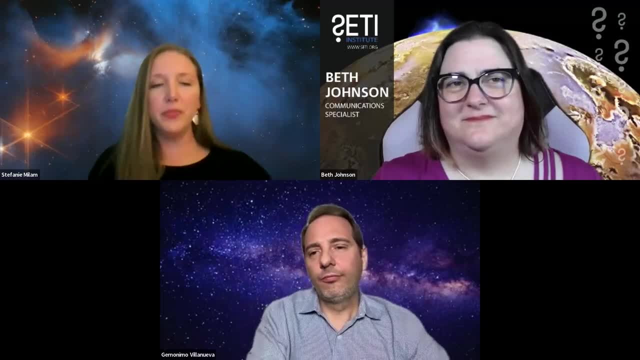 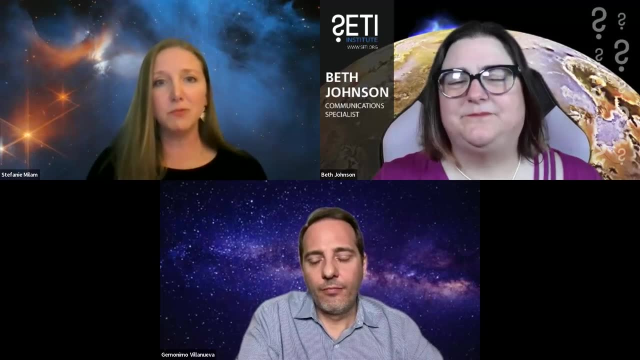 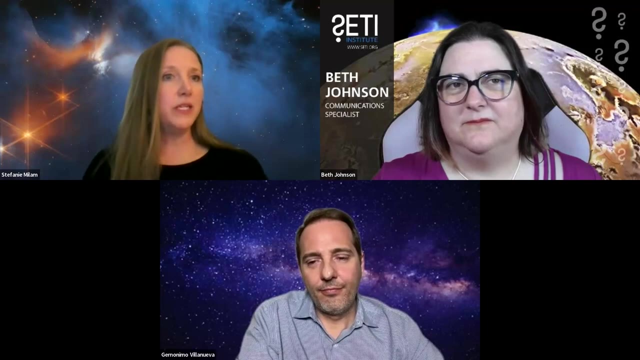 stars, So we have to know the exact position and when they're moving and what time and how fast. We also have the brightest objects in the infrared sky that the James Webb Space Telescope will be ever observing, including Mars, And that is very, very challenging And we didn't, we weren't able. 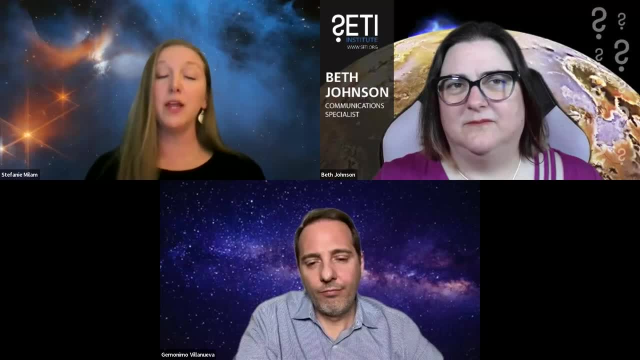 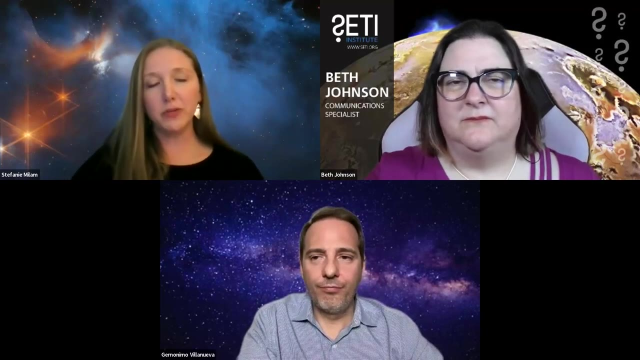 at that point to go in and modify instrumentation to enable new science, And so one of my roles was- or actually, whoever this person was going to be- their role was to make sure one we could track targets that were moving in the solar system, but also to ensure that we had capabilities and 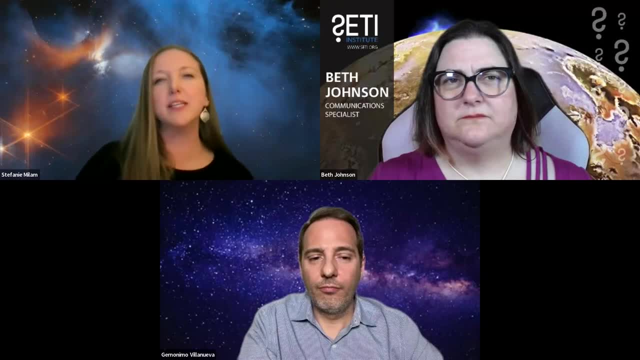 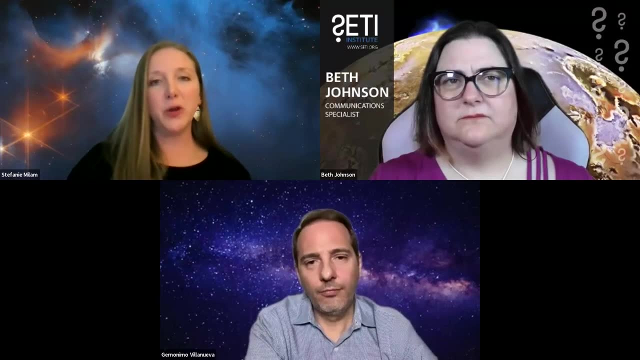 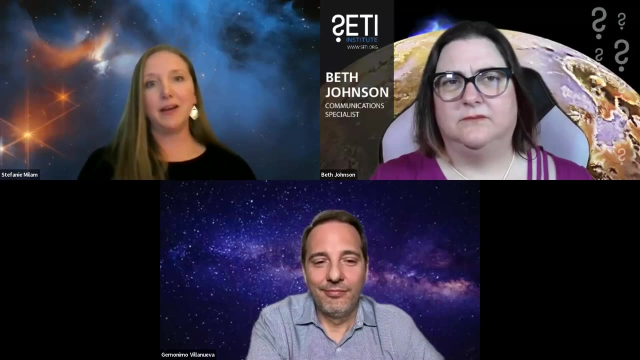 an instrumentation, sort of accessibility, to do the science that the community, the solar system community, really, really wanted to do. And so I was a planetary astronomer and spectroscopist and they, they thought that I would be a nice addition to the team Goddard did, And so they encouraged me. 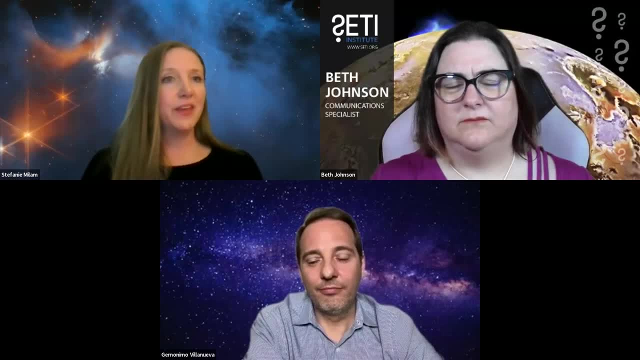 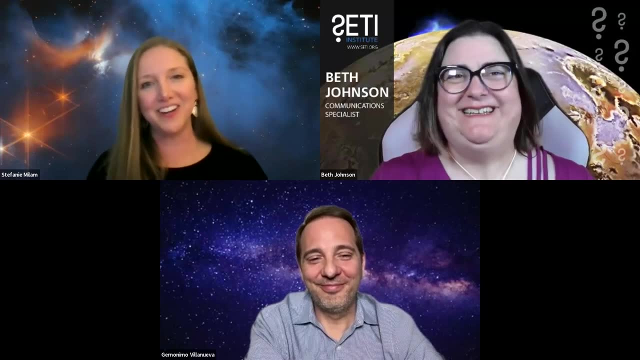 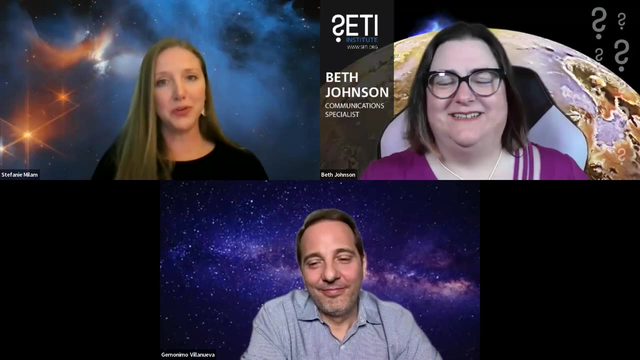 to apply and I was fortunately selected. And then I had this whole project, you know, this billion dollar project- sitting on my desk now And I had to figure out not only how to be a commentary scientist, but how to observe every object that this telescope could point towards. 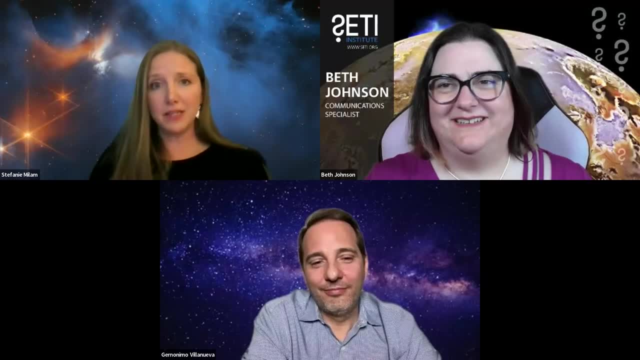 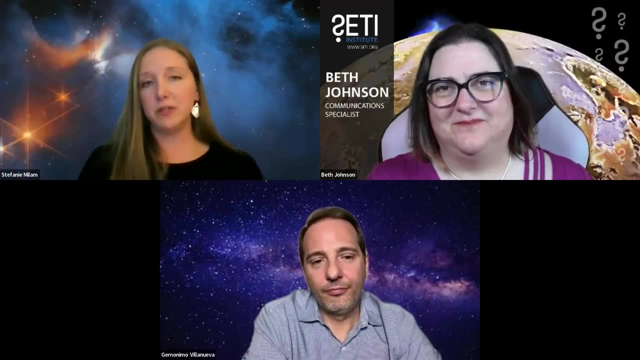 in the solar system and find out if that science case that the community really, really wanted to do could be enabled by the James Webb Space Telescope. So I reached out to the entire solar system community- multiple forums, multiple ways- and a lot of people were. 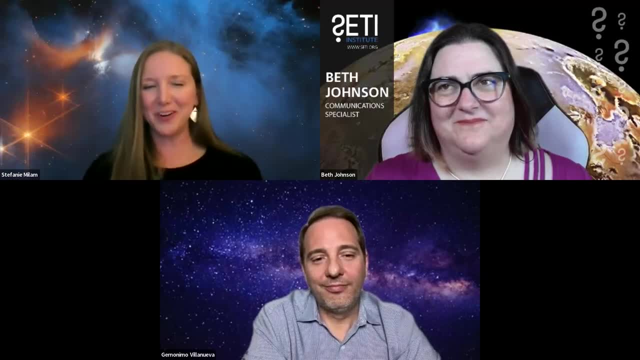 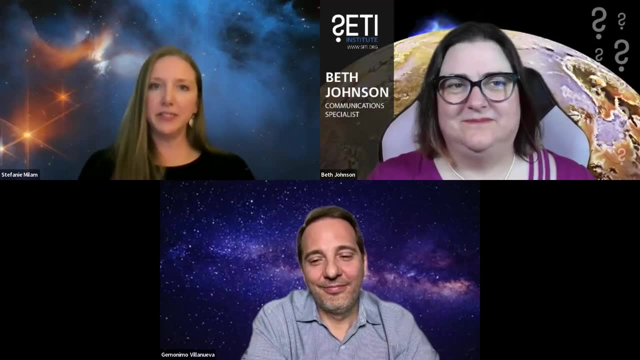 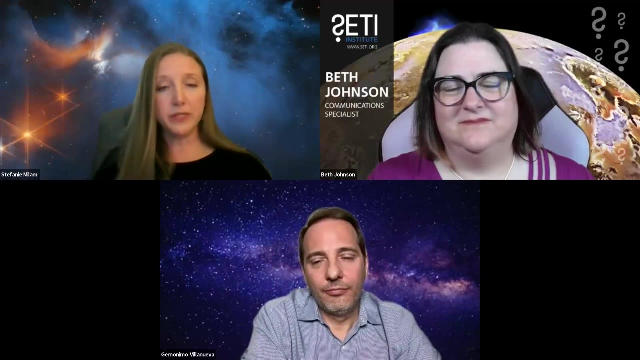 very receptive, but some really weren't And I had to twist a lot of arms and convince people. you know, I know we're not launching for a number of years and it was even less years at the time, but we really need to get the work laid out now so that we're ready to go when the telescope does. 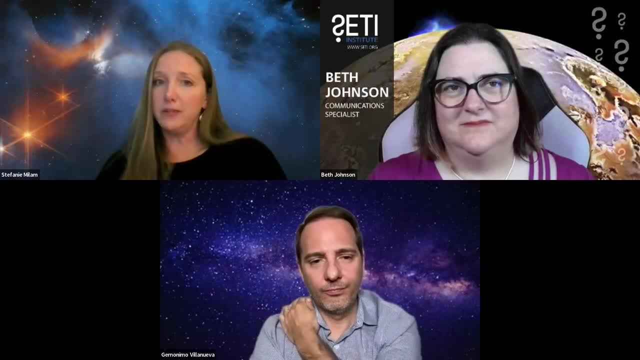 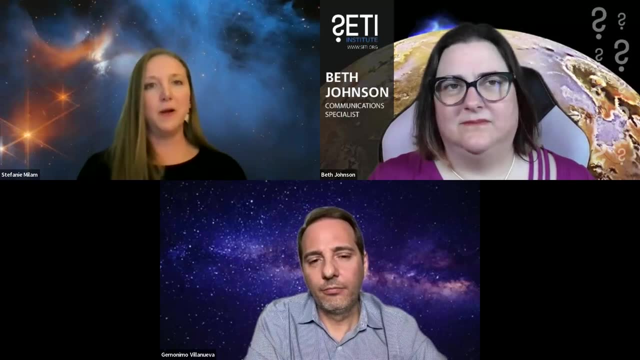 launch, because we were anticipating anything from a four to 10 year mission lifetime, not this 20 years. So we didn't want to have to wait and figure it out after we launched, And so Geronimo, fortunately, was very receptive when I asked him about a Mars science case. 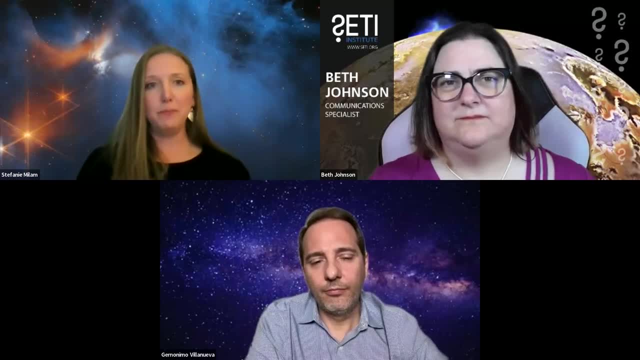 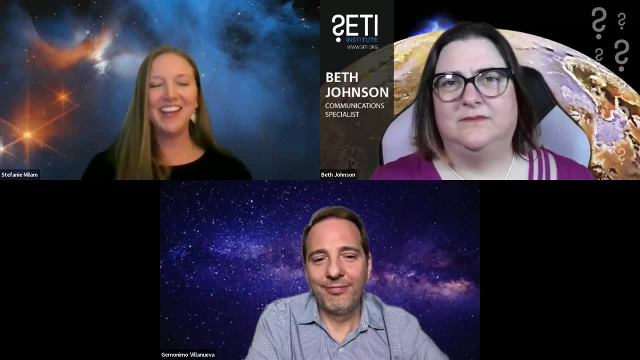 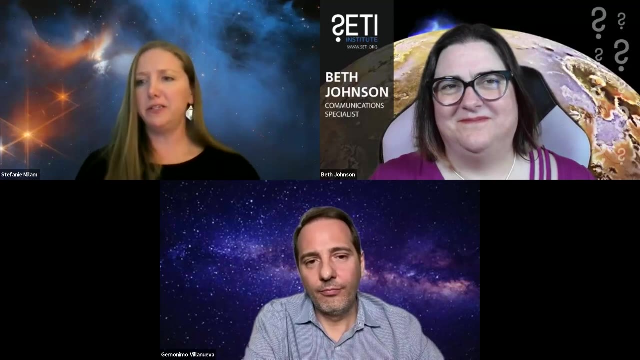 And he helped me work through that. We published a paper on the types of science we are expecting or hoping for with the James Webb Space Telescope. He showed you some of his methane predictions And a few years after that we were getting ready to get our cycle one guaranteed time programs. 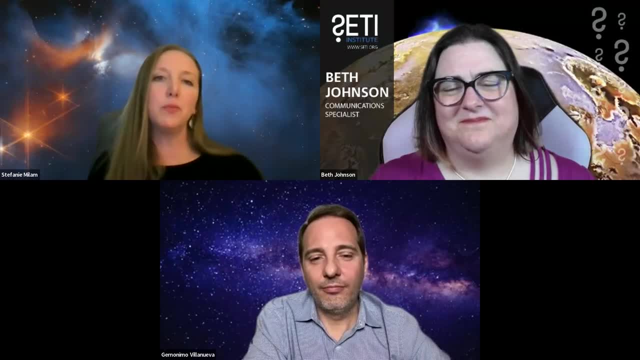 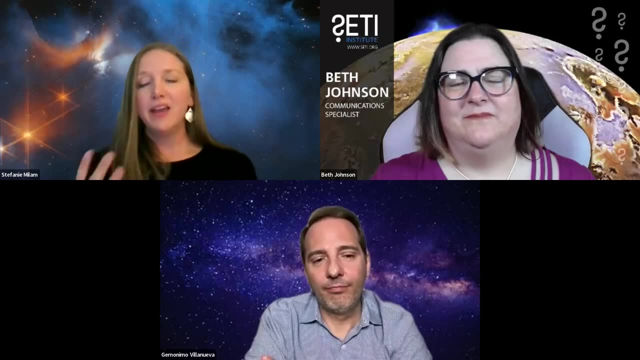 established and submitted so that the community knew what science we wanted to do in the guaranteed time programs, so that they could compete for time to do other things in the solar system. And I saw a gap and the big gap was ocean worlds And I was like, oh no. 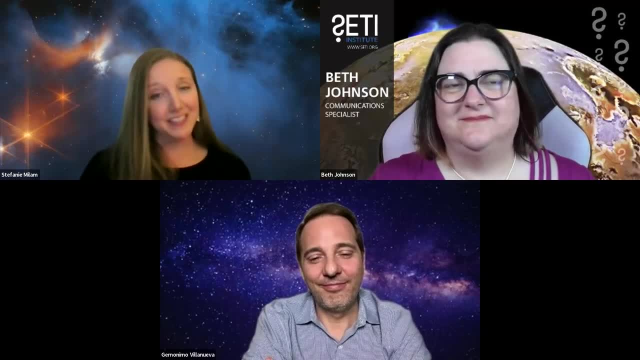 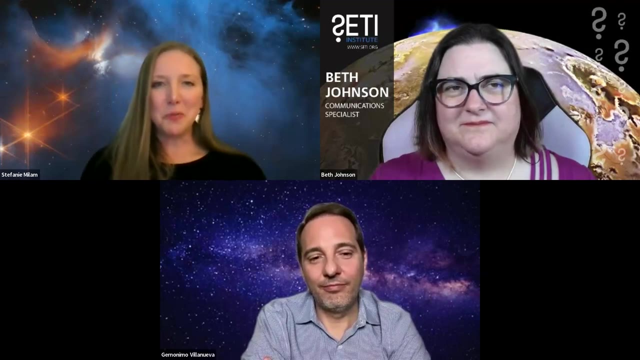 what am I going to do? And I had already worked with Geronimo on the fantastic graphic that we'd for the Europa simulation with the James Webb Space Telescope, And so he stepped in at the last minute- him and a number of other people that he'd worked with before- And we were able to get a Europa. 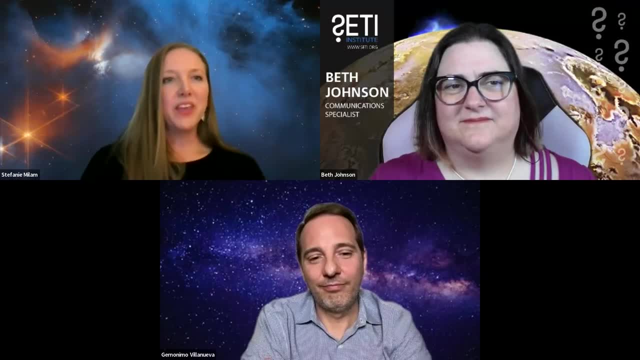 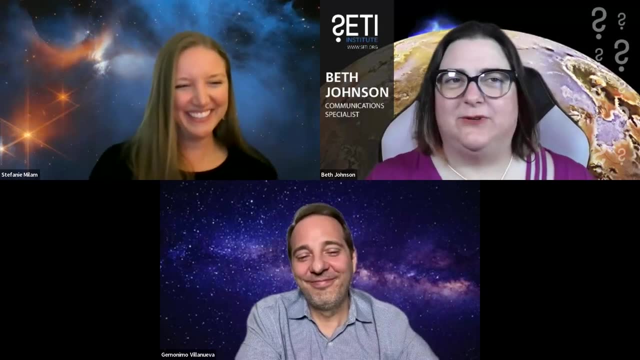 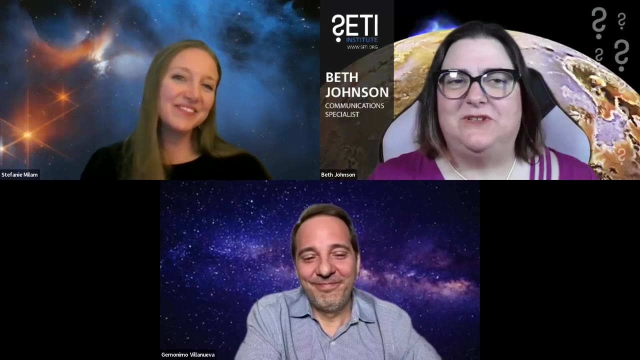 and Enceladus science case established, And so he came in, whether or not he liked it, and ended up having to work with me. No pressure for either you or him on this project at all, I see. So, Geronimo, what did you bring in when you came in the door? What did you find? 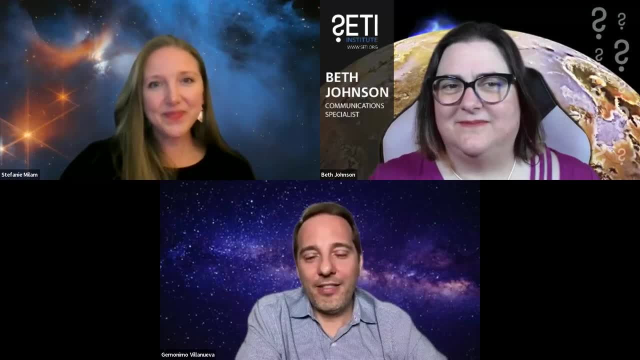 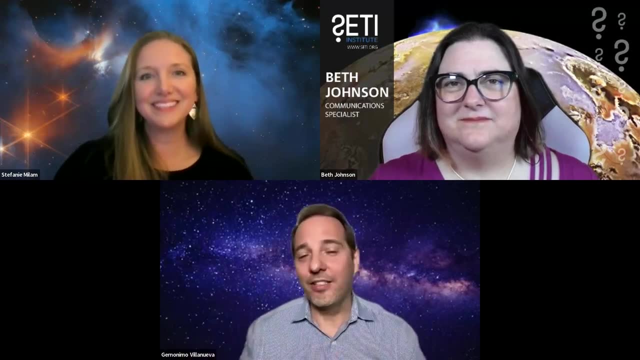 Yeah, it's definitely. I mean the amazing thing. you know, when we think about a NASA center, they tend to be normally focused on mission development, you know, and normally the astronomy side of things is focused on galaxies or other things. So planetary science is very 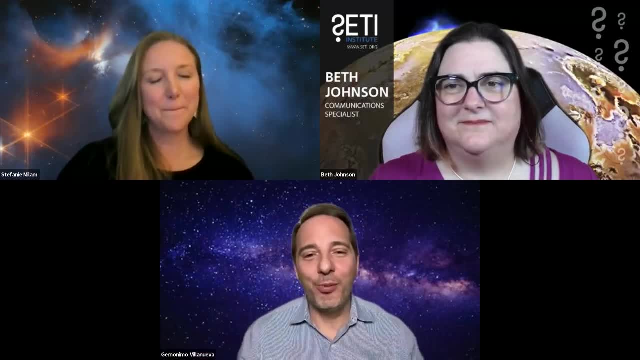 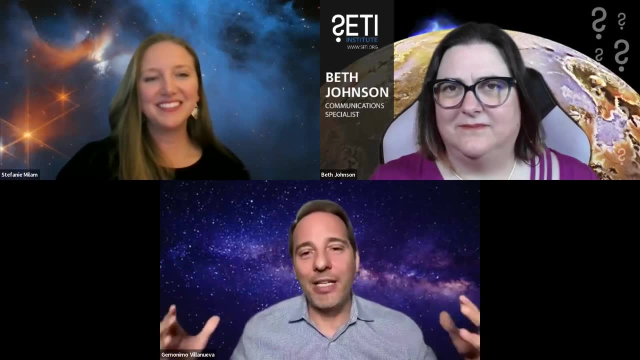 typically in situ. So we are a small cadre of people at Goddard who do? I mean we do use telescopes with the ground and a few telescopes out there, but you know it's not like we are. we don't dominate, We are not the dominant force at Goddard. So 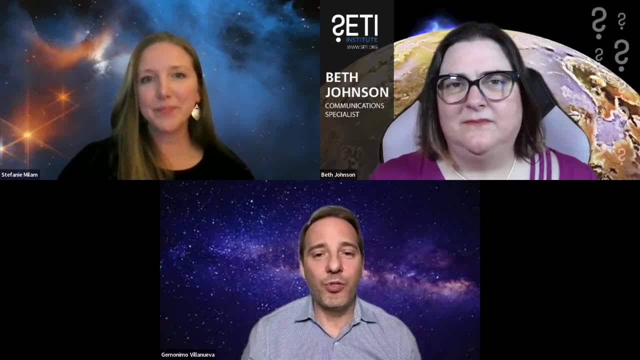 when Stephanie was leading all this effort with GenWeb. it was a great opportunity for to get involved in. you know this thing. It was in the future, but we saw that there was a new golden opportunity here to do great science And I think, if you ask me, the chances to work with 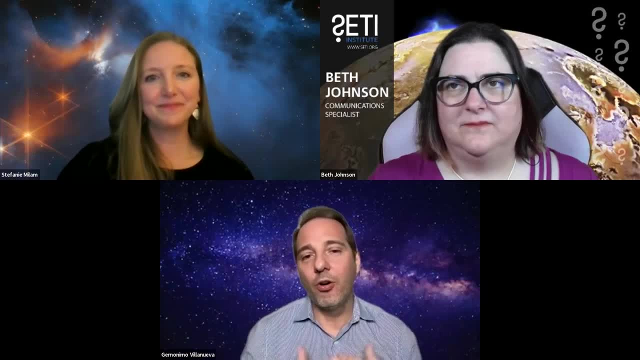 things like Mars or the Ocean Wars studies. they're fascinating because they're all related to astrobiology, The you know the things that are very interested in searching for organics, water, the origin of life and things like that. So it was a fantastic duo And I have to say as the data is coming now, after you know waiting for a couple of weeks, you know waiting for the data to come in. you know it's going to be a lot of fun And I think it's going to be a lot of fun. 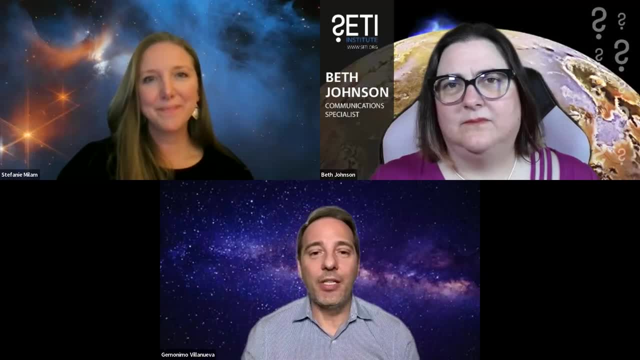 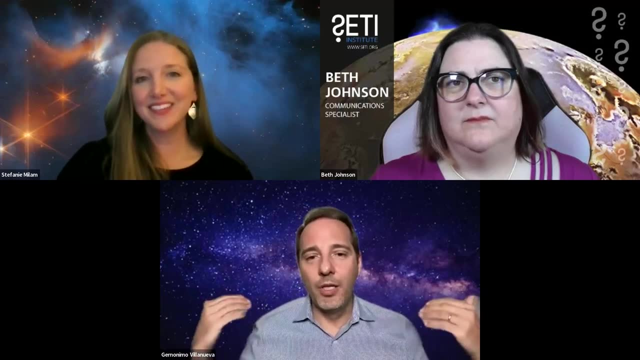 is coming now after you know waiting for so many years and you see it happen. It was. you definitely see, the collective knowledge of having people like Stephanie that push for the solar system research and all this team behind our teams that we have The Mars team, is huge. 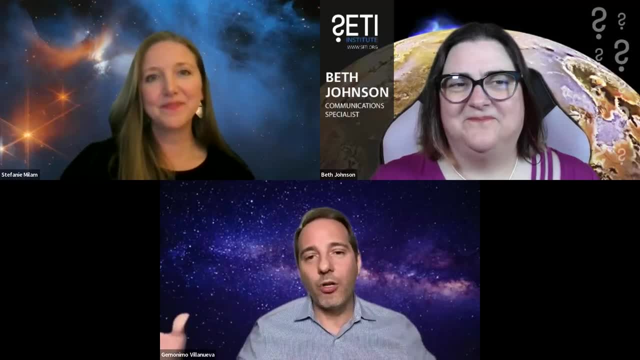 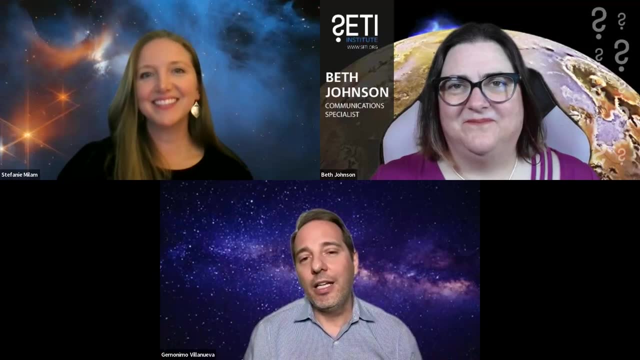 The Ocean Wars team is big, So these are big groups of people that we all worked together many years to get these, these results out And it's paying off because definitely GenWeb is going to- if you ask me, is definitely going to be there for many, many years. It's. 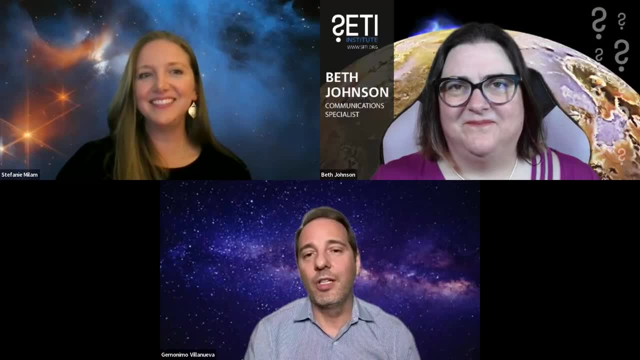 going to produce incredible science. I mean, we already see it with the Ocean Wars and I'm and you will. we're going to hear more stuff from Mars and stuff. So I think you know at the moment it was more like like, oh, we will see what happens. 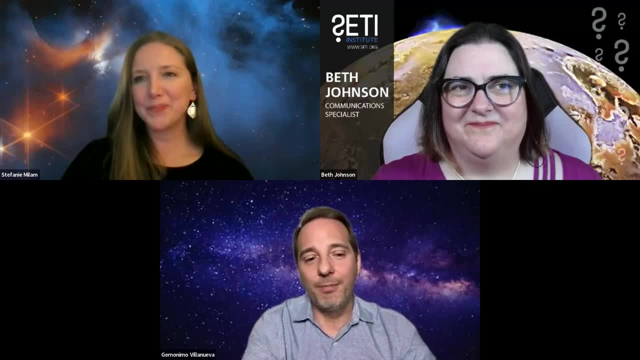 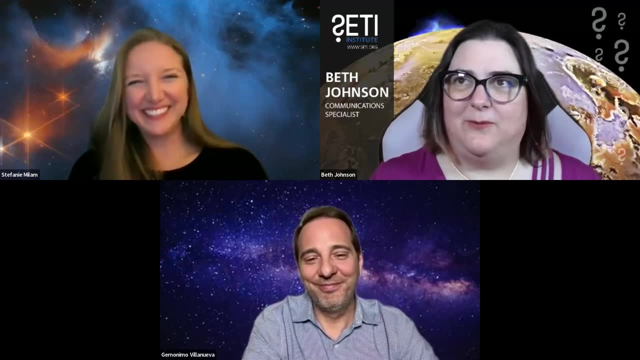 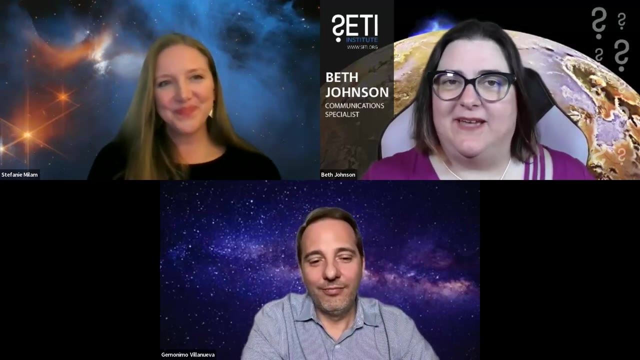 but now it definitely is. you can see the results coming out already. Very fascinating. So, speaking of results, cause we're? we're already at four, Okay, Whoa. All right, We are. we're 40 minutes in. Just a reminder to the audience, please put questions in the Q and A. 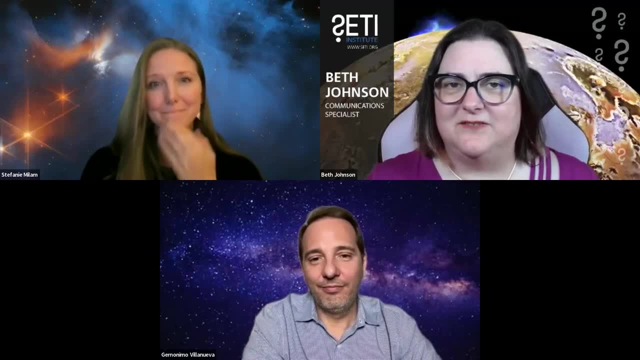 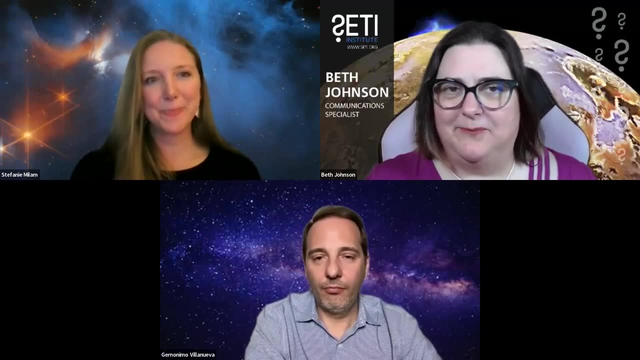 I've got a handful of them now, but if you have questions for our, our speakers, please put them in there and we are going to answer them, Thank you. Let's talk about some of these results. There have been a couple of major papers. 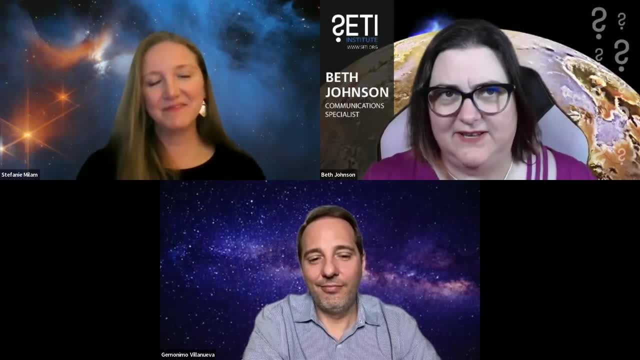 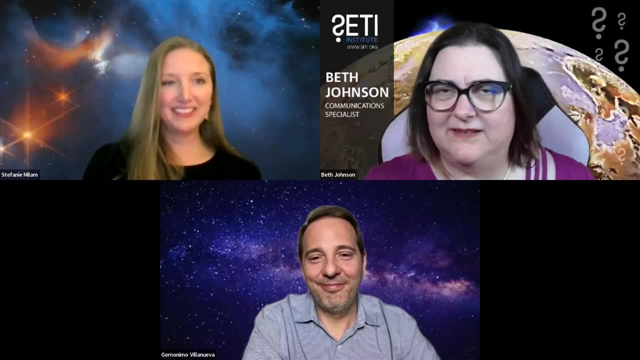 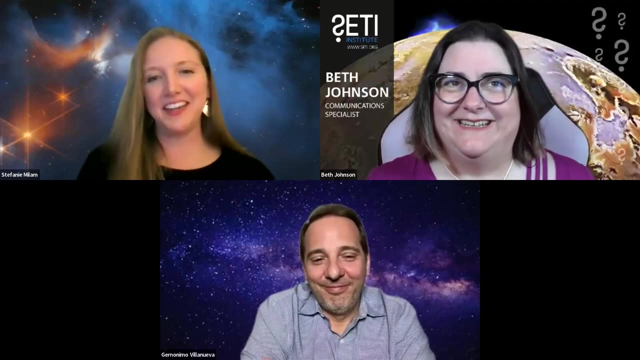 that came out that have been very exciting. Stephanie, yours was first, So we're going to start with you. You had some water from a comet that's in the asteroid belt, Yeah, And you said it exactly as we said it when we saw it, So I'm going to share this present. 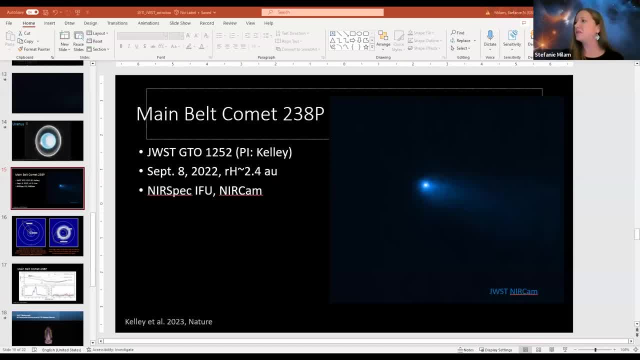 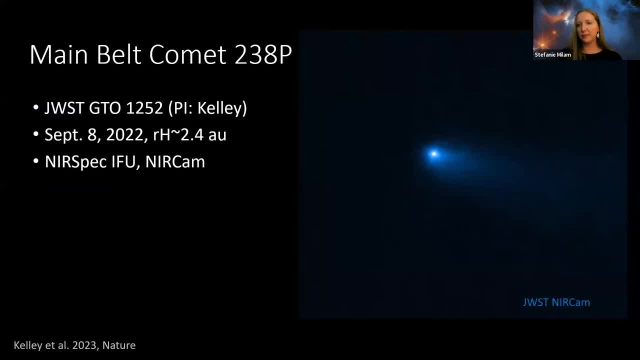 a couple of slides just so Everyone can see what I'm referring to here. So we had a program, All right. So I already kind of briefly talked about the guaranteed time program, And so these were a number of observations that were were set up and already in the queue in. 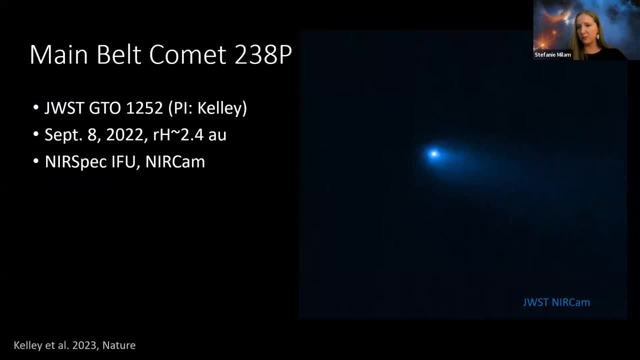 2017,, I think, was when we did our final submission And, as you know, that was with the anticipated launch at that particular time of 2018, and then it got bumped a little bit. and then it got bumped a little bit, which, for most planets, or 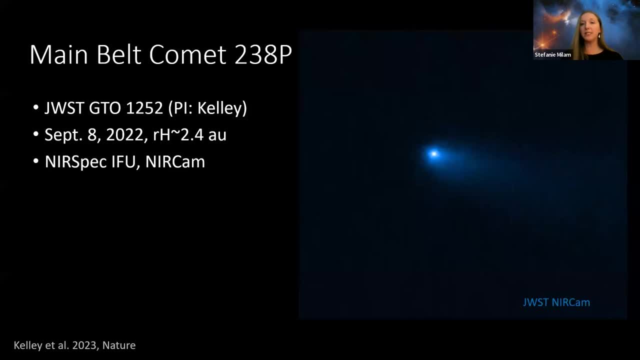 objects that are nearby us. that's fine because we get to see them about twice a year or per observing cycle. But there are some objects, namely asteroids and comets, And if we were ever lucky enough to get an interstellar object again, you get one shot pretty much in a 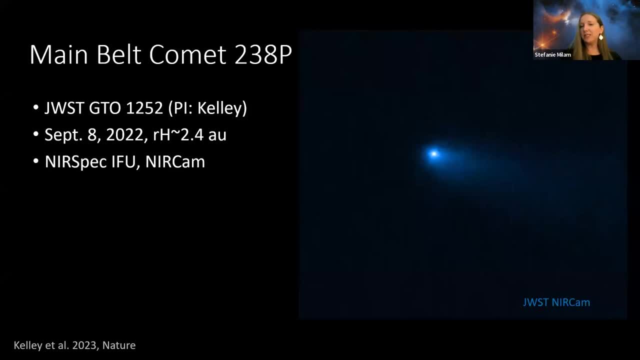 of year span, Even periodic comets. they come around every couple of years. Asteroids are every couple of years that are in the main belt because they move so slow, And then if we get a new comet, who even knows if it's going to last or survive coming into the inner solar system? So 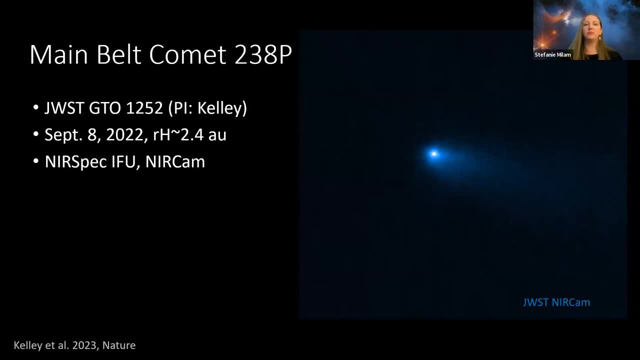 one of the programs that we had was to observe periodic comets, And unfortunately, with one of our launch delays, that comet moved out of what we call the field of regard, So JWST could no longer observe it the first year of science, And so we submitted a target change request And 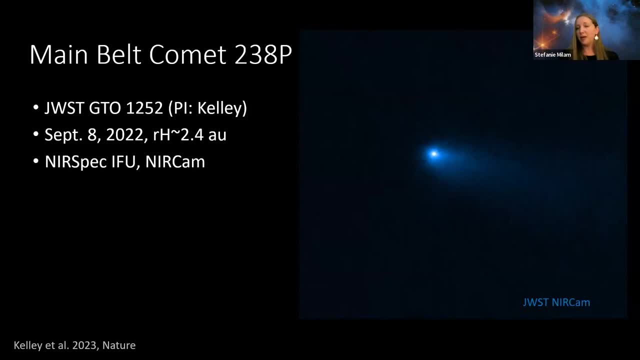 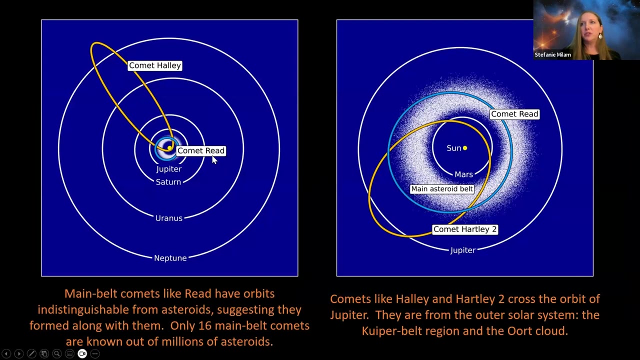 the person that was leading this program- his name is Mike Kelly- at the University of Maryland, decided that he wanted to try and see what JWST could do on one of these main belt comets. So these are objects that reside in the asteroid belt, So this is showing you where they actually. 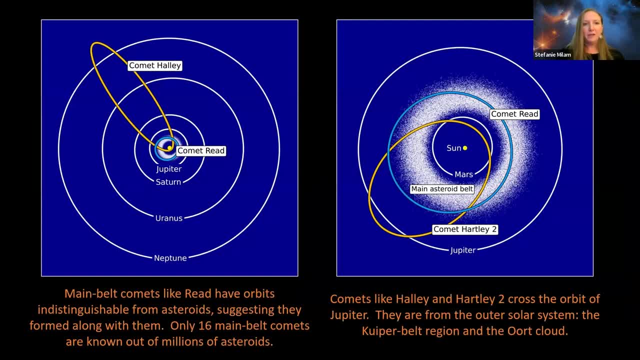 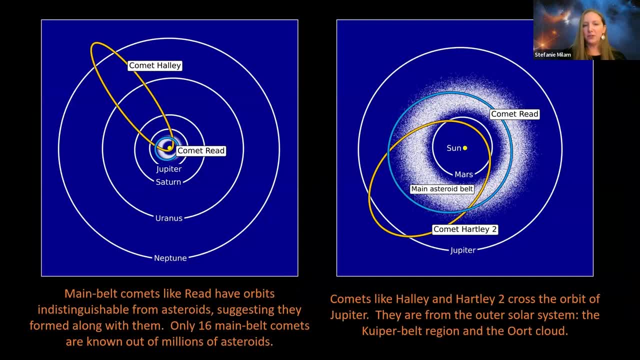 the asteroid belts, a fuzzy little circle on the inside, on the left, and then the fuzzy circle on on the right, And it resides between Mars and Jupiter. So this is where most of our asteroid population actually lives, And there's a handful of these objects, a dozen or so that actually 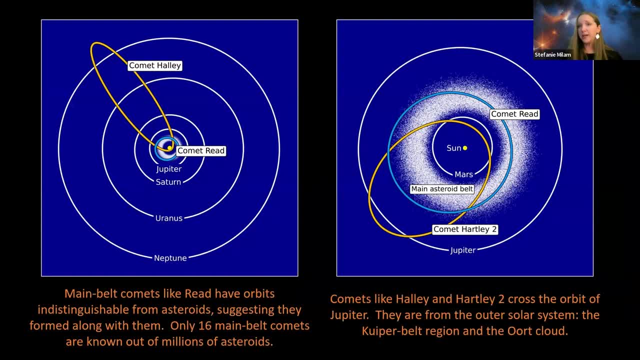 are fuzzy. they don't look like regular solid asteroid bodies And we've been observing them for years now with every big telescope there is in and out of this world trying to see why they had a fuzzy coma. So they looked like a comet, but they lived in the asteroid. 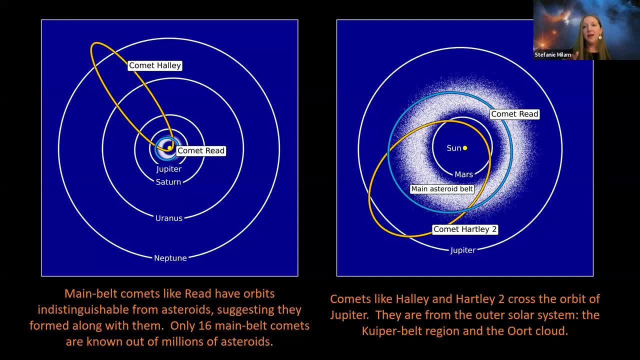 belt, And there's no reason there should be any activity of an object, a rocky body, in the asteroid belt. It's too close to the sun for water to actually exist- water, ice- And then it's also far enough away that you wouldn't have a chance to see it, And so this is showing you where they. 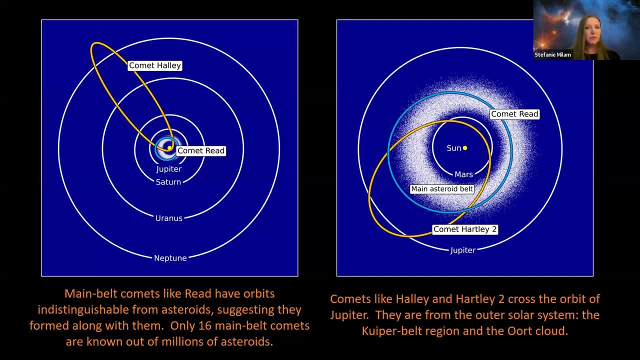 have liquid water beneath the surface. There's been results that alluded to hydrated minerals, maybe, and asteroids, but nothing real, definitive and definitely not anything volatile or you know, an ice actually turning into gas and driving a fuzzy appearance of a body. 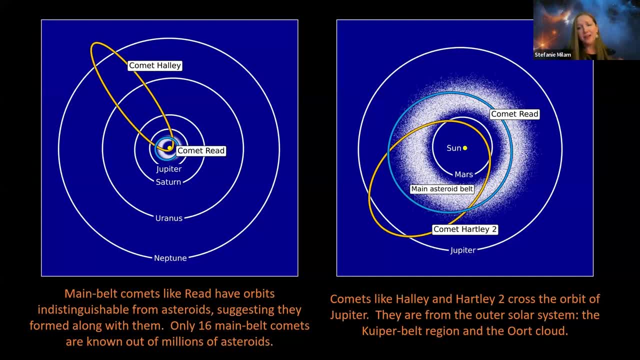 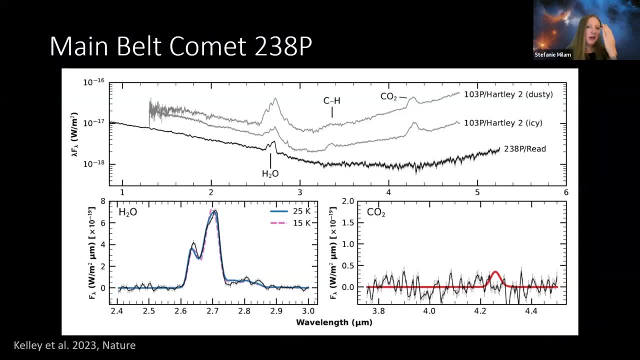 Anyway. so we thought it was a great idea to give us a good try, because if anything's going to detect anything, it's going to be JWST. And lo and behold, we detect water vapor. So this is again some of the spectra that Geronimo was talking about. So we're looking for these sort of blips again in these lines that are indicative of different fingerprints of given molecules. 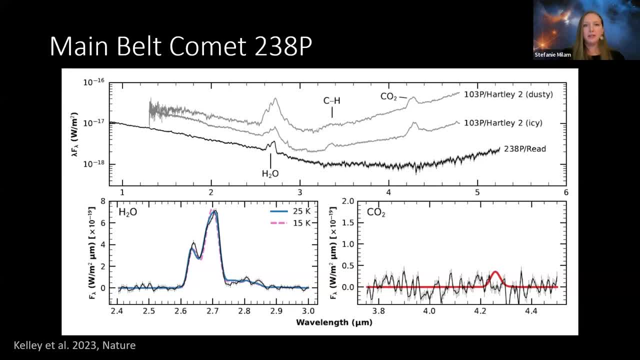 And so on the top panel, the black line that spans on the bottom, that's the comet, the main belt comet or active asteroid Reid, And then there's two other comets that are observations that were from the flyby mission of the former Deep Impact spacecraft. 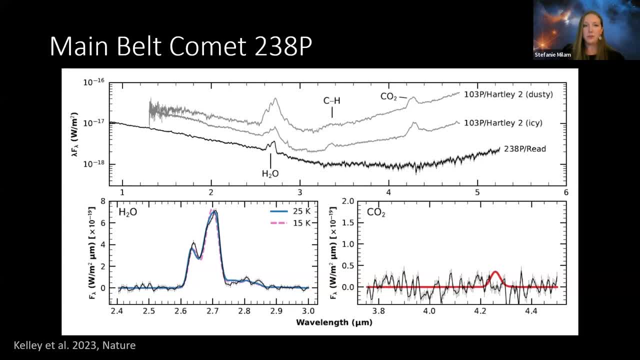 It was the epoxy mission that flew by Comet 103P, which is a periodic comet, And not only is the water emission absolutely booming in this main belt comet or asteroid, but there's no carbon dioxide. Every comet we've ever looked at with these with access to 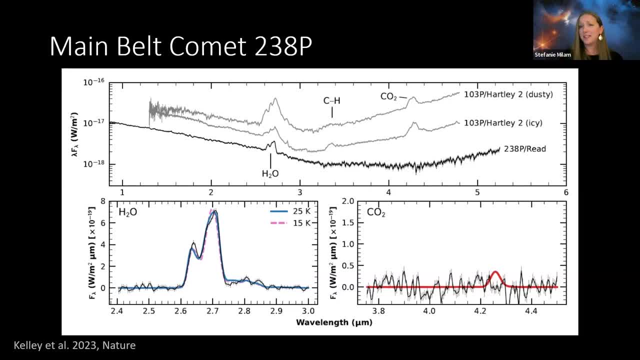 the carbon dioxide fingerprint has a huge carbon dioxide signature. It is the most obvious thing. So now we know that there's water ice, that somewhere in the subsurface of this asteroid type body. no carbon dioxide, but at least we're getting some clues that water actually exists in the inner solar system. 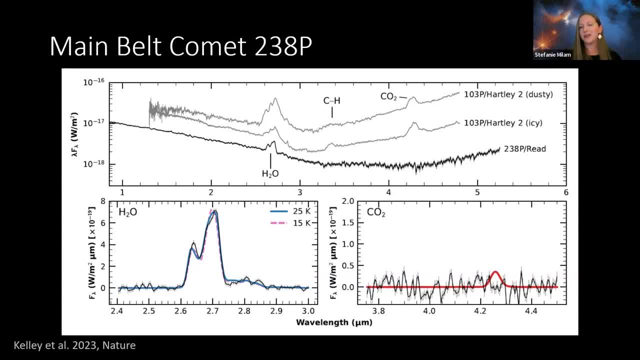 And that's that's imperative information. And the more of these objects we study, the more we'll learn about what the actual composition is, how much water or other gases may be present. This has huge implications for delivering water to Earth or other terrestrial bodies. 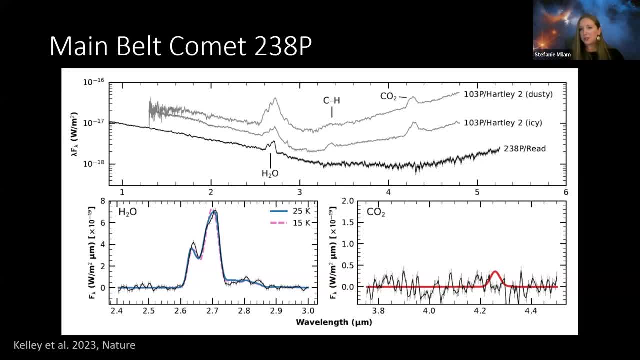 Statistically speaking, an asteroid bumping into another asteroid and getting knocked towards the Earth is a lot higher than a comet coming from the outer solar system and hitting us Even during the heavy bombardment era. most of those bodies now reside in the asteroid belt. 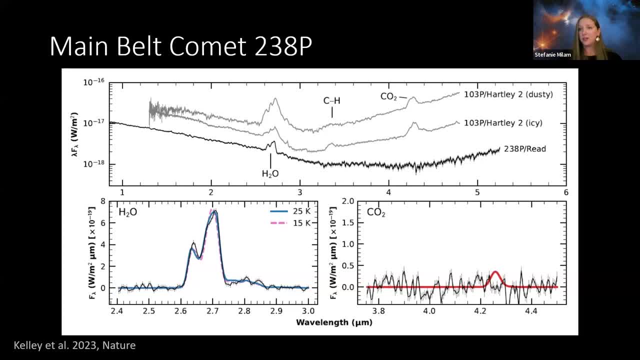 So having some preservation of water ice in these objects is huge for us, And it's very exciting to understand what the distribution of water across the solar system actually looks like- And JWST has that capability. That is fantastic, And thank you for explaining it so clearly. 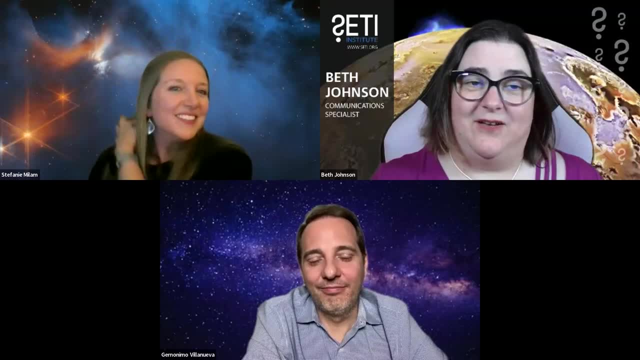 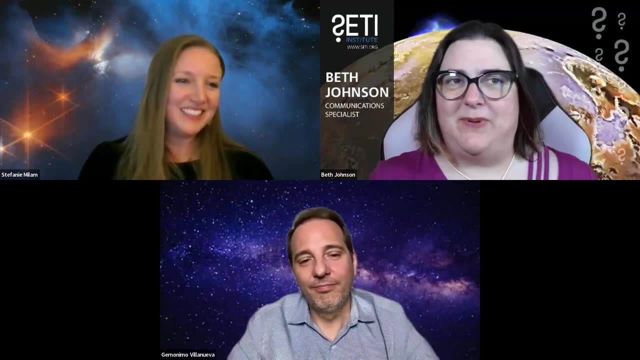 The carbon dioxide part was also fascinating. I mean, the whole thing is fascinating. It's just sort of a surprising result across the board. Geronimo, you had a paper. Well, it's not. the paper has been accepted. It's not actually published yet, but you can talk about it now. 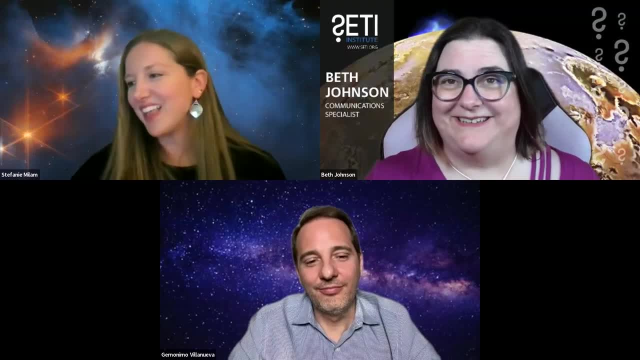 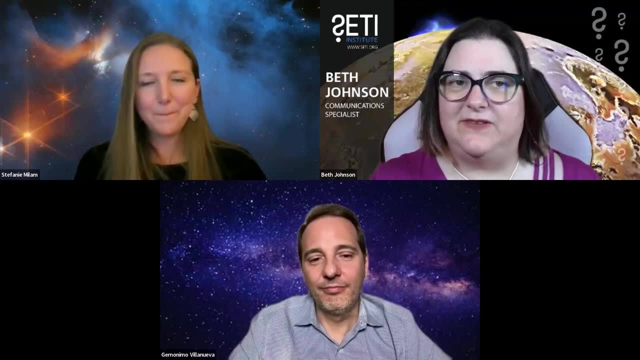 That came out just the other day, And this is about Enceladus, which you mentioned in your opening. So tell us about the research that you've done, the observations that were made of Enceladus and what you guys found with this plume. 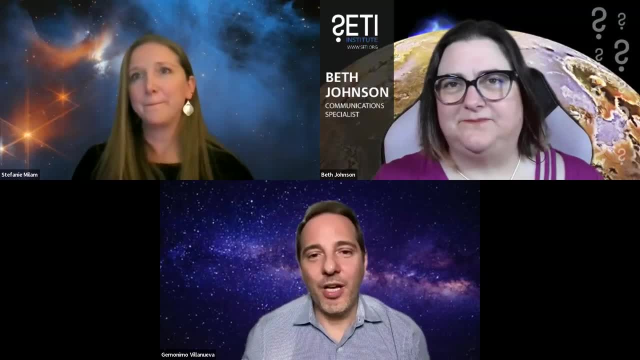 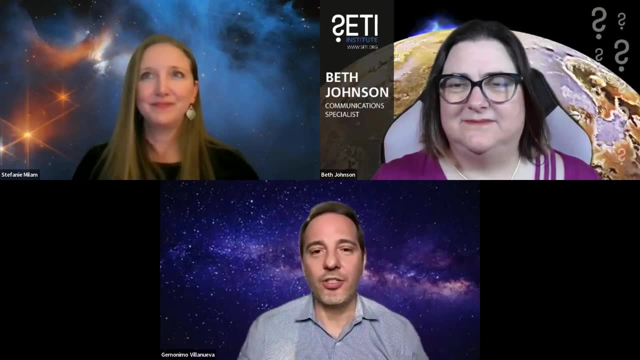 Yeah. so the big driver of me, when you're looking for thinking about astrobiology, is looking for the building blocks of life. So you want to have chemical diversity. looking for the carbon, you're looking for the oxygen, looking for the nitrogen, for the things like that. 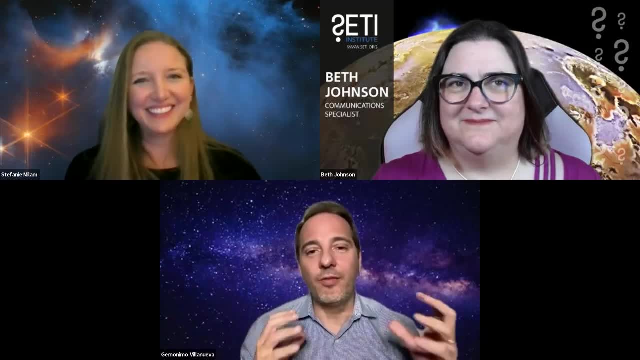 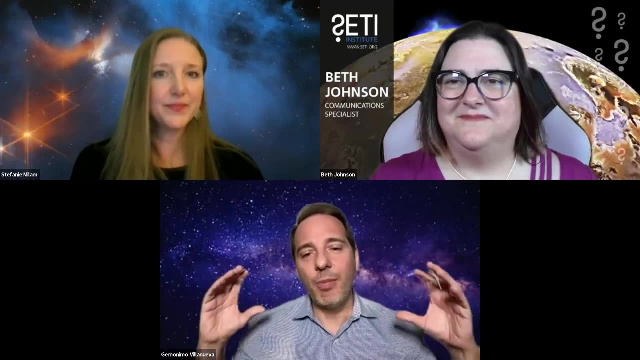 The John molecules And those are stored in different molecules. The main reservoirs for those molecules you have water, carbon dioxide, methane, ammonia. So these are big molecules that you're looking for because of the main repositories for those building blocks. 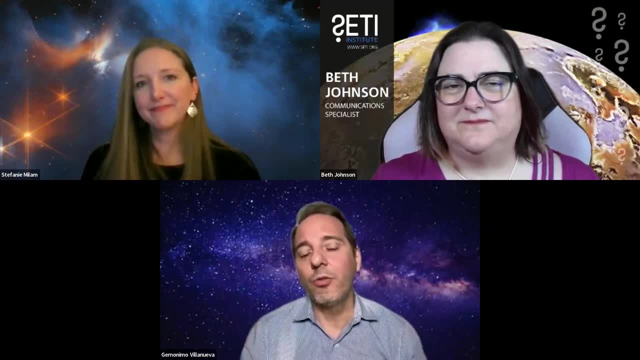 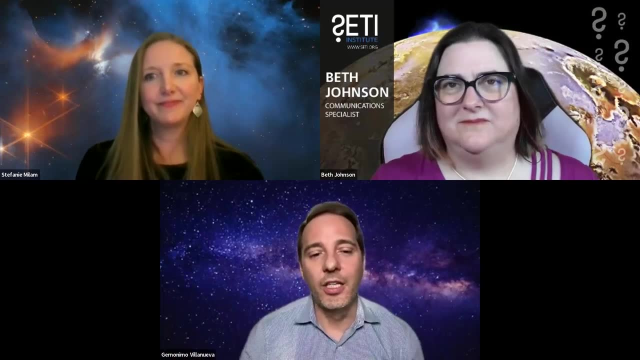 Then they produce more complex molecules that they are kind of difficult to do remote sensing on them because they are too big and they are difficult to do. So you have to focus first on the smaller molecules and see that the chemical diversity. So when we, you know for some, when you see water in a member of the comet, that tells you that you know maybe that water is everywhere. 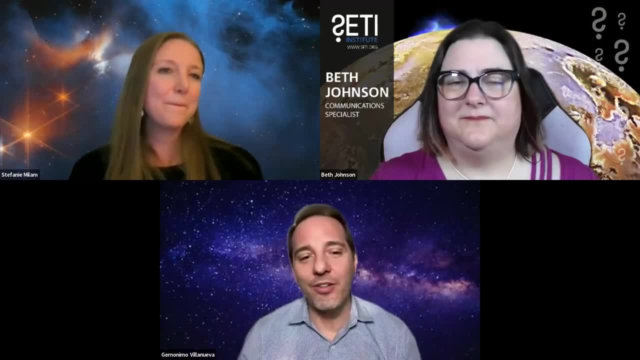 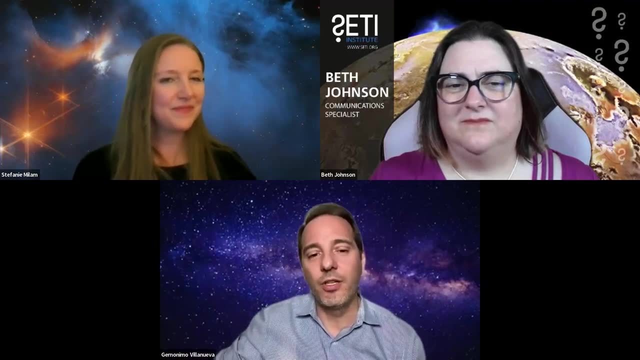 And that's what we're looking for, And that's what we're looking for. And then, when you point to Enceladus, you are looking at this, you know cryogenic objects which are very far away, And it tells us about the primordial conditions of the solar system. 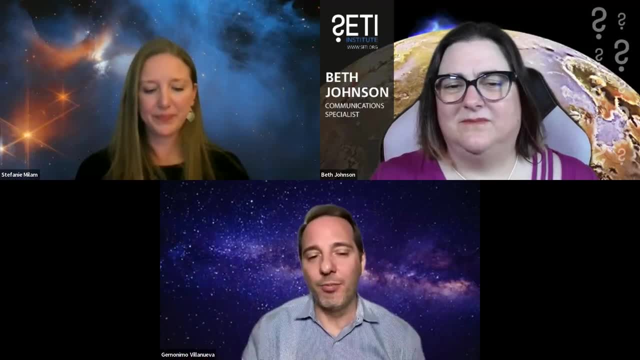 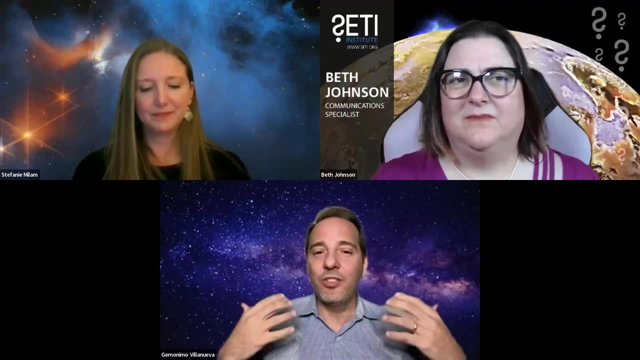 But also they may tell you that it's a habitable environment And the way to explore that is, first of all, unique energy and chemical diversity. So the fact that we saw this plume, massive plume that we were reporting just today, we see this huge plume coming out. 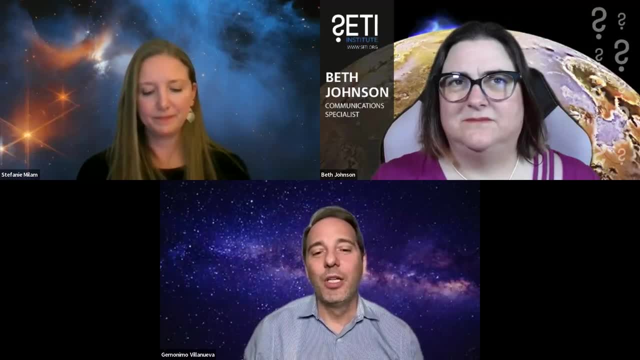 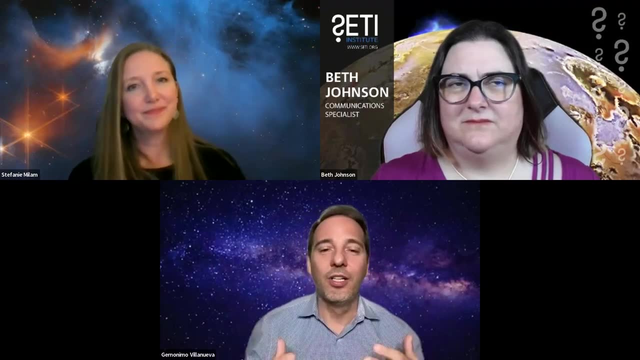 It tells us that at least there is water. We can see it in the plume, We can see the dimension. We can see the dimension of this massive jet of water coming out. that not only indicates that there is an activity or higher temperatures at a terminal activity happening on Enceladus, which is interesting for astrobiology reasons. 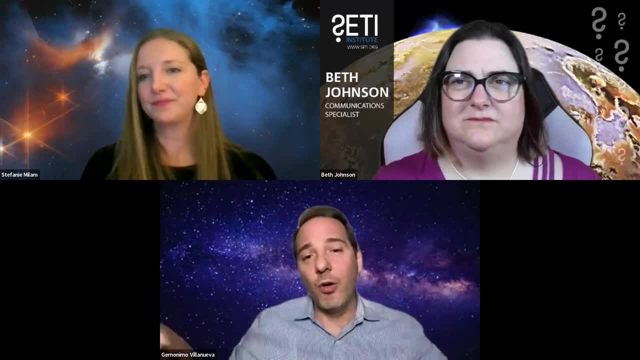 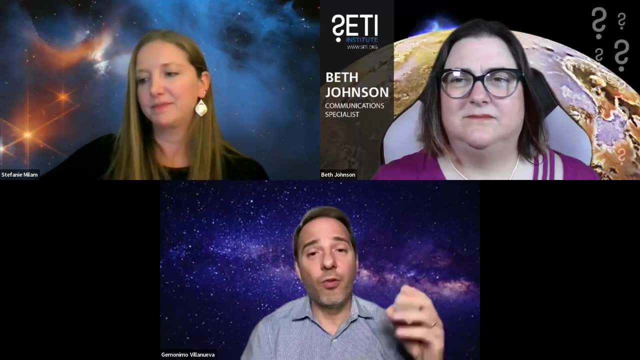 it also tells us that that water is going to be flowing away in the Saturnian system. So you have, you know, you are quantifying that source of water And these are trace amounts of water. So for someone, if you see trace amounts of water in the upper atmosphere of Saturn, you may know: oh, that water came from Enceladus. 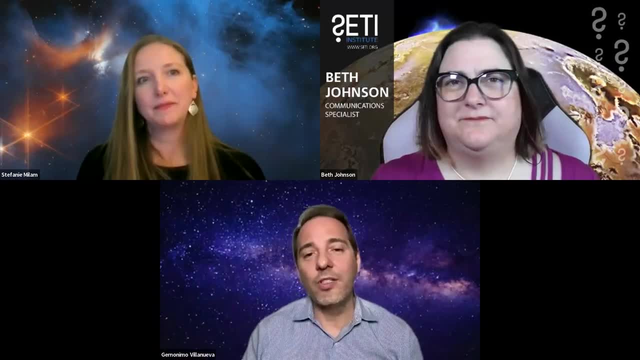 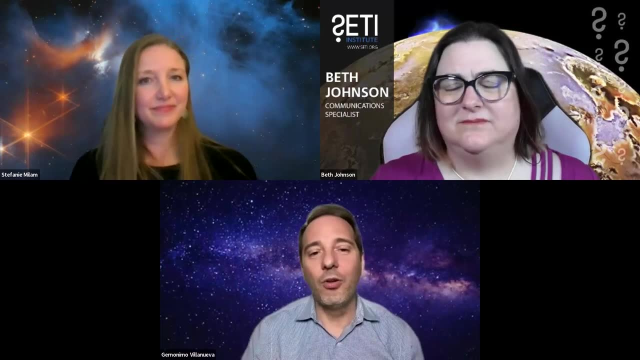 If you see a little bit of water in other moons in the Saturnian system, you'll know the source. So as you explore for chemical tracers, it's always important to know the origin of these molecules. For example, I know you're looking for a cryogenic place in an outer solar system like Saturn, Pluto. 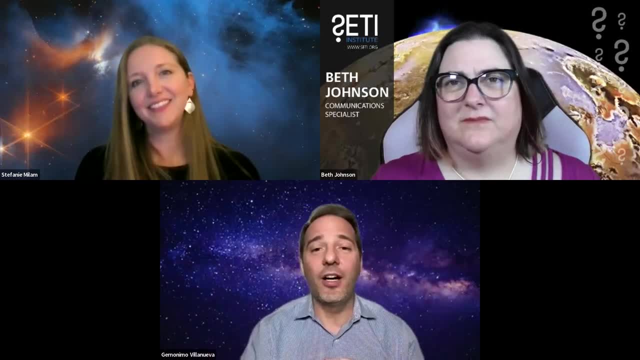 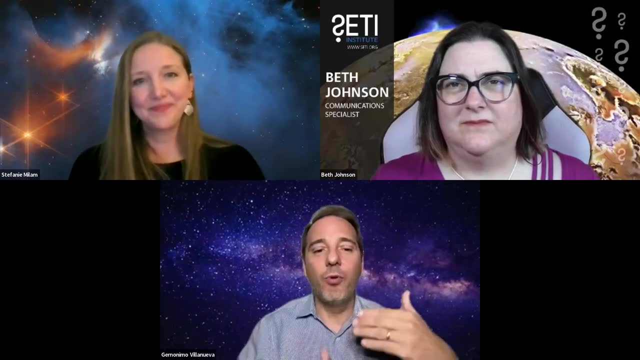 You need to understand that those molecules, how they got there? to see if there are. you know, something is happening on the surface or they were implanted from other sources' bodies. So these are evolutionary steps for us to understand more about how this water is being delivered across the atmosphere. 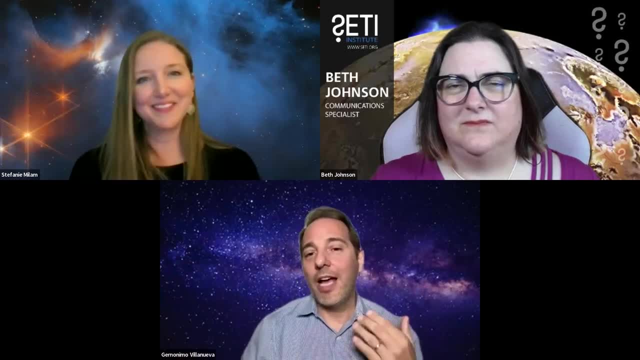 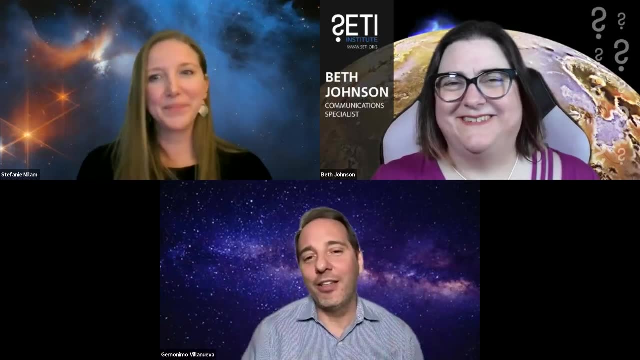 Thank you. And so how is this water being delivered across the solar system? Is activity going on And it may indicate that there is something happening on Enceladus below the oceans? And if you ask me, if you want to send a lander to Enceladus now, I would go to the South Pole. 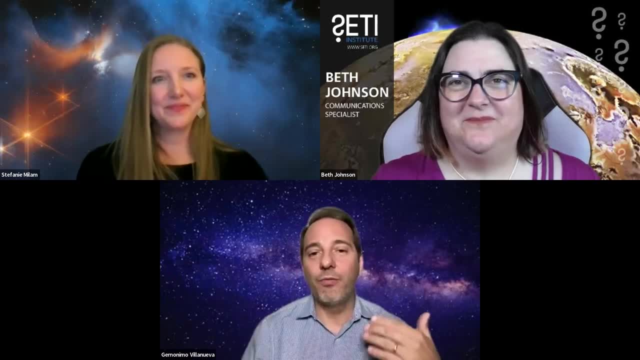 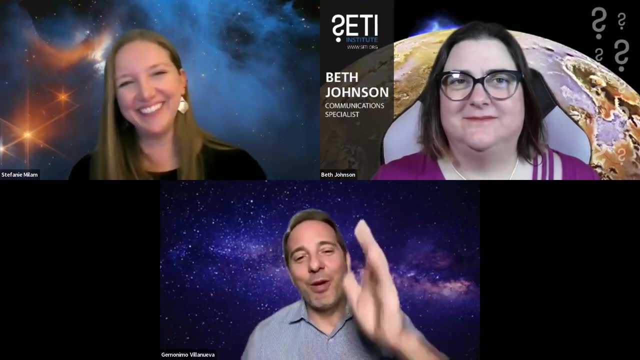 The fact that we measured that thing indicates that that activity is pretty constant over decades. So that indicates if you go there you're going to go to the geyser. You have to go a little bit away from the geyser, Maybe find a way to get into the ocean. 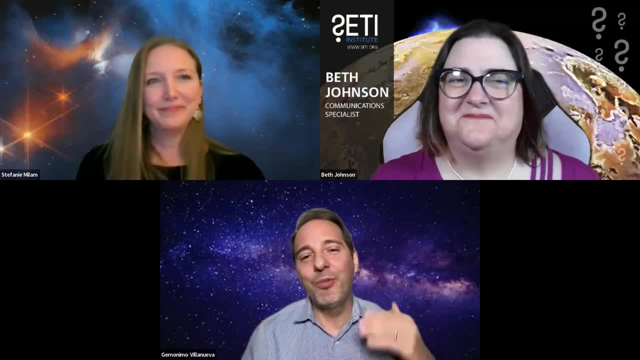 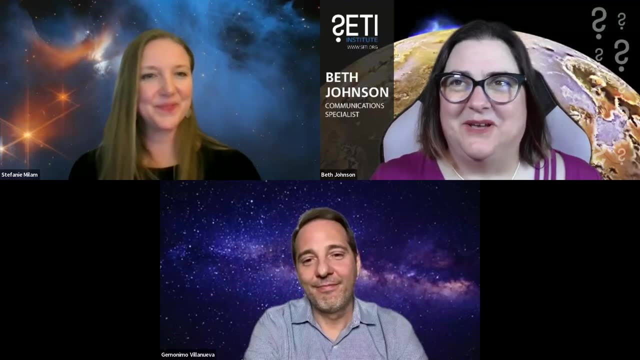 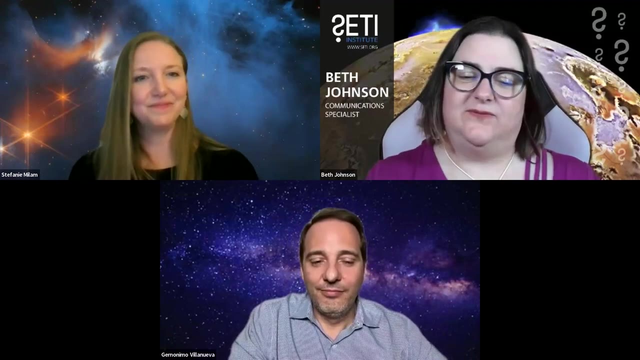 So I think those are interesting things that GENWEP can keep doing And we can keep doing those many other things. we can keep doing those measurements year by year. so that's those are exciting things about things like James Webb- Oh, fantastic. so all of this is sort of in a quest to find signs of. 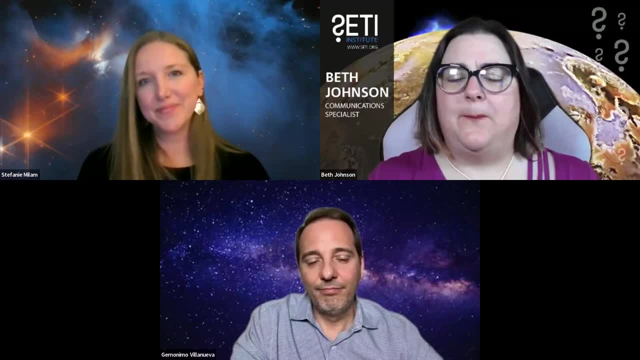 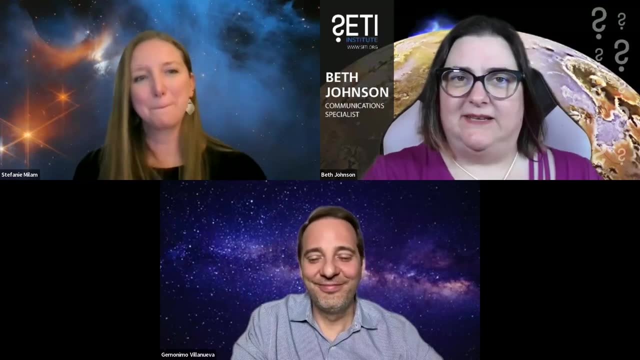 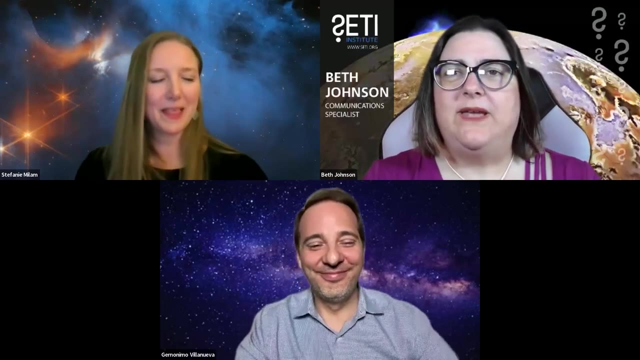 habitability, the potential for life. but I know you both want it clarified that you're not looking for life, that this is not a oh look, we found little green men. or or you know, look, there's a plant. unless you actually manage to find a plant, in which case hey great, but what, what do? 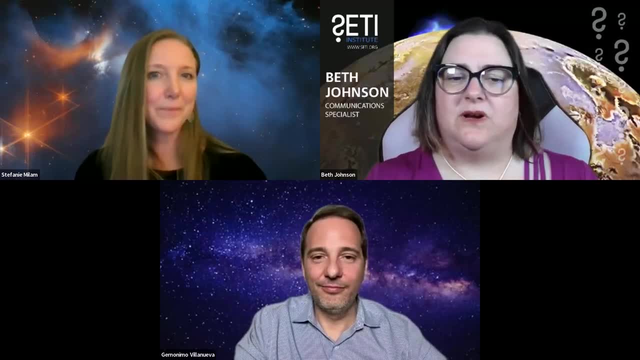 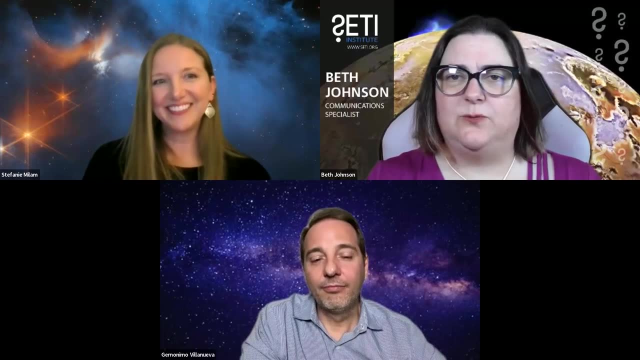 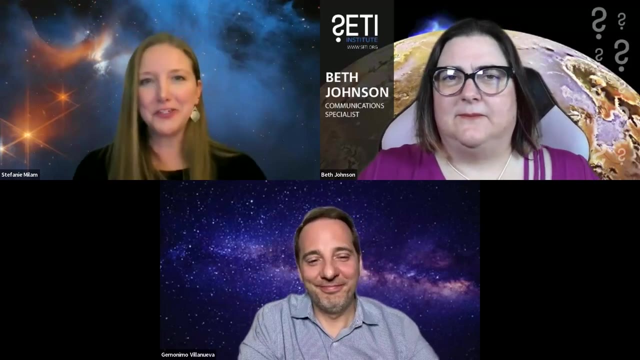 these? what are these molecules? what are these signs that you're looking for? tell us why these particular molecules. give us a few details between the two of you as to as to what all of this means and what it's used for. I'll give a. I'll go start. okay, so we're as, as you said, we're not looking for. 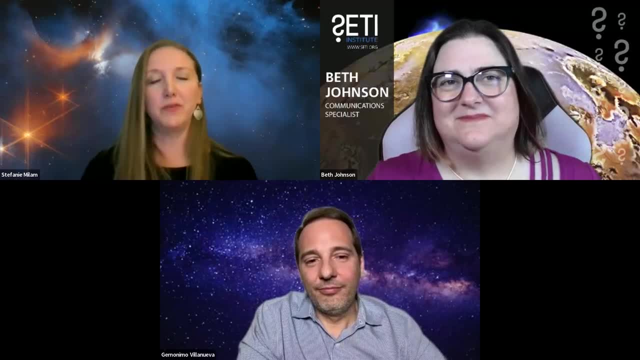 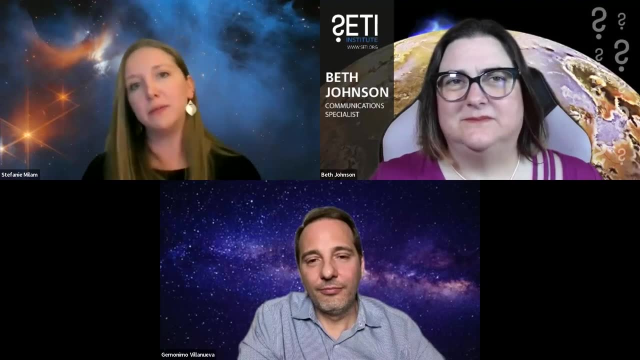 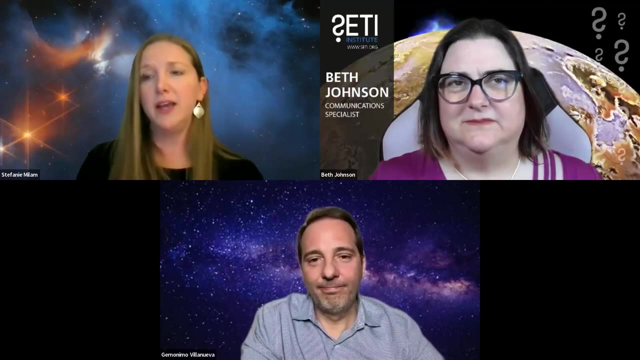 life itself, or technosignalism, or anything sort of on that kind of level, at least at this, at this point in time, mostly because the capabilities of the telescope are limited to infrared wavelengths. and what we're looking for are these, these key molecular fingerprints and something that would suggest something different. 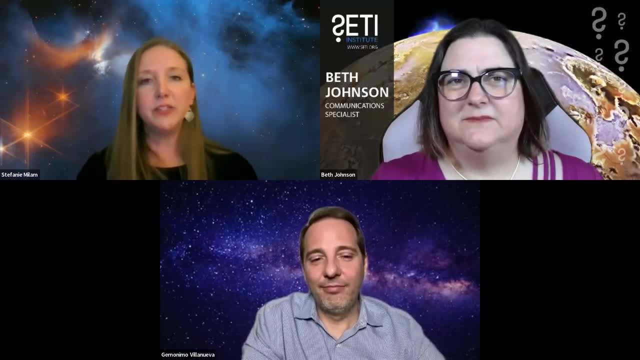 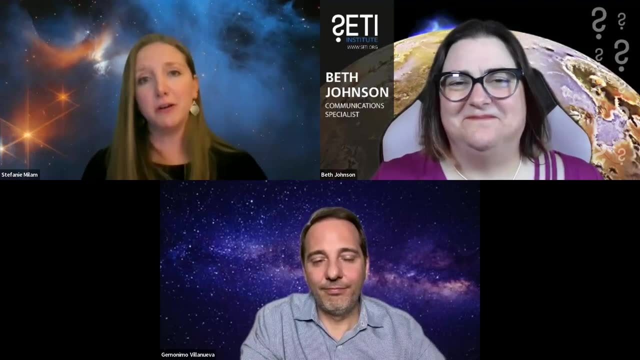 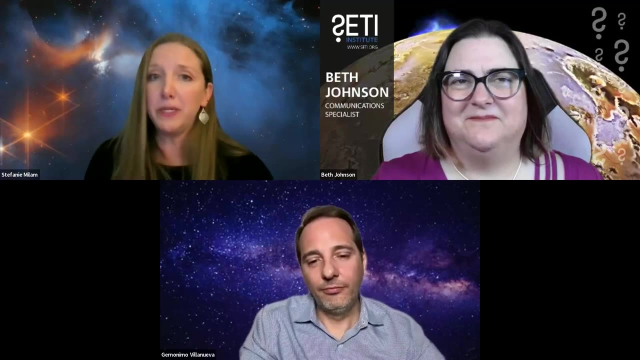 is happening within a given body, and so, as drama already beautifully showed us with those fantastic graphics, there's different processes that can actually alter the way that we're looking at the atmosphere of a planet, and that can be geology, that can be an impact event, or it could be. 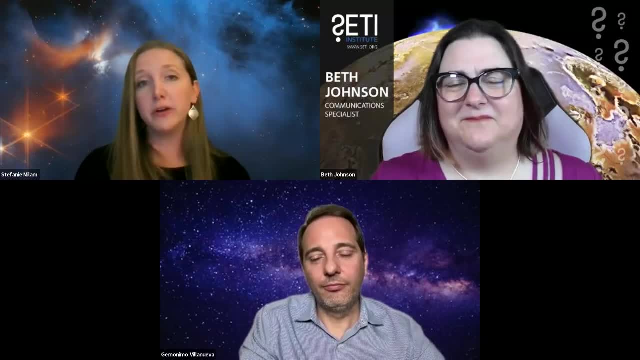 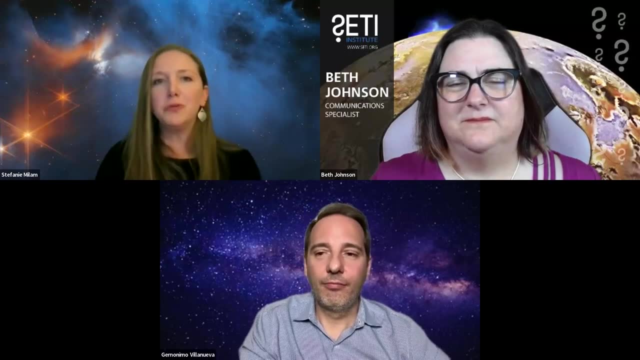 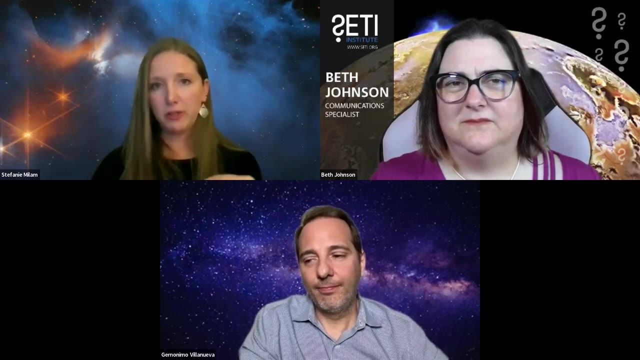 something like life. we know there's molecules in our own earth's atmosphere that should. that would not exist if we had a very neutral environment where the chemistry is in what we call equilibrium. it's these processes that actually throws that equilibrium off. and so, if we can see, 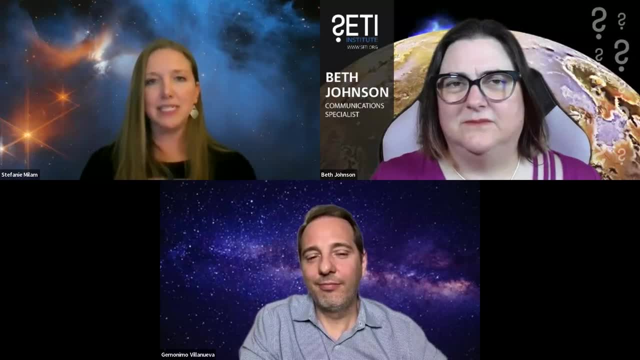 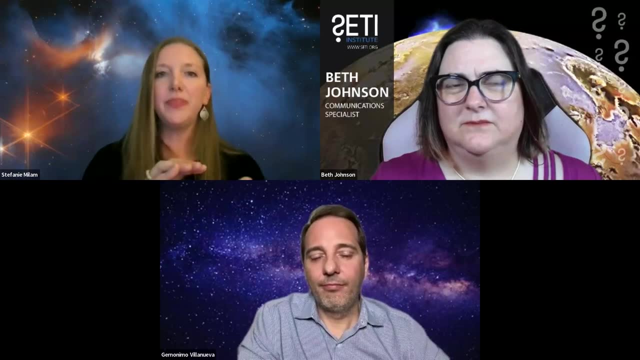 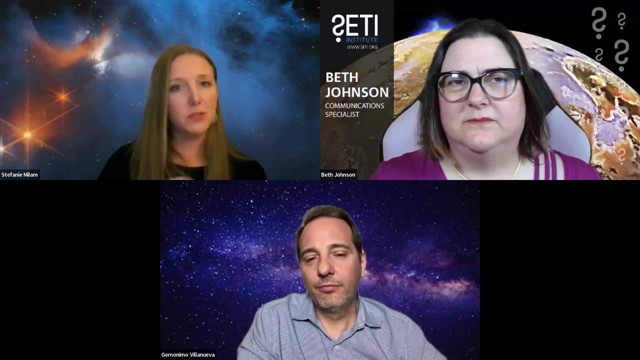 two molecules that would normally exist in a nice, happy, complacent environment, that are tending to fight each other chemically, then that's suggesting there is a process and that's why studying our solar system, even with the same telescopes, that's looking at for planets and other planetary systems, it gives 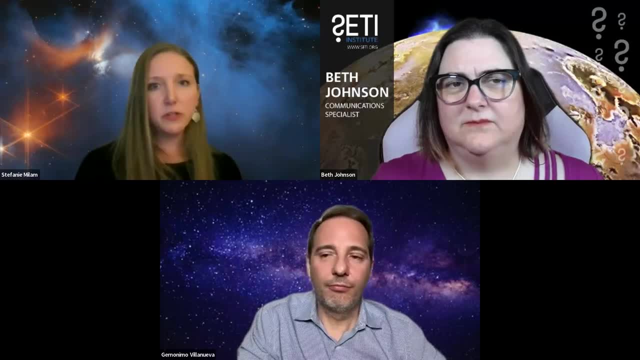 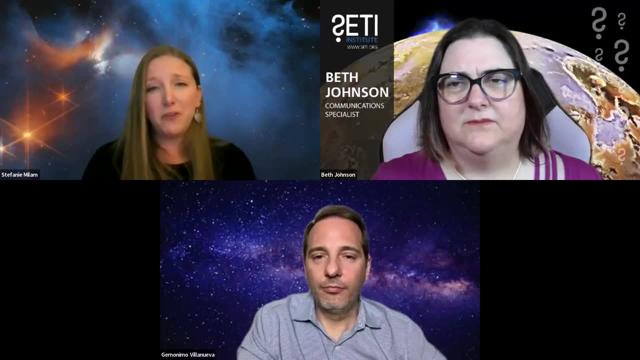 us the the context of what are the signatures that we can actually see, the processes that we actually know that are occurring in our own solar system, because we're looking at the universe and we're seeing the planets and we're seeing the planets and we're looking at the planets, we're seeing the. 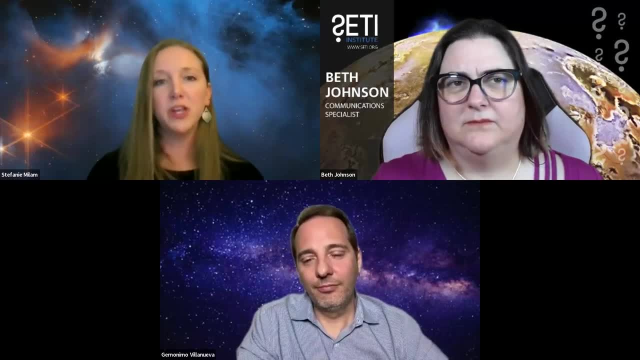 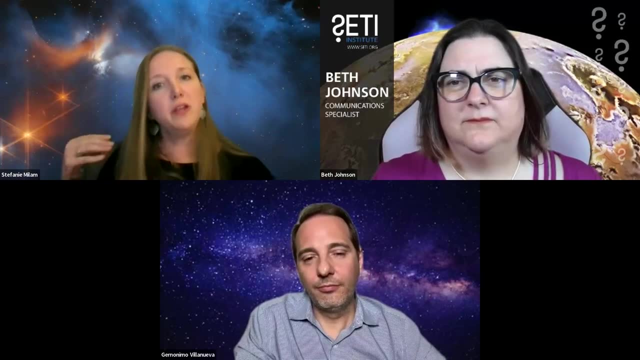 planets and we're seeing the planets and we're seeing the planets and we're seeing the planets. we've we've flown there, we we've sent probes, we've sent orbiters, um, we've landed on on multiple planets. now, um, we know what's going on in those environments and so, looking at them remotely, with 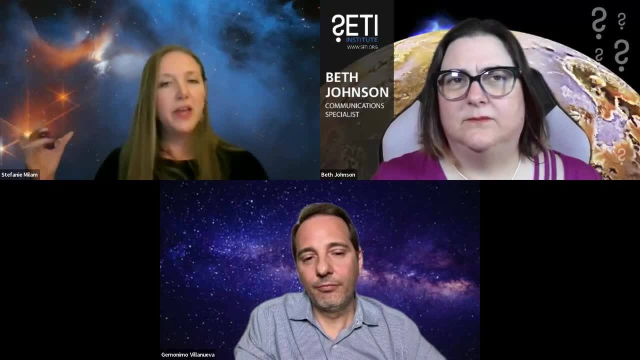 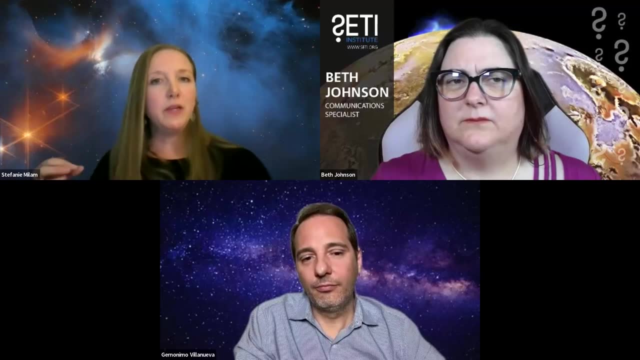 a telescope like hubble or the james webb space telescope. it gives us some context for what's happening on the surface, in the atmosphere, in the environment, but also what we can see remotely. in addition, we have molecular tracers or or instruments that can be used to measure the 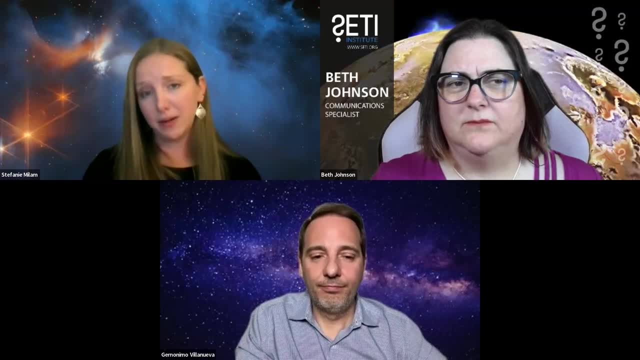 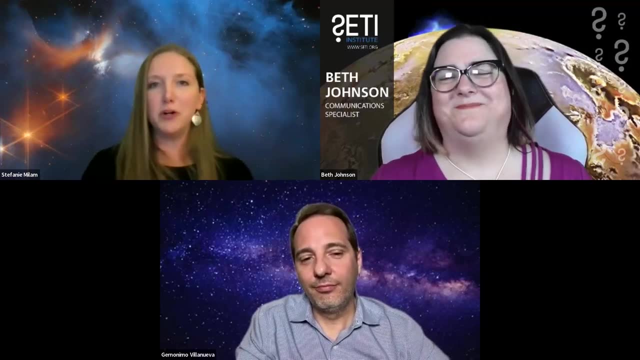 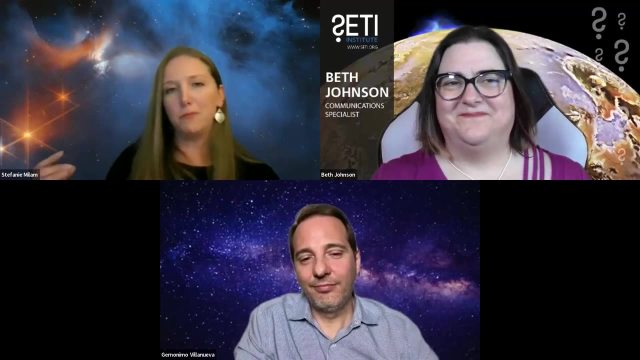 that has capabilities to see things that we can't see in orbiters. It gives us a nice global pictures of planets. We can see, you know, the sandstorms of Mars going all the way around the entire planet, or how the polar caps melt and move and migrate up, you know, from one to the other. 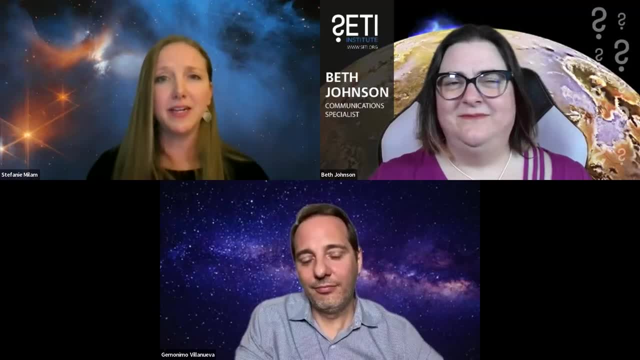 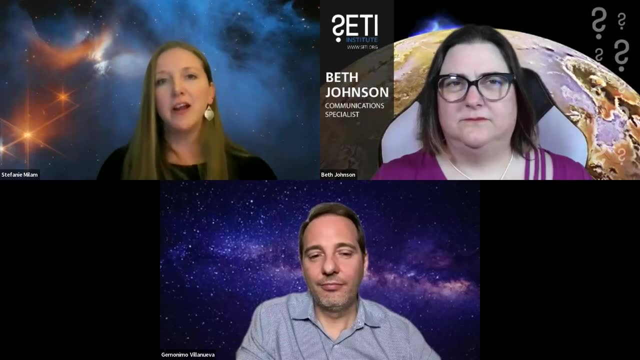 We can see how the environment or the atmosphere of Titan is dynamic, Jupiter, And that tells us a lot. So when we look at a planet around another star, we can determine how many, how thick the clouds are, how thick the actual atmosphere is, how hot the atmosphere, what it's. 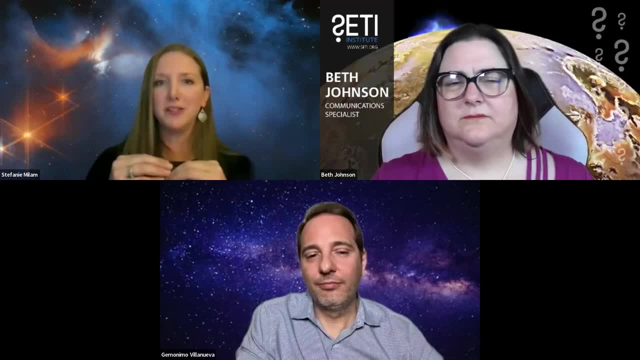 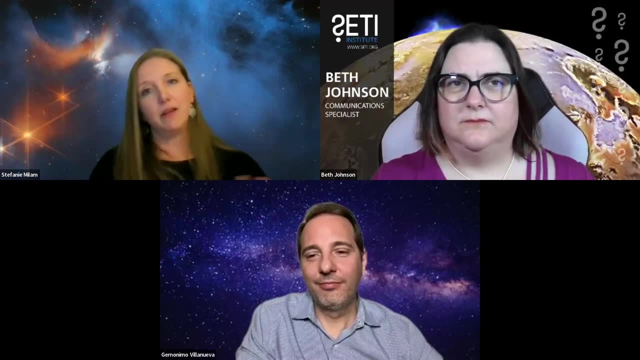 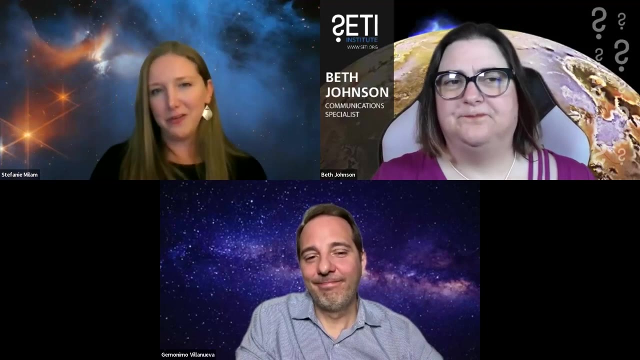 made of, And we can start looking for these little process signatures suggesting that something else is happening. It may not be obviously something like life, but at least it gives us a short list of objects So in future missions we know where to really hone in and put our energy. 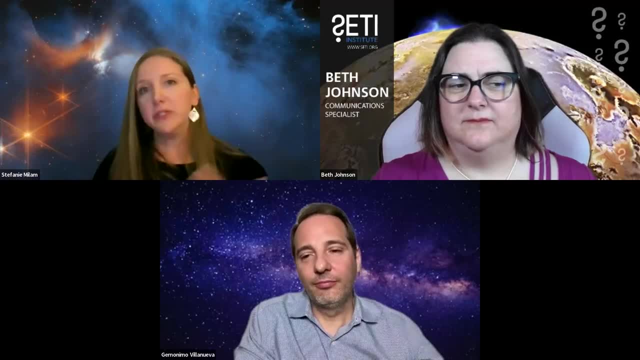 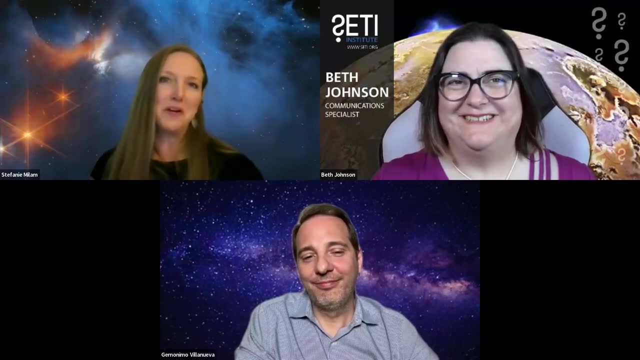 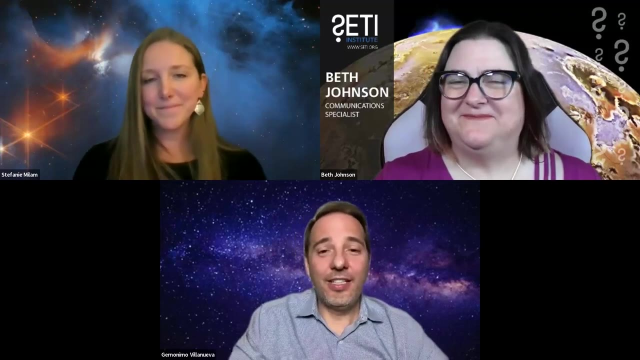 towards And look at those objects much closer, with different telescopes, different techniques and maybe even some crazy day sending probes or whatever elsewhere in the universe to try to explore those regions. Geronimo, Yes, Yeah, exactly What Stephanie said: the idea of this. 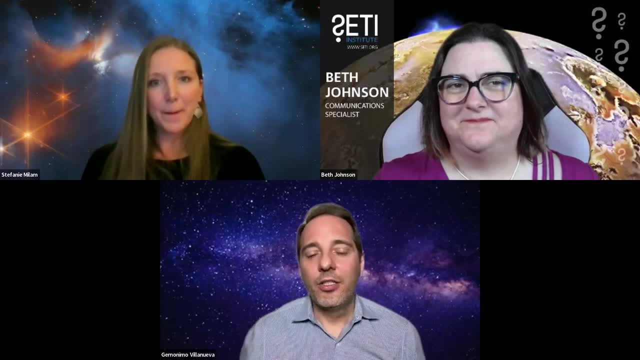 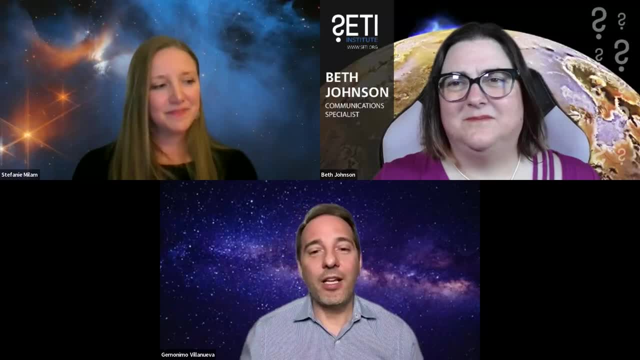 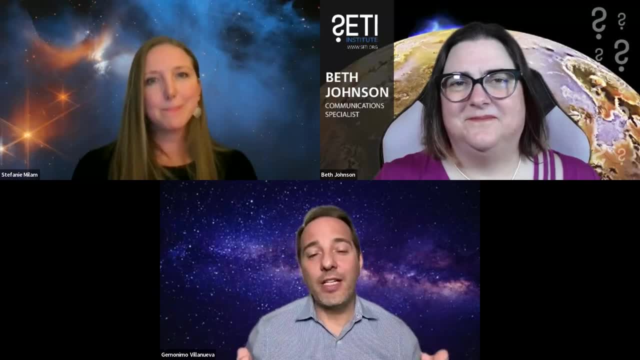 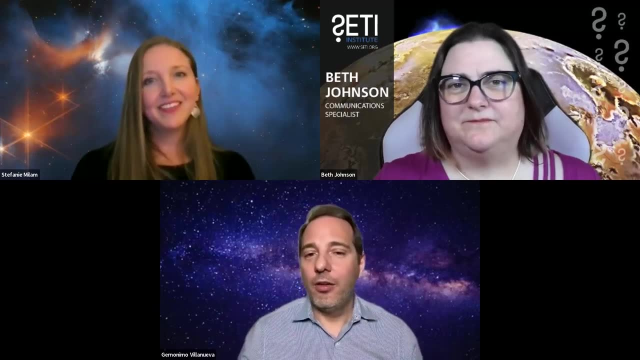 you go And the way you can direct those things is by doing these things. you know, for some of the, if you find a site on Mars that is releasing methane, then I would probably go there and look what some of the findings that we need about methane, even though they're very complex and 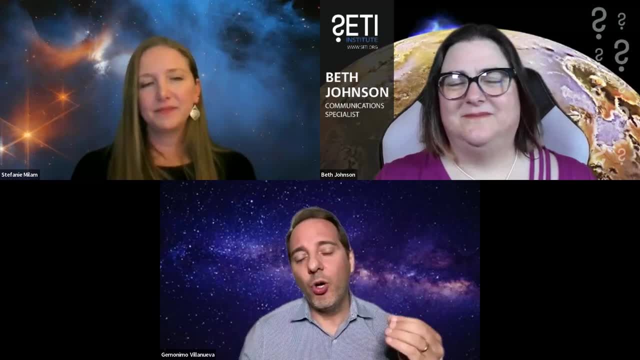 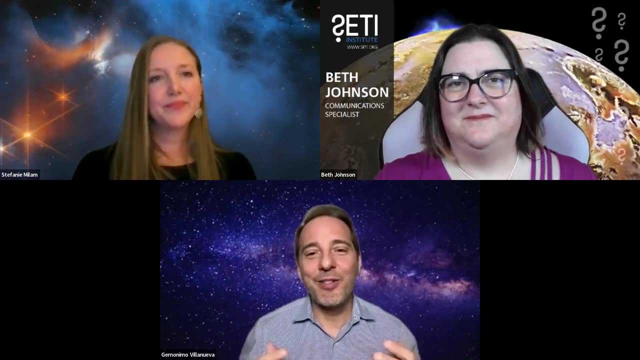 there was a lot of controversy about the system of methane on Mars. that motivate us where to go And you know the pretty clear: a lot of the searches for life on Mars right now are the subsurface And everybody's looking for that aquifer below the surface. So you know the idea of the idea of 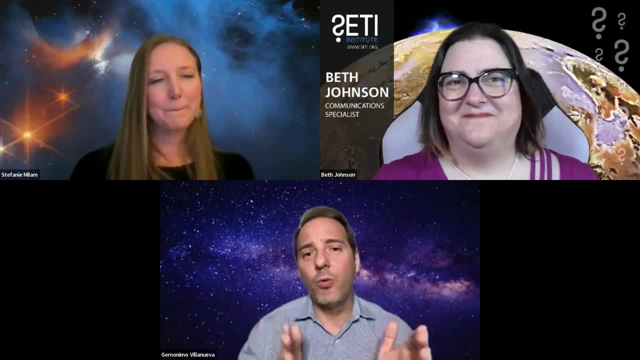 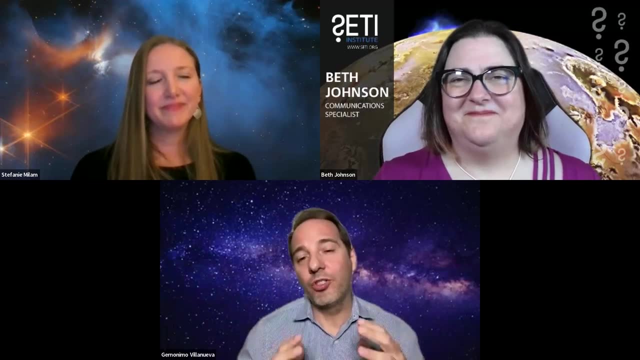 this remote sensing ideas to direct, as Stefan said, honing where are you going to go, instead of going randomly anywhere on the planet. you know where you want to go. this is more chemical diversity, the more chances you're going to see something. So I think you know the idea that. 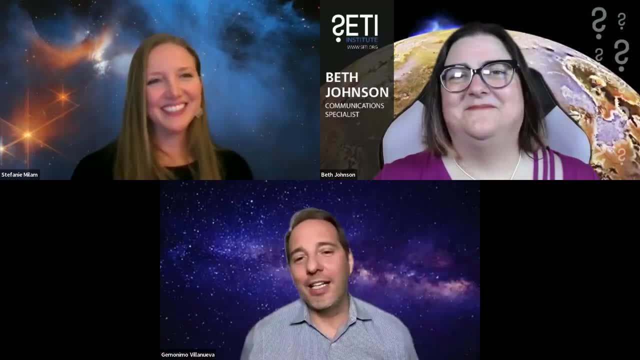 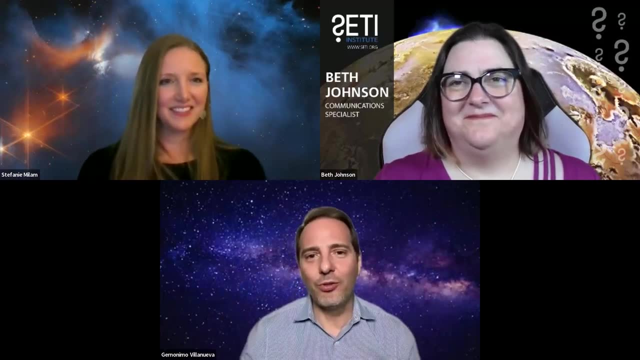 we have this massive telescope up there that we can point and cut, catalog, catalog all these, all these complex molecules. And we're just talking about, you know, methane, CO2, water. tell us about the chemical, but there are other molecules that we also searching. they are within: 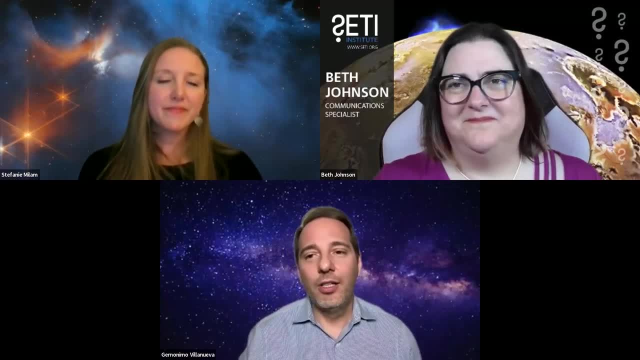 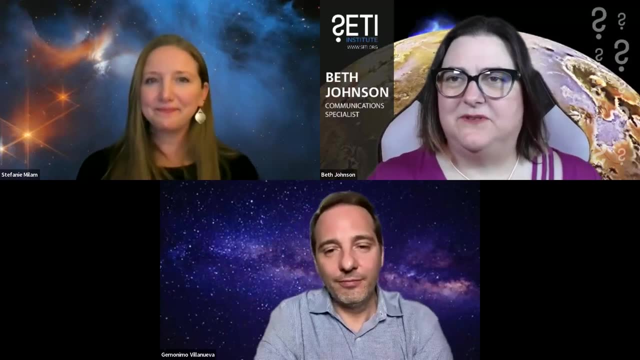 the same band pass And we also searching for them. So the potential for many discoveries are there. I want to get to some of the audience questions, And this one sort of struck me as a good follow up to what you guys were just talking about. you're talking about different molecules, that 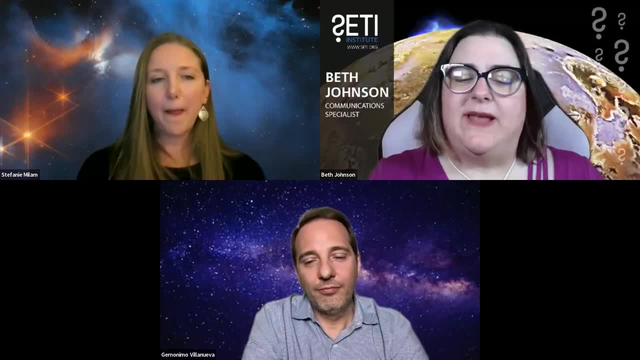 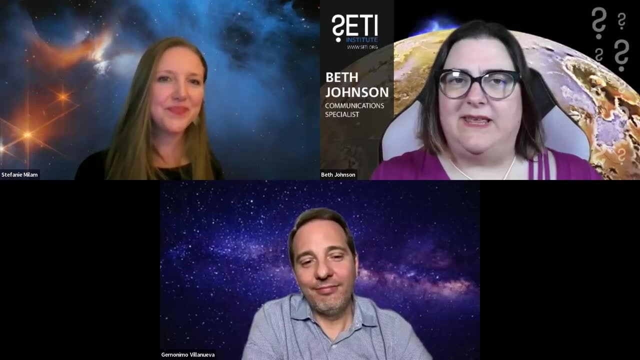 you're looking for. Do you consider any of the any? are there any molecules that you would say are definitive signs of life, Or is it going to have to be sort of a combination of molecules? Are there anything? Is there anything that's unique to life that we would say, ha, that's a smoking gun? Or can we find a more? 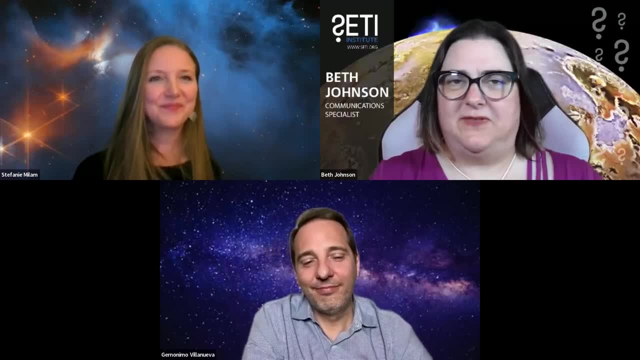 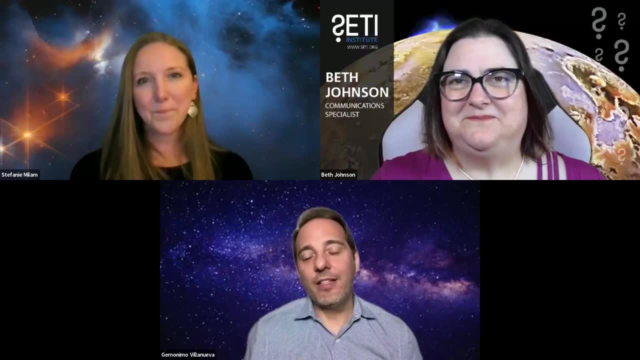 terrestrial, non-biological explanation for most of the things you're looking for. I can say quickly- I mean Stephanie, you can. so I mean the thing I can say is always, as Stephanie was saying, it's about chemical imbalance. You're looking for things, for example: 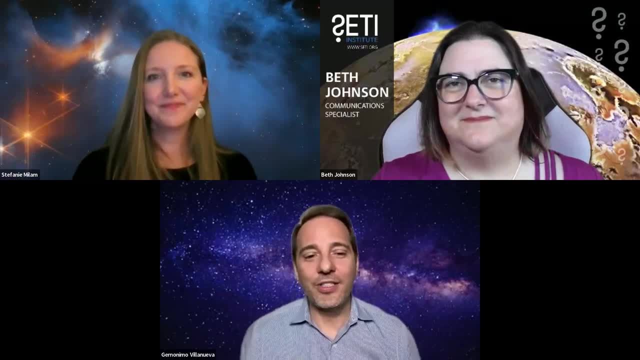 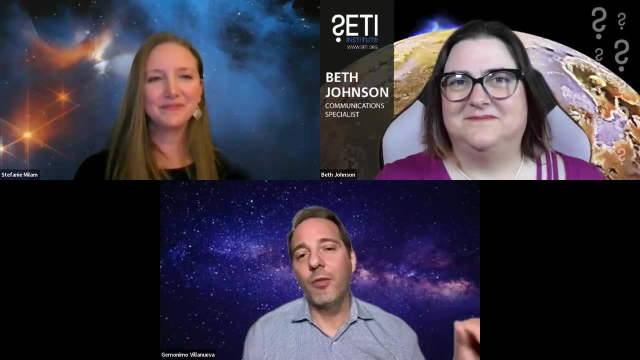 if you find methane in Pluto, you didn't find life on Pluto, it just is there because, primordially, we're given a lot of methane. So the idea of chemical. you're looking for molecules that should not exist And methane should not be on Mars today because it gets destroyed and 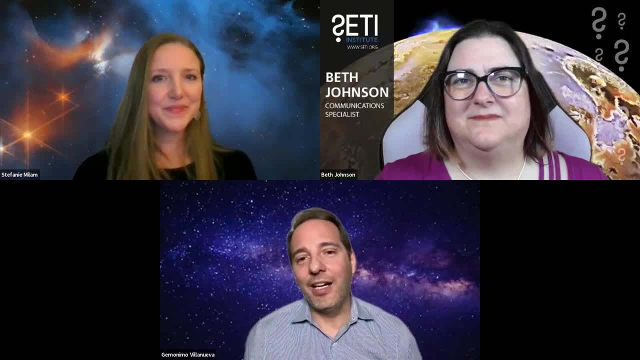 other things. So the idea is to look for molecules which shouldn't be there, but a chemical imbalance, And the idea is to look for chemical diversity. If you ask me, it's very difficult to find smoking gun, molecularly speaking, Actually, even if you send a rover and it's doing mass spec in. 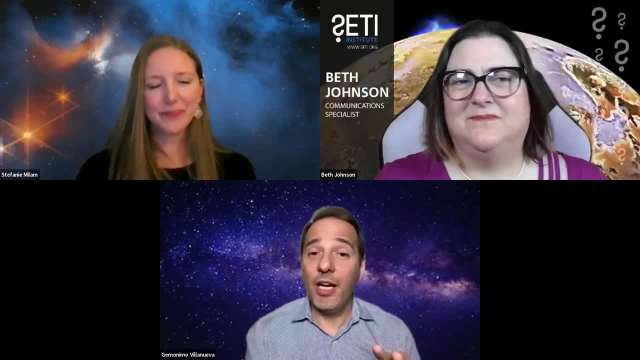 complex molecules like this, you will have a hard time. There are ways, a lot of the work that we can send to Mars that you can find structures. So most of the work, for example, in the world. look, you know, the rovers are looking for chemical complexity, They're looking for patterns on 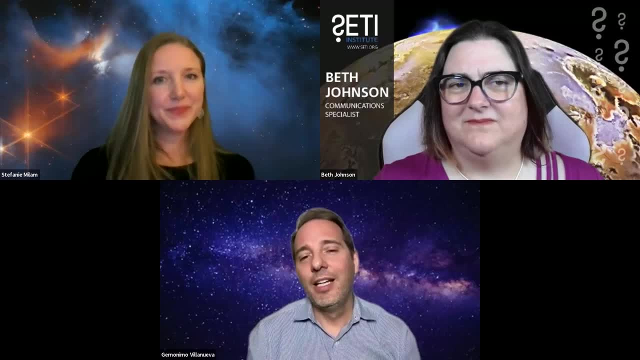 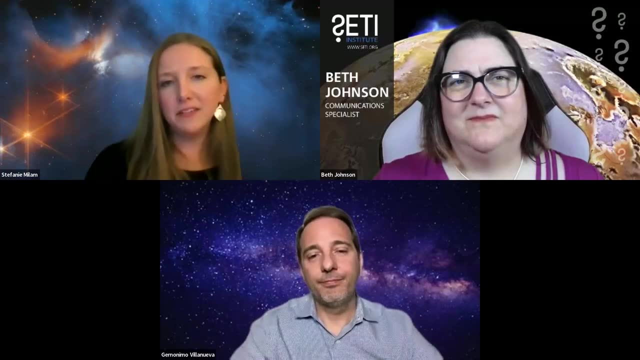 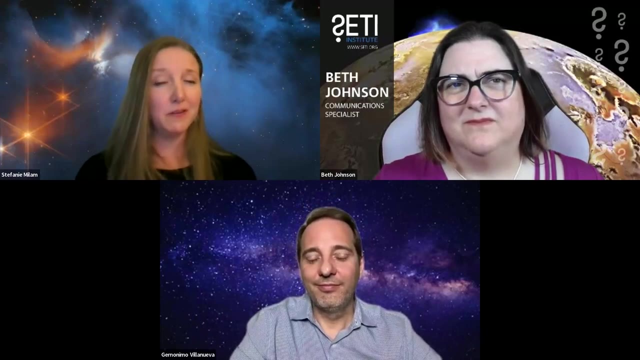 chemical structures which are more perhaps inclined to biology. but it's very difficult to quantify those things with, especially with a telescope, And I'll add just another little aside to this. So we're even trying really hard to find a smoking gun and things like meteorites where we can analyze them in much more sophisticated labs with. 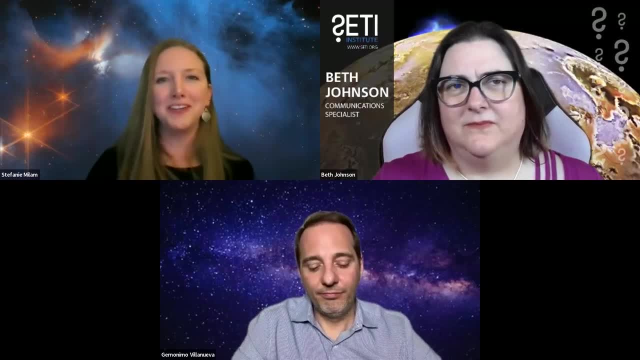 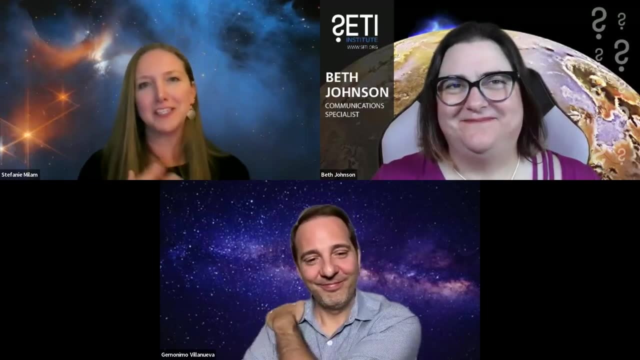 better sensitivity. You know we have instrumentation that are, you know, synchrotrons that are as big as a whole city. that can, you know, study these, these tiny little rocks? and very high precision, And even in those, 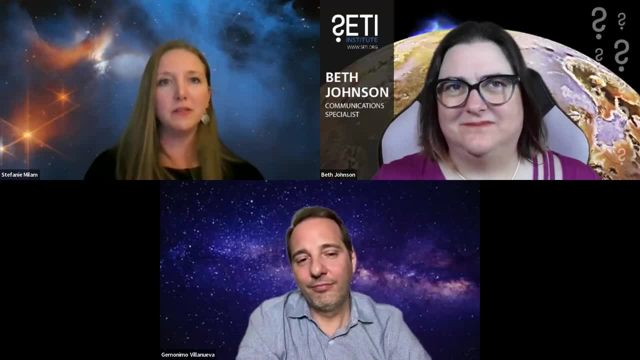 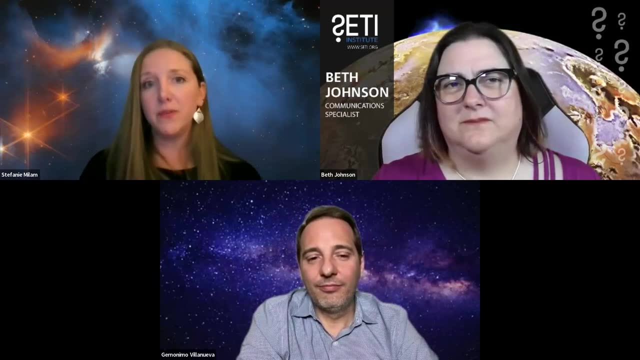 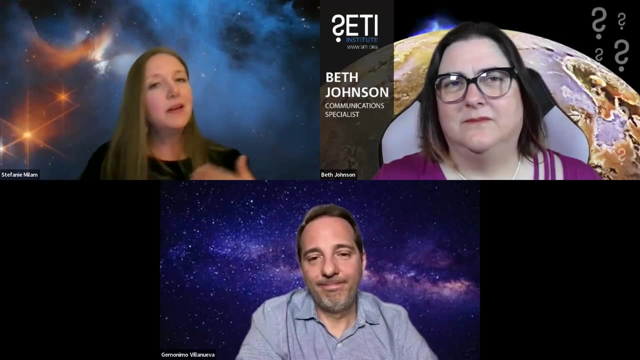 even when we found things like amino acids or nucleobases, the chemistry can always be explained abiotically. A lot of the amino acids that we find in meteorites aren't amino acids that we find in life itself here on Earth. It is provocative, though, because it suggests that maybe that chemistry is actually evolving. 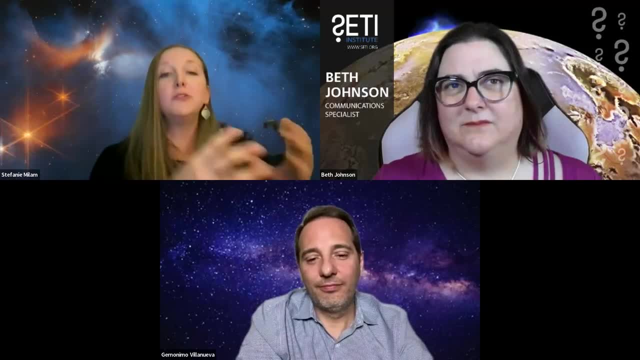 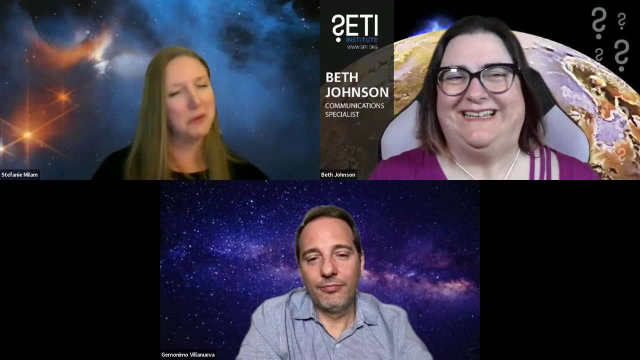 to a state where we have bigger building blocks to initiate something like life on a planetary environment. But the detection of an amino acid in a planet around another star. we're pretty far from that capability right now and probably ever, just because that type of signature, those types of molecules 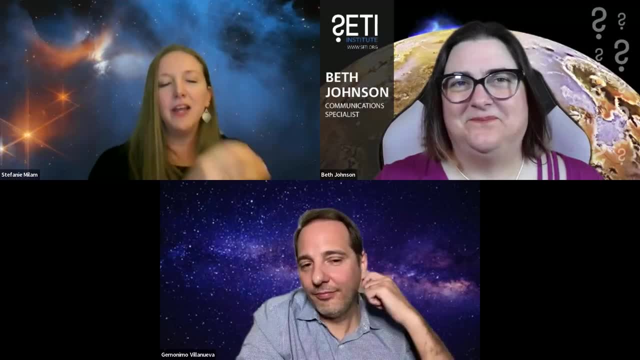 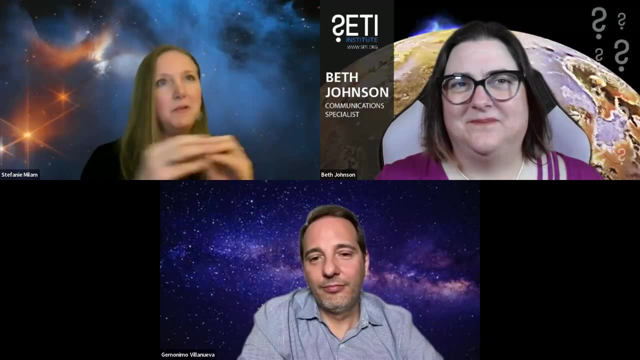 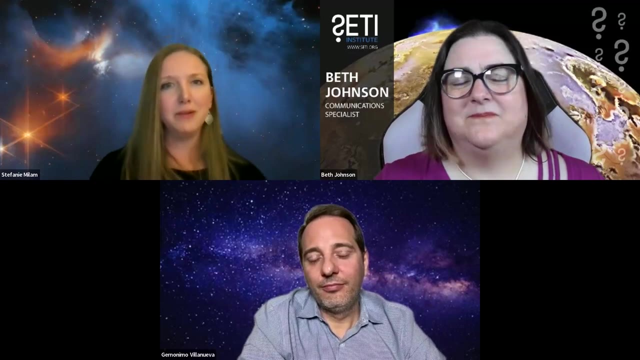 they're so complex, complex. There's so many atoms that are put together to make this big molecule, macromolecule, that finding it with a remote sensing capability is a huge challenge for us. And even in a laboratory. we're talking parts per billion, parts per trillion, types, abundances And what we can. 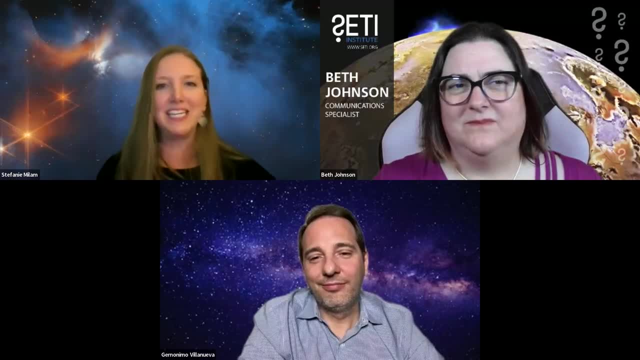 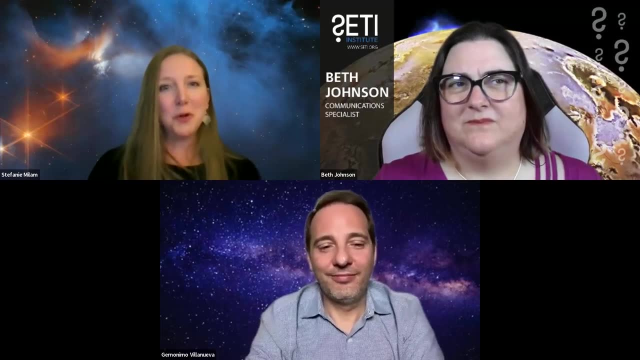 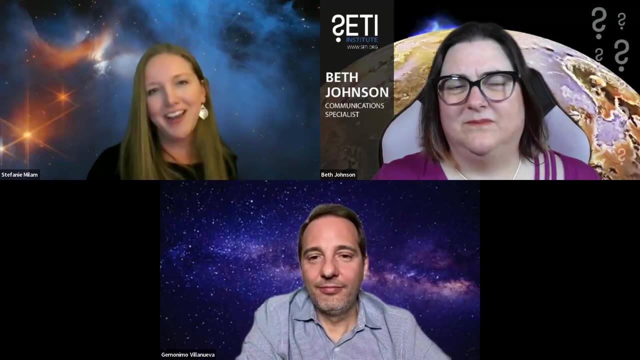 even detect on Mars remotely with JWST, we're nowhere near a part per trillion type of sensitivity for something as simple as methane. So if we start getting more and more complex and have three or four carbon atoms and multiple oxygens and nitrogens, that just makes the detection limit. 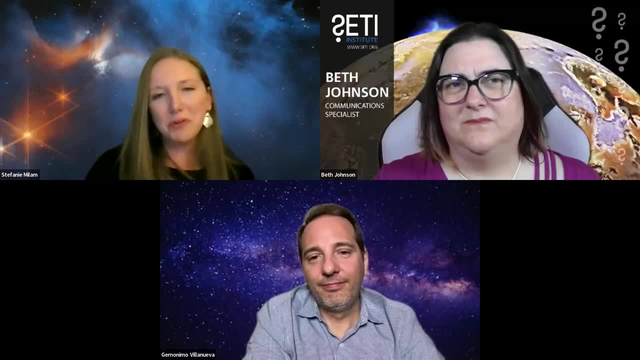 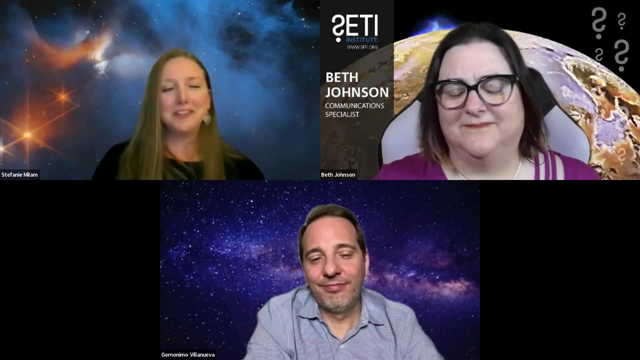 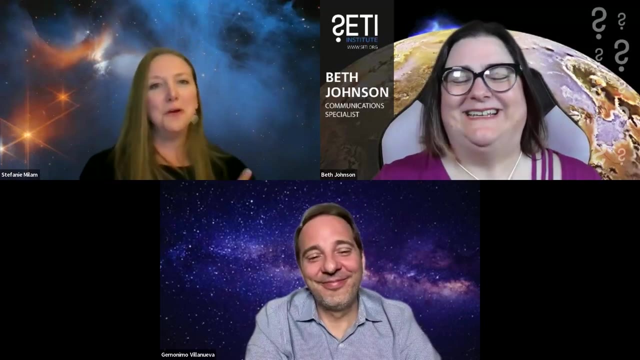 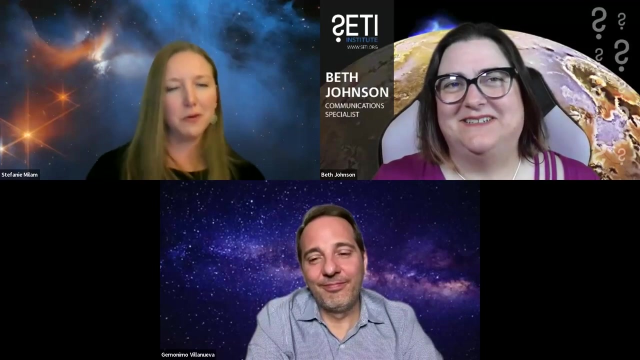 even harder and more complex. So the smoking gun thing is a very hard sell for an astronomer that's doing remote sensing of an object, where we're doing as best we can to detect water in an asteroid. So there's challenges for sure. So I think it's looking for this chemistry. that's a little bit. 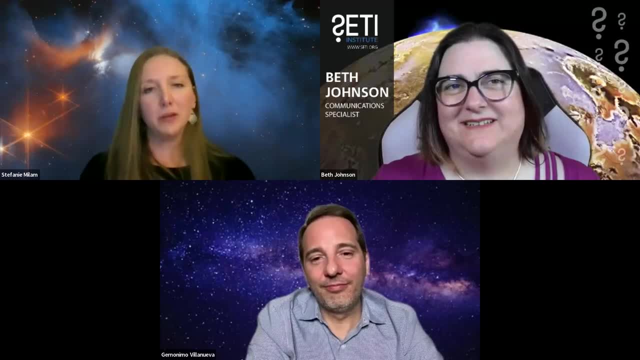 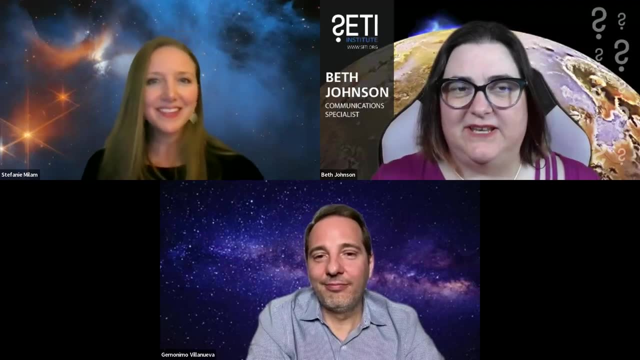 different and trying to figure out why it's different and what could be causing it. So so far we've been talking about looking at our own solar system, but obviously JWST has been looking at exoplanets as well. You mentioned that at the beginning. Have we found any? 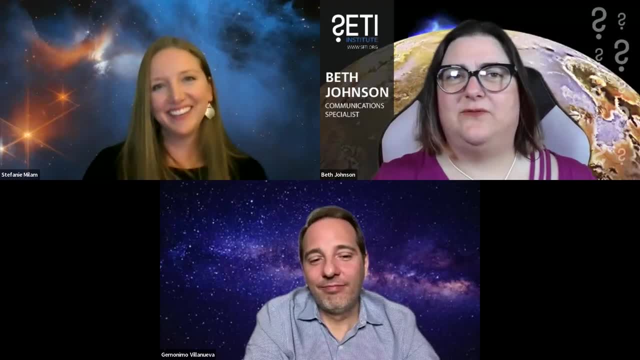 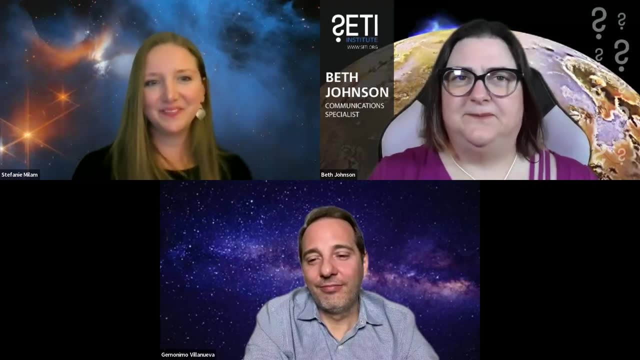 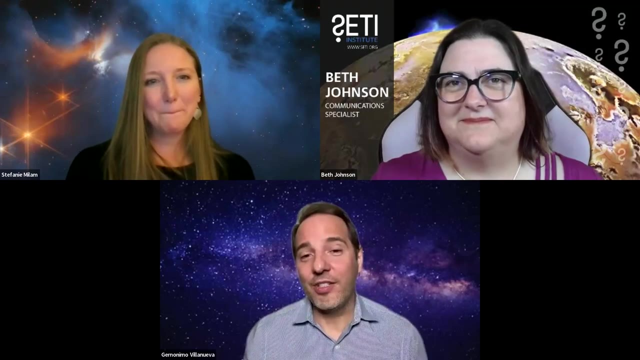 interesting targets so far for JWST as far as exoplanets are concerned. in the future, I can I can mention: yes, so the thing about the most of the plants that we're interested in is definitely showing that there are these plants which are tidily locked. They're very hot because 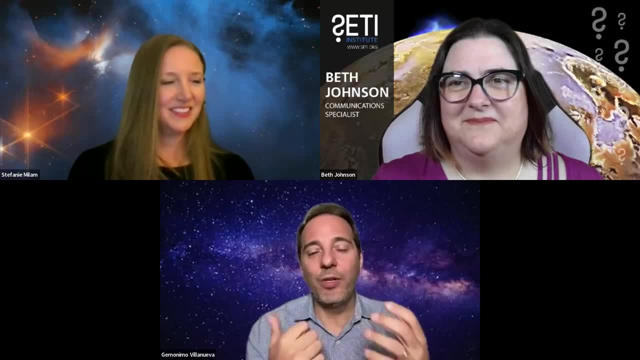 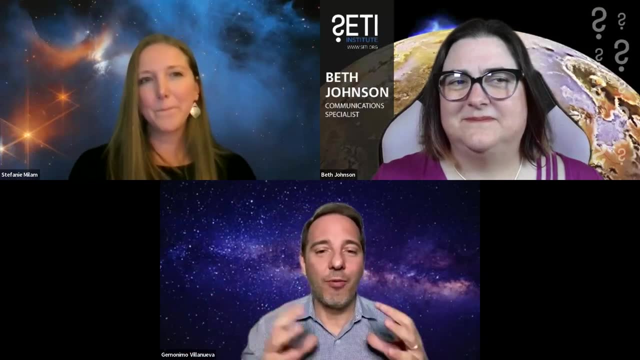 they are the way we detect them. But you know one of the drivers- a lot of the big emphasis is on these terrestrial, like planets or plants which are our size, and they are a bit colder because they are around M dwarf stars, And those plans are more gifted than ever. That's the criticism we've. 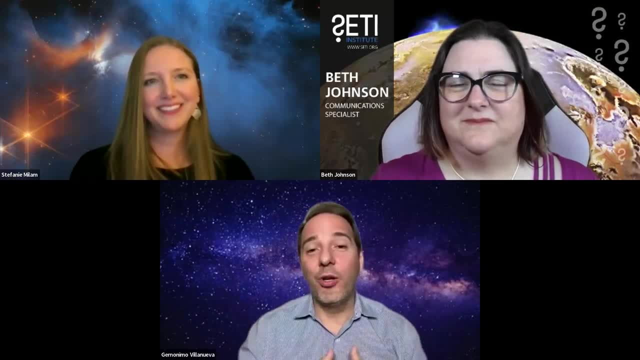 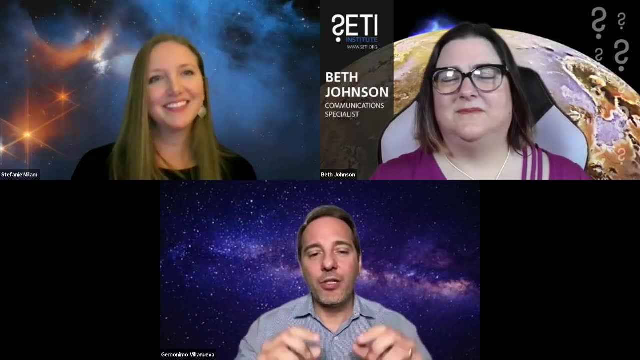 had so far. Yes, so that- Yeah, I'm just gonna let you wrap us up- are more closer to what we think about habitability. so a lot of the emphasis that we're trying to do is to measure them. they are really challenging for, even for gens web, because the atmospheres 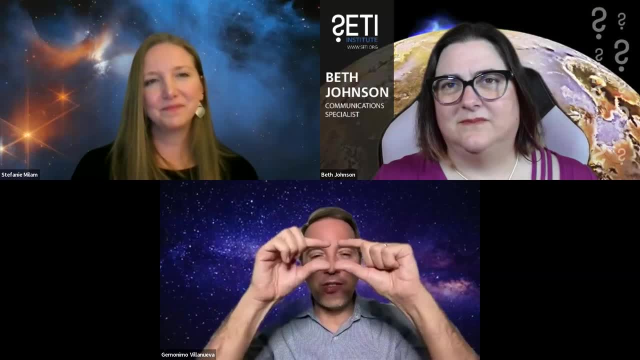 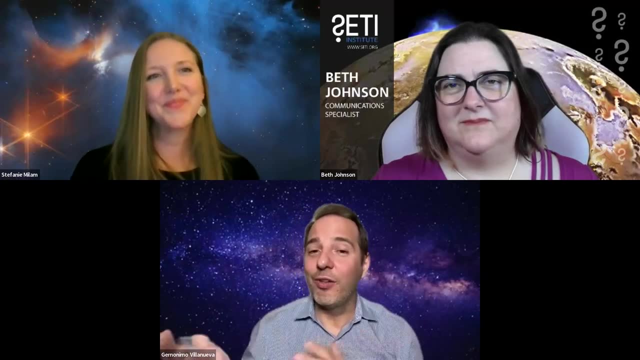 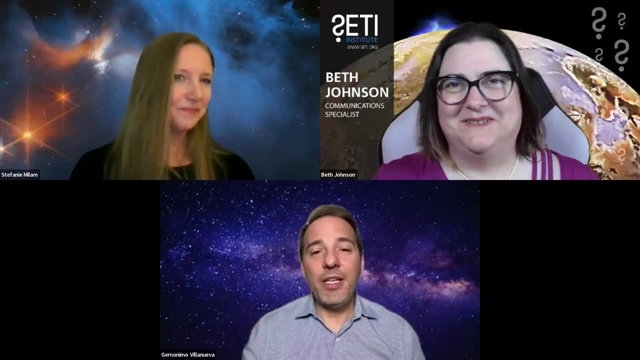 are very compact. so when you're looking at transistors, spectroscopy, those trends have become very compact, transits and become very difficult. yet there was this detection of co2 and people are looking for other complex, other complex, other molecules like methane and water and so on. so there may be a chance that we may be able to determine complex molecules. but if you ask 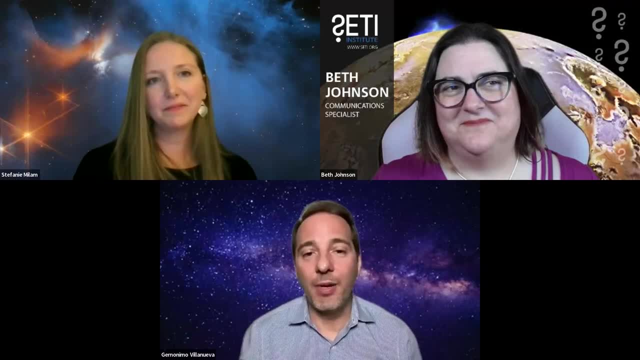 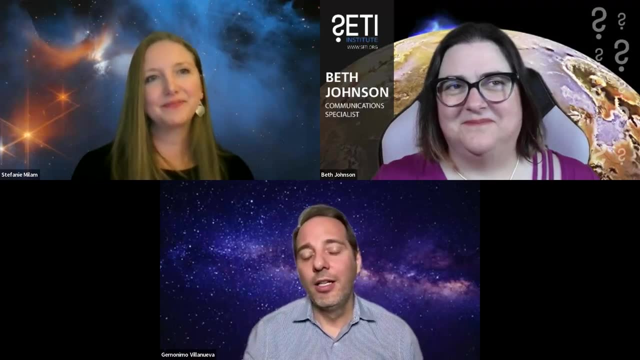 me. if you can detect a lot of chemical diversity in a planet- and we are lucky to do that- that definitely makes a lot of interesting studies about chemical imbalances, as we've been talking about the ideas to see why those imbalances are happening. it's like oxygen in our planet. 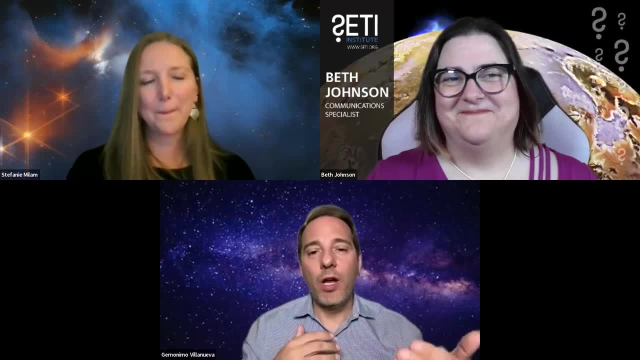 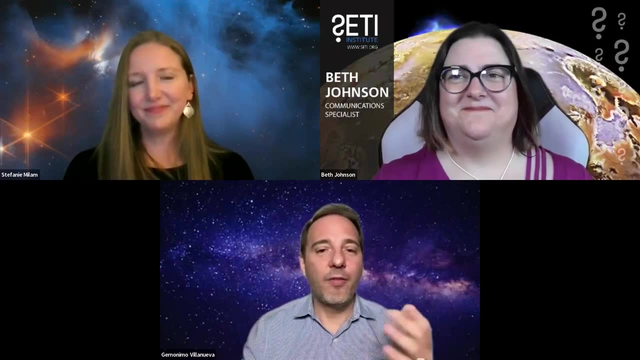 is. it shouldn't be here or in this proportion with ozone. so when you find him, when you find chemical desiccators of that form are diagnostic of maybe something happening, but again, as stephanie was mentioning their geological process, so we call them false positives and it's. 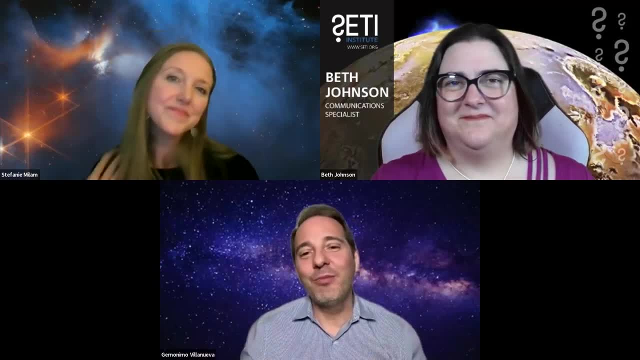 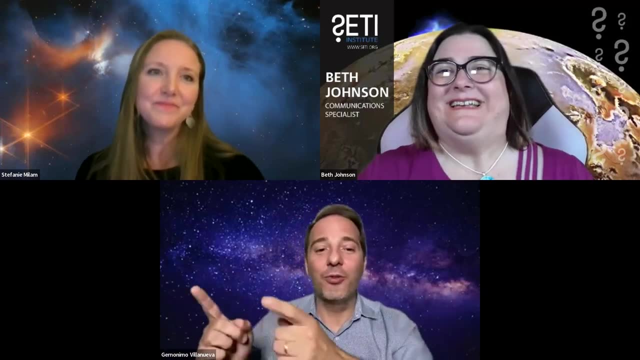 part of the big research. but if you ask me, i will keep searching. you know, the more plants we find, the more we understand the chemical diversity, the better. we can just say, okay, if i have to go to a planet, at least i go to those that they have some chemical diversity. 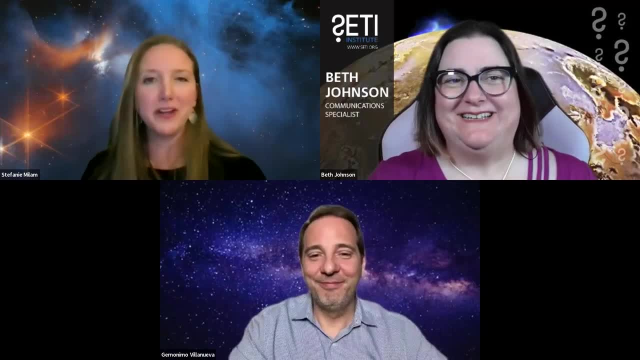 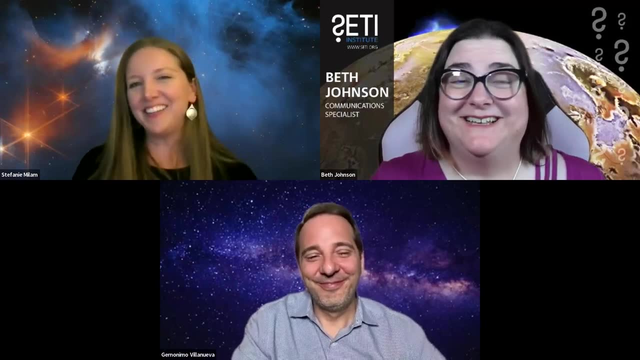 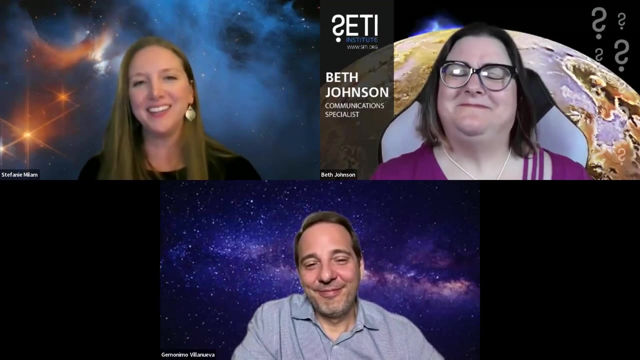 um, oh, go ahead, stephanie. oh, i was just going to say my favorite exoplanet observation to date has been the one with absolutely no molecular signature. uh, it's arguably the most uh flat spectrum anybody's ever observed towards the planet. um, and there's a lot of humor, that goes. 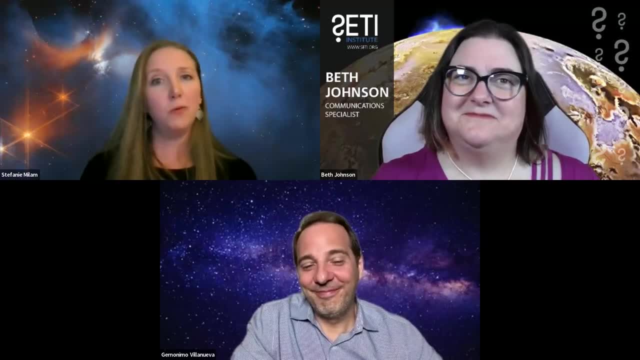 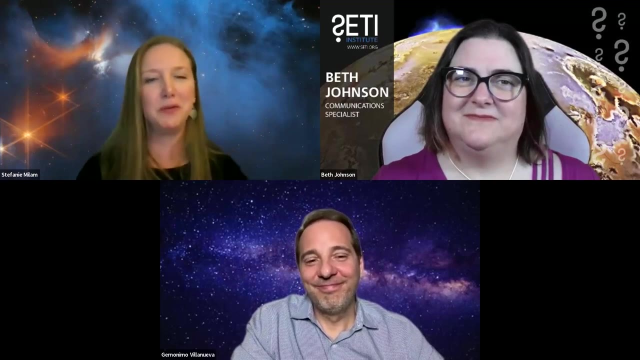 around the community about it, but, um, they detected nothing. no water, no methane, no carbon monoxide, no carbon dioxide, um, at a very sensitive level, and this is one of these, uh, terrestrial planets that's in the habitable zone. um, but yeah, it's a. it's a pretty dead planet, it's probably what? what mars? 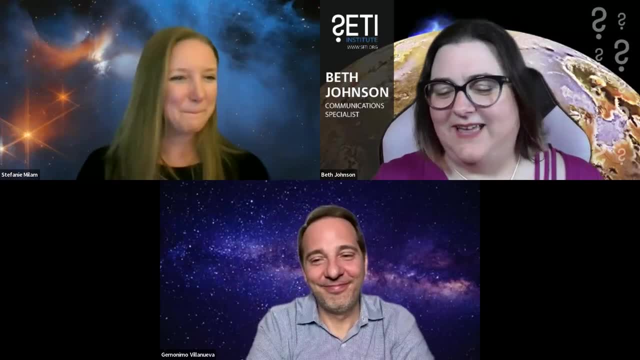 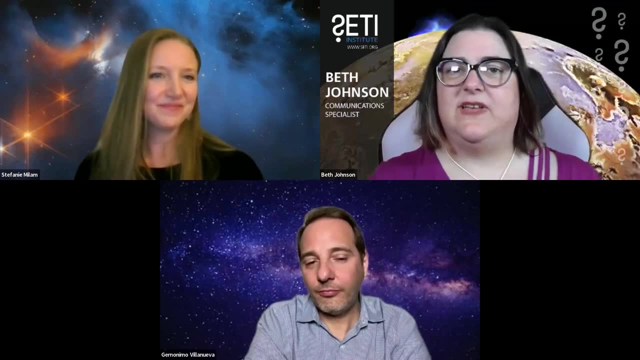 would look like for us. wow, uh, that brings me to sort of another audience question here. um, you mentioned that you you observed this uh exoplanet at a very sensitive level when you talk about jdst. how sensitive, how accurate are we talking about these observations? what sort of 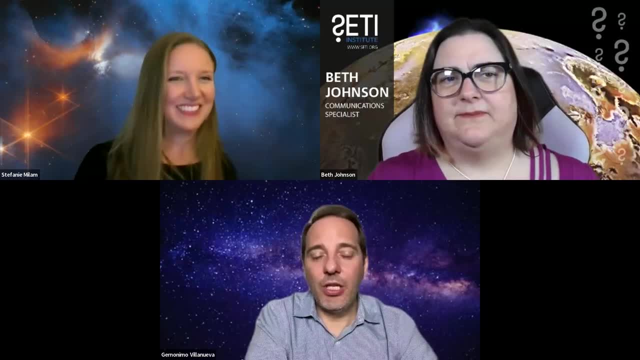 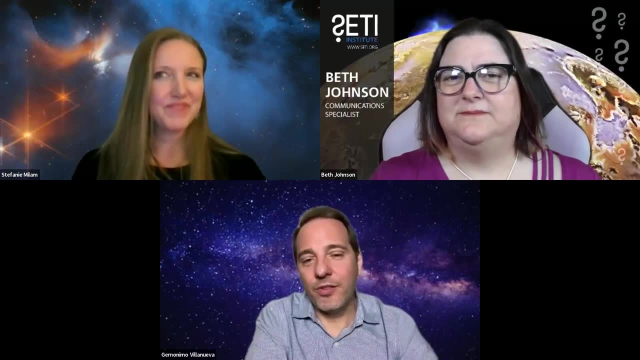 level are we getting to here? these are, these are: you know, these are incredibly precise measurements. this is what we call parts per million, so you actually can detect sunspots on the stars and you know, in some of the other work- actually- stephan was mentioning that- what we, we, are. 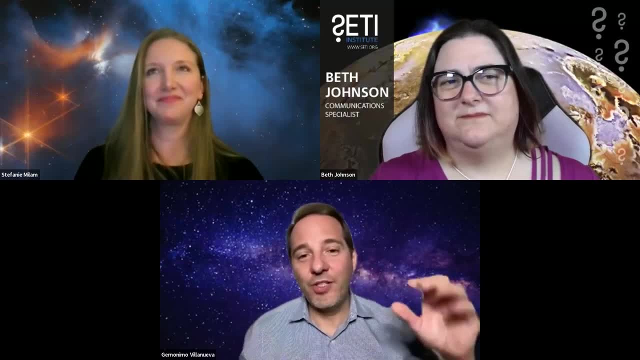 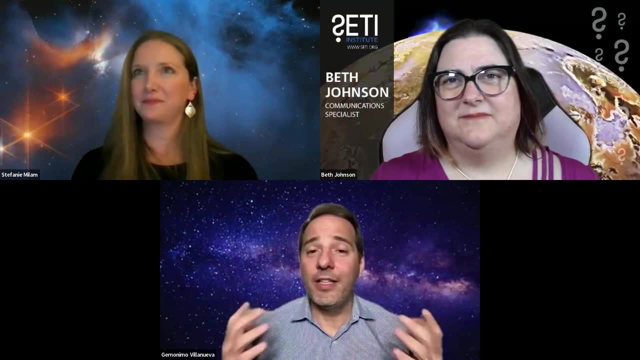 reaching the moment that we are already. basically, if we we see in sunspots and the stars, we are getting some sun storms on the star than on the planet itself. so i think it's incredibly precise the level of thing- and i think this is the beautiful thing about being in space- you can 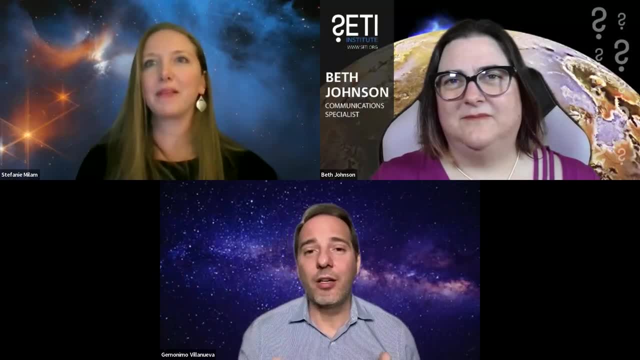 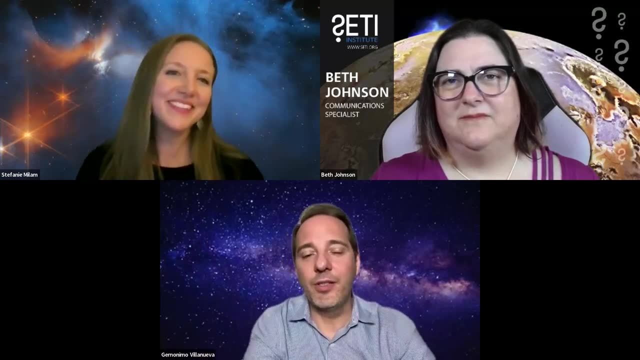 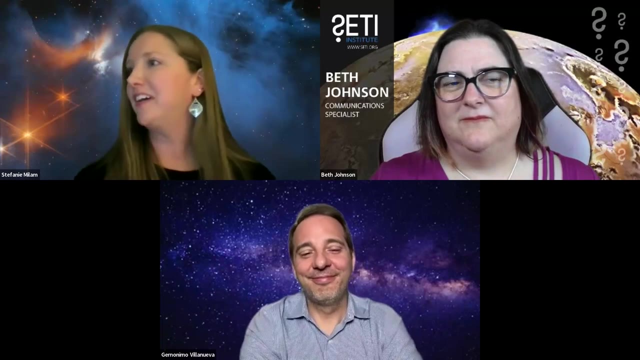 have a massive telescope on ground, but all the elements of being in ground makes the measurements very difficult. being in space with such a big telescope- cryocool, it's what is what allows this. incredible sensitivities of parts per million? yeah, and i i will show one of my favorite examples: um. 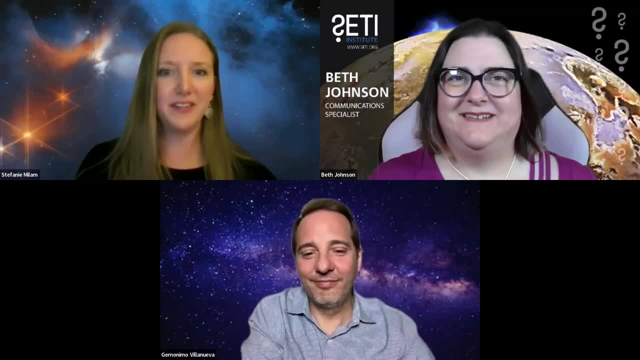 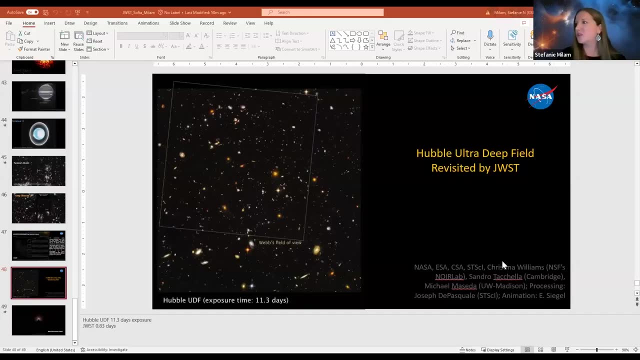 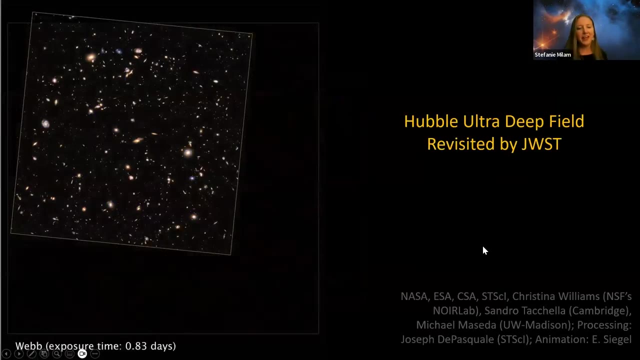 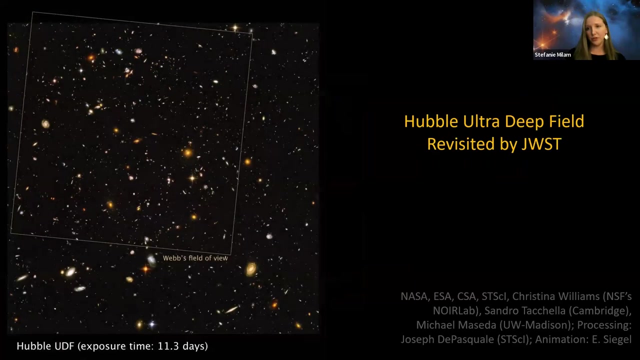 so this is a fantastic one. let's see share. i'm sorry i have to share first. so um the hubble telescope uh was known for doing uh the ultra deep field, and um hubble uh spent a lot of time. the director spent his own time that he had to allocate as he wished. 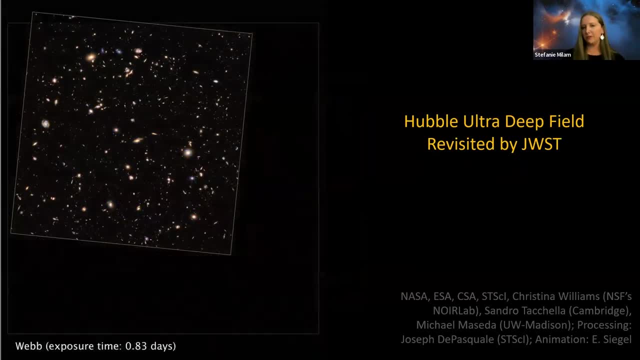 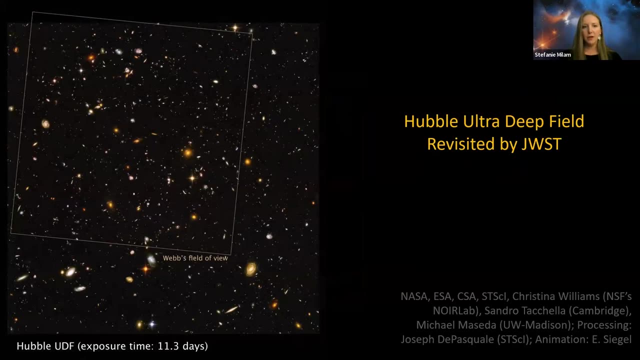 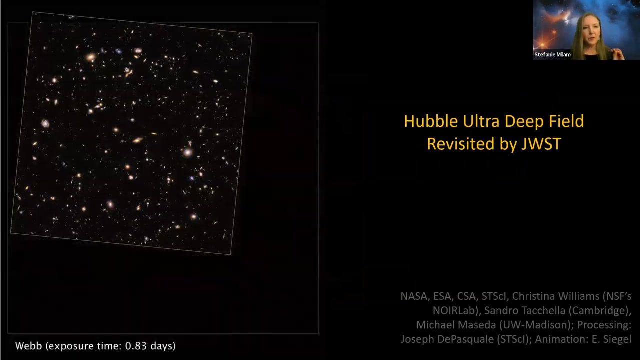 to just sit and stare at blank sky for hundreds of hours and um one of which is known as the hubble ultra deep field, and so the total time accumulated was about 11.3 days worth of time staring at one spot in the sky, and we took a glimpse at it with the james webb space telescope. 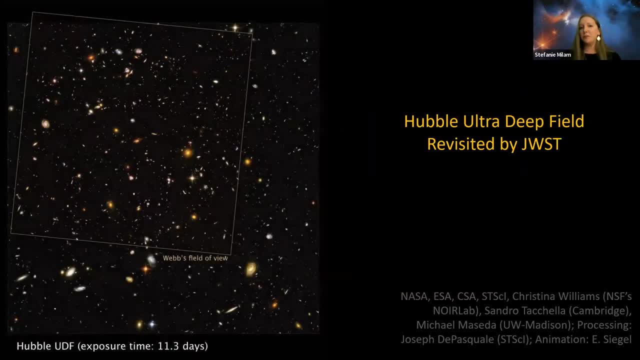 for um, not even a full day, and they actually operated at the same wavelength. uh, hubble ultra deep field had was at the near infrared wavelengths, so hubble did go a little bit overlap with jwst um and you can already even see in the blinking of this image the 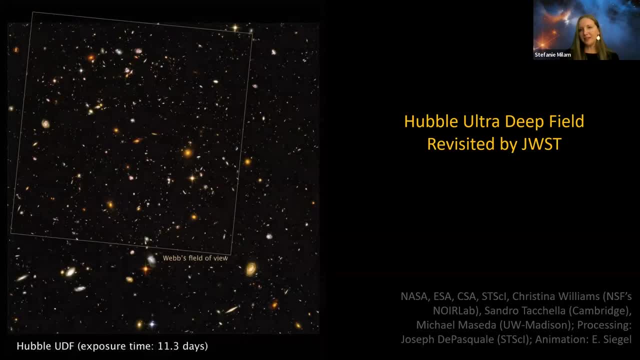 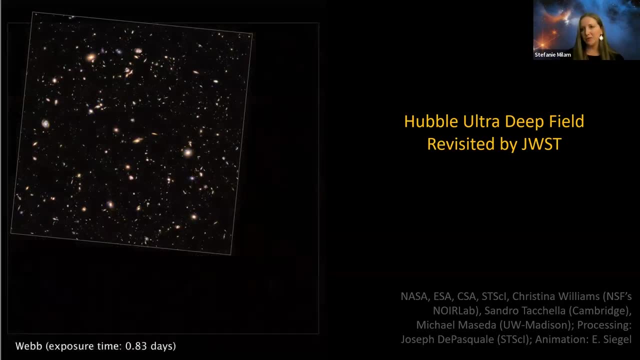 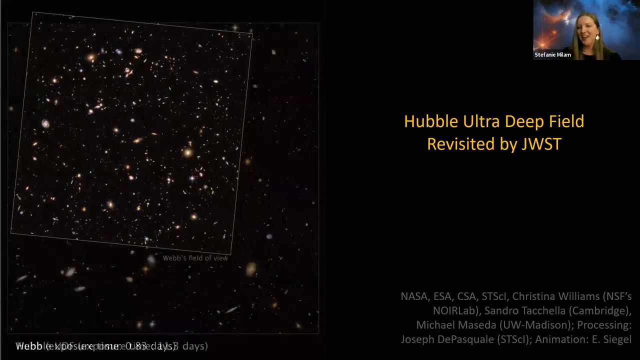 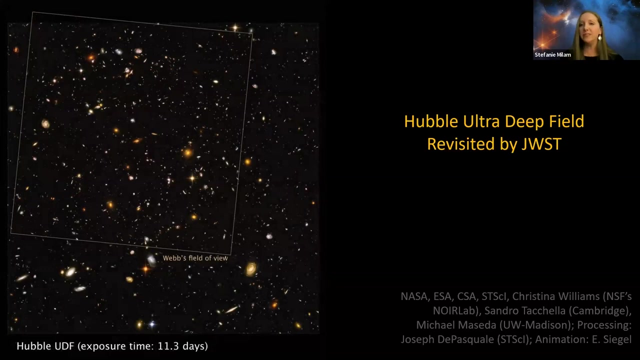 capability of jwst and um a tenth of the time, basically just to get something even better, even more spectacular, even deeper than what the hubble space telescope could do at these wavelengths. so we are incredibly sensitive and it's only revealing itself. every single day, we get to see new images, new deep fields, new discoveries being made, even in our own solar system. 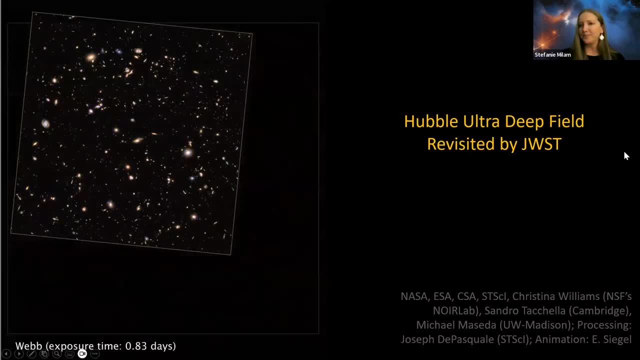 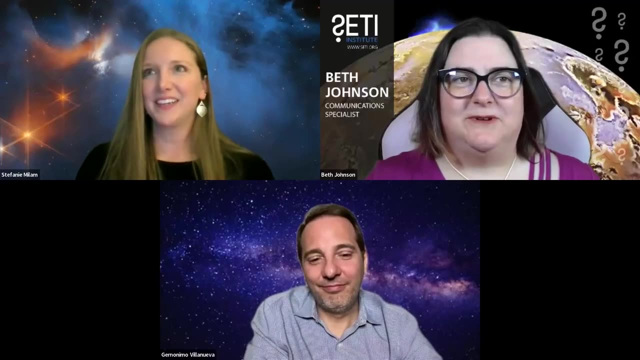 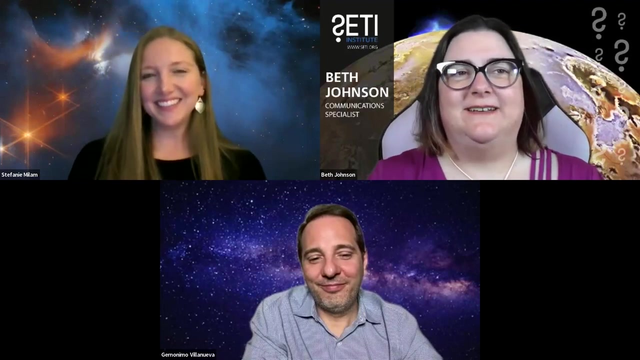 with capability that we've never had before. that's, that's amazing, and laying it out right there is is really fascinating. um, i'm going to take one last audience question here, um, kind of because it was going along with where i was going to go. um, they said: i love this. i know jwst, science is exciting, but what's next? 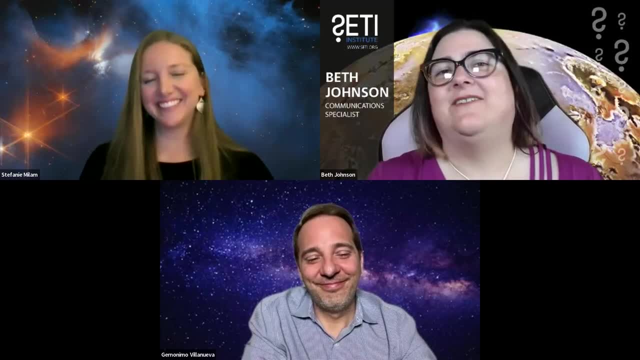 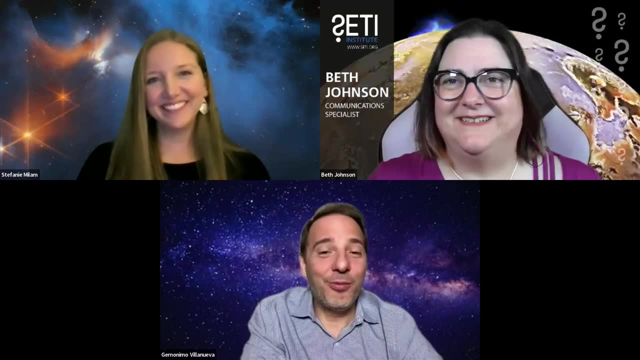 what is the next type of telescope we should plan for to get us to the next level of astrobiology research? i can go, yeah. so we are working, actually with stephanie on on different projects. so right now we're working. we have we have roman. this is the next frontier, this is already. 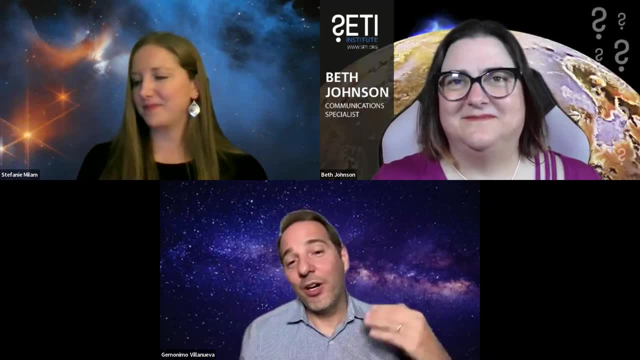 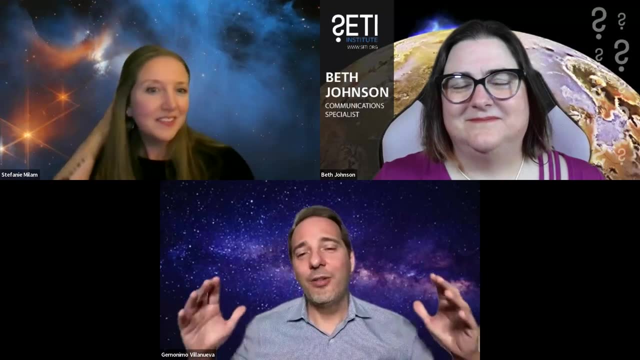 happening and we have a lot of exciting things with roman, but i think we are also thinking about the future beyond roman and that. then we have things that you know. we have things about things like like a, like a lube or havex, or have the warship. so there's a huge observatories, a lot. 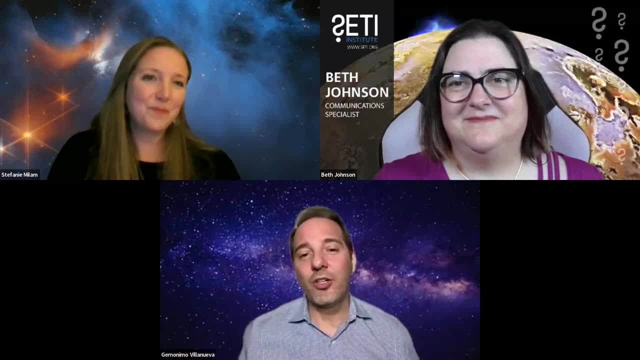 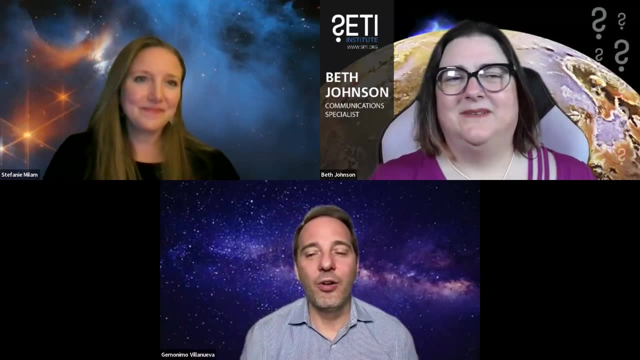 of collecting area. we're also thinking about an infrared like origins telescope that it can do the thing we're talking about, the infrared, but even even a broader wavelength and collecting area. so yeah, so there is a lot of things that we're thinking is all about, you know, spectral. 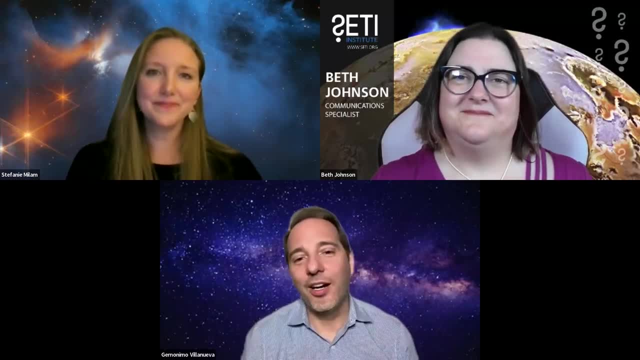 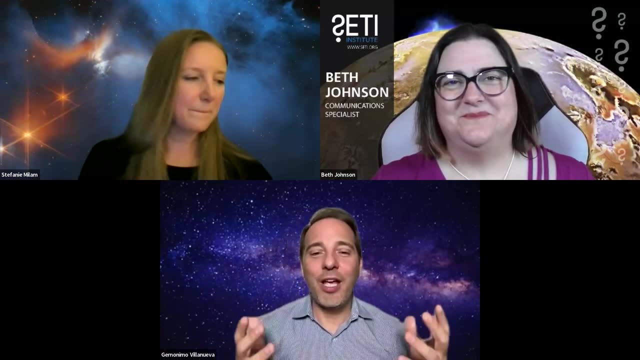 instrumentation. most of the things you hear today are our spectroscopy. so we are. we are biased to spectroscopy. we think all these chemical tracers are best land with the best instrumentation. so the infrared for us is very powerful. the higher resolution and the high collecting area are the 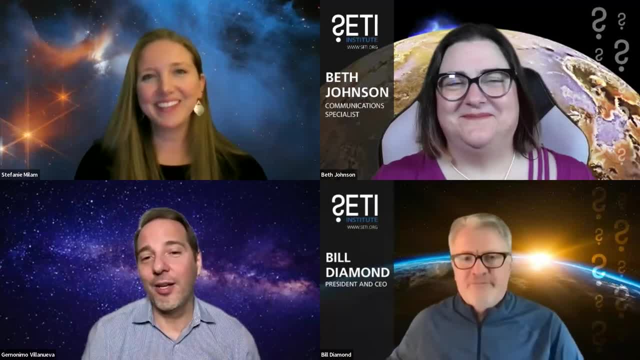 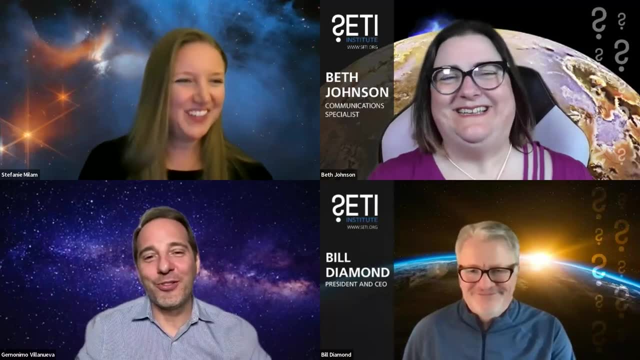 things that we really need to make these measurements happen, and i think we are going to be working for at least probably till we are retired from science and the future telescopes that i think they're probably going to be in 2040 or so. it's job security, that's all. 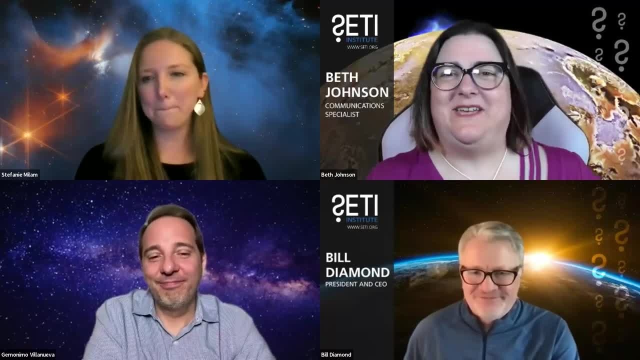 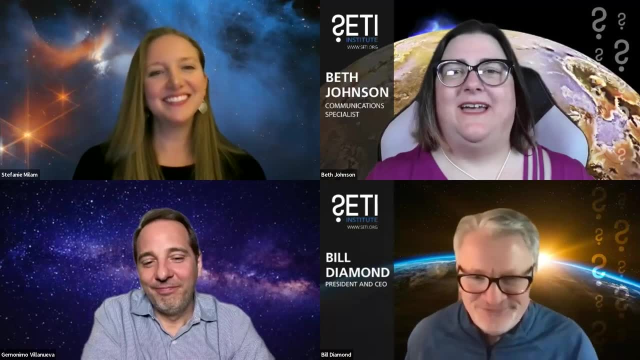 all right. well, i have, i do. i will have one last question, but i'm going to let bill take over for just a few moments here. no, go ahead and ask your. ask your last question, bet. ask my last question. oh, of course you do. uh, here we go um. all right, so what does, in your opinion, this science? 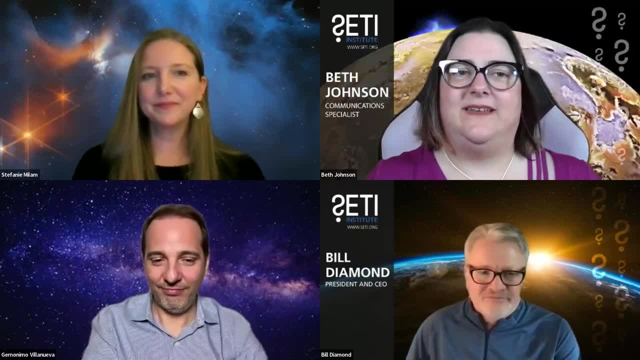 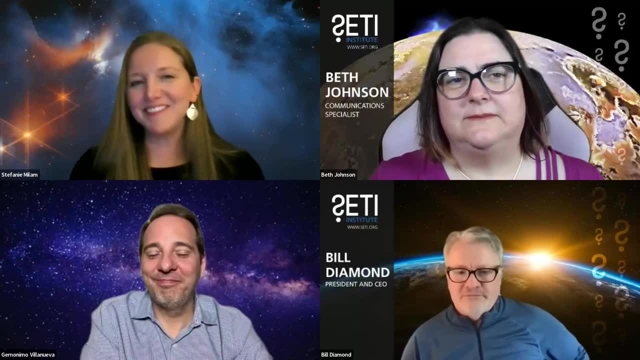 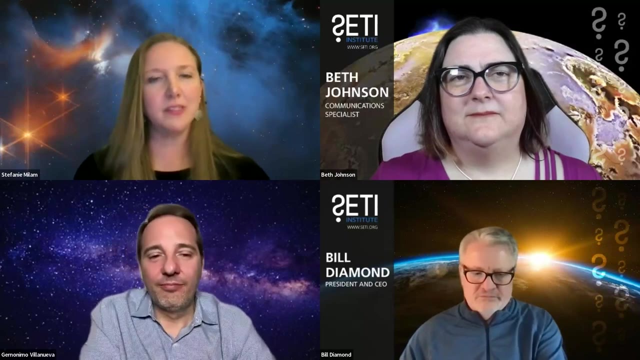 mean to you, to science overall and and to humanity at the end of the day the day. Well, I'll start, I guess. So I think what we ultimately are doing is we're in this realm of you know, the big questions that humanity has always asked, you know, are we alone? How did 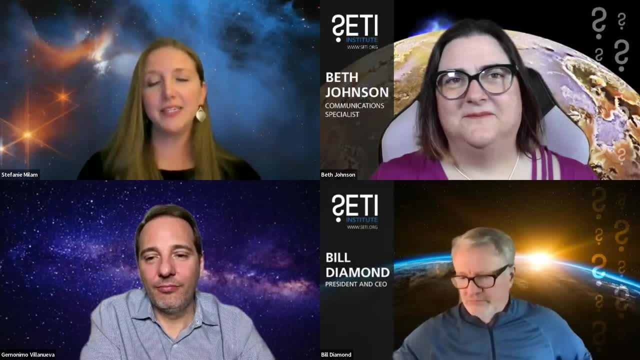 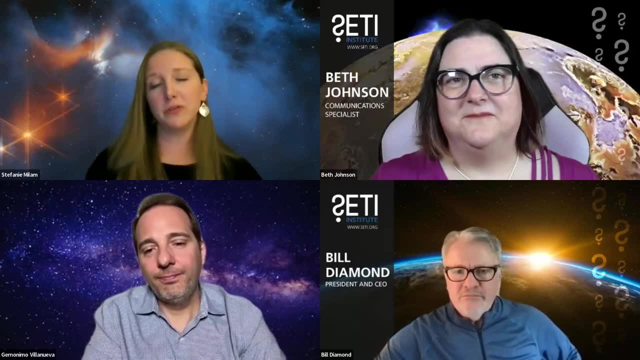 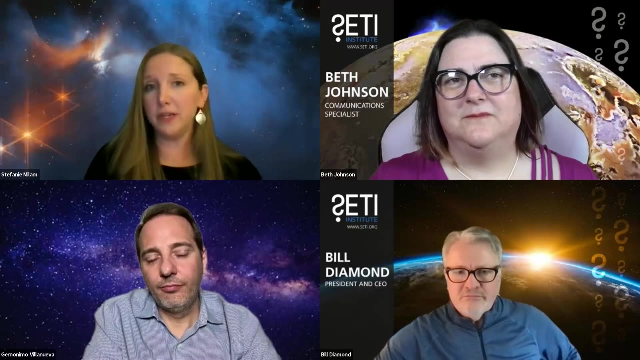 we get here, What's out there, And by searching in a very systematic manner, understanding our local environment, so earth itself how it's evolved, to planets that have sort of resembled history of earth- so Venus and or Mars- and understanding how they've evolved with time. 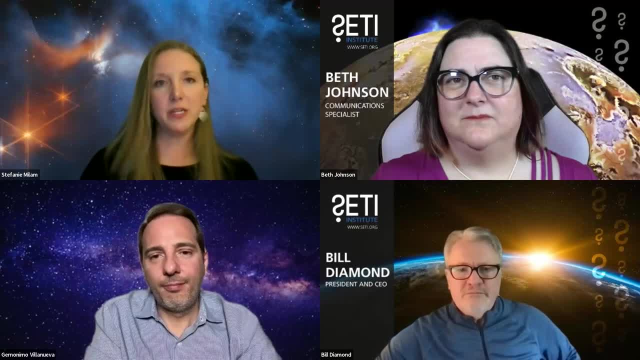 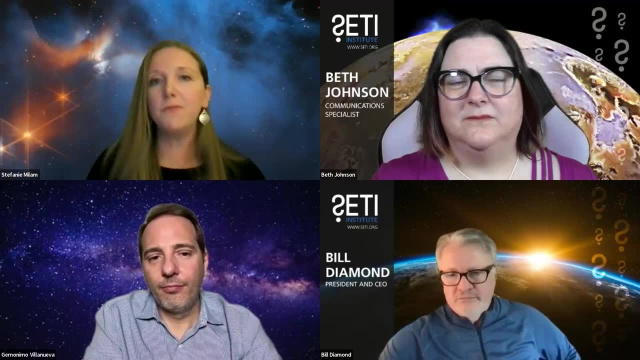 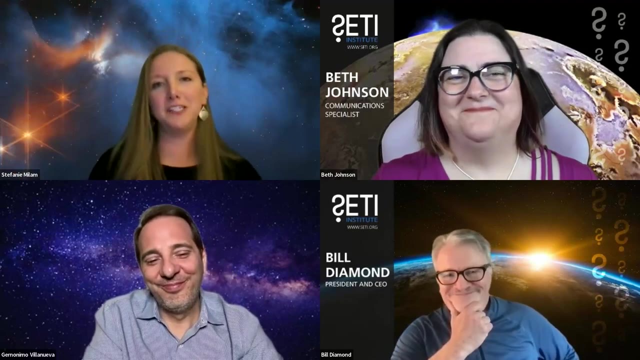 even since the formation of the solar system, understanding what the composition of the material that created the planets in our solar system, how that formed, how that evolved, how it gets processed. Every time a comet comes around the sun, you know it's getting a sunburn, it's getting a little bit cooked. So when we're actually 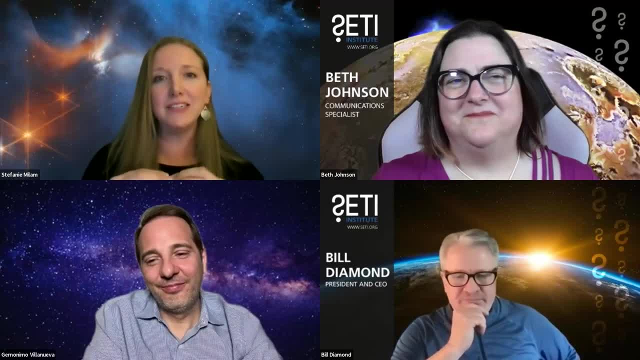 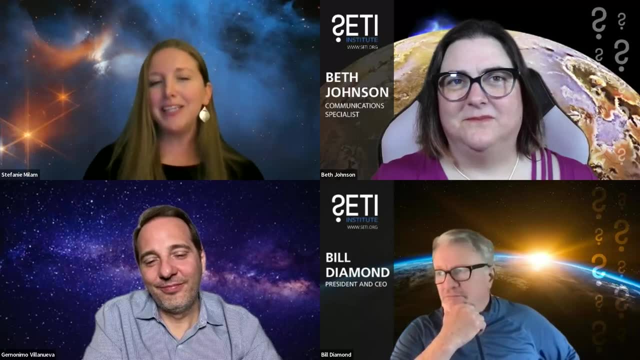 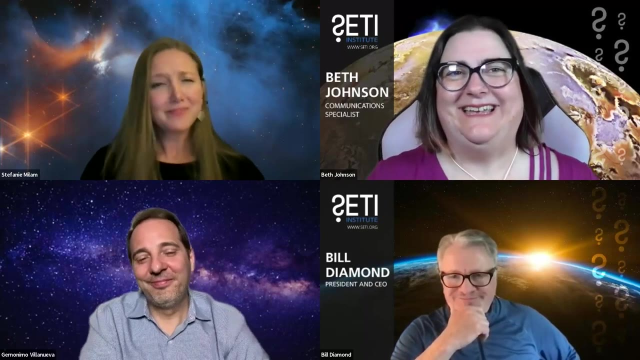 observing comets. are we seeing that true, pristine, you know fossil material from when the solar system formed? Or is it a little bit cooked? Is it a steak, a leftover steak in the back of the freezer that's already been on the grill? Or, you know, is it the fresh cow? And then we can compare. 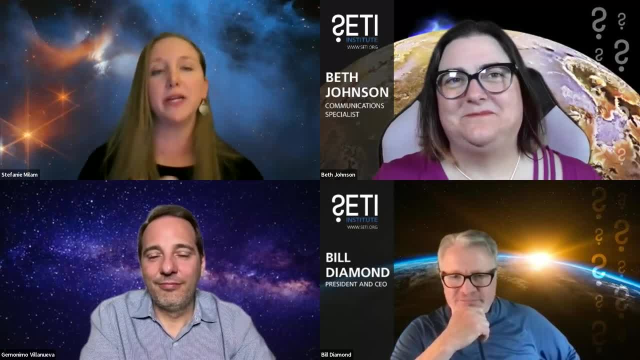 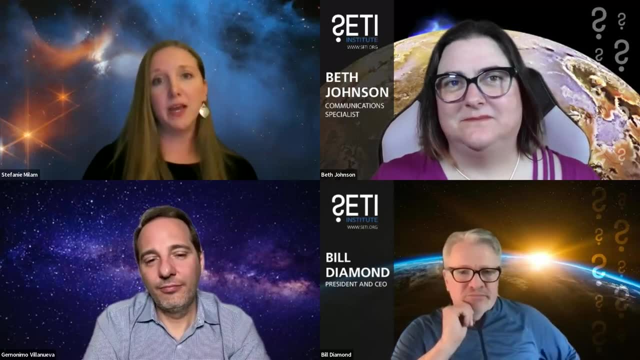 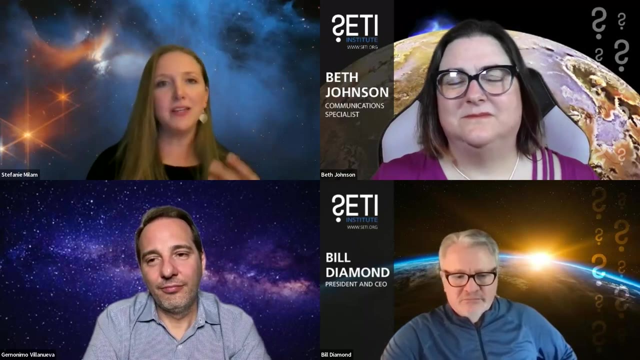 that and understand sort of that evolutionary process in general by looking at other systems, planetary systems that are forming, studying planets and other planetary systems, studying star formation and the chemistry that's happening in that star formation and evolution. As a star dies, what does that mean? Does it annihilate all of the planets that were around that star? and 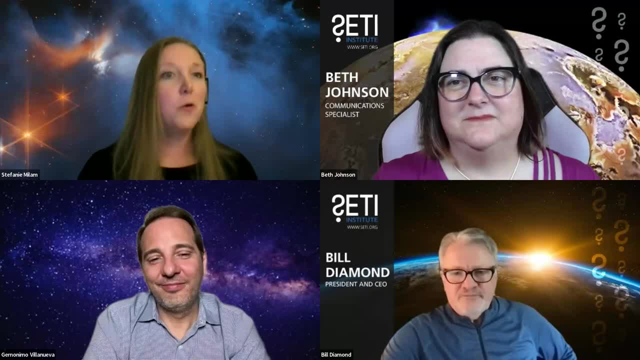 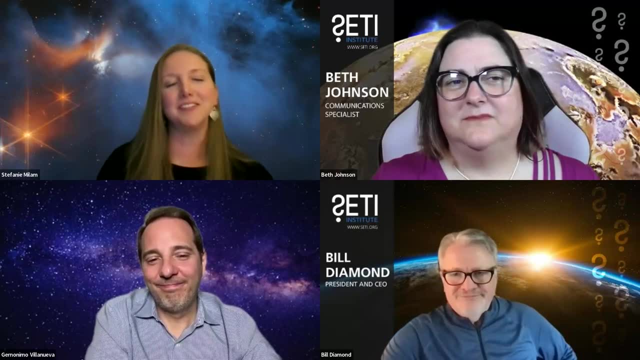 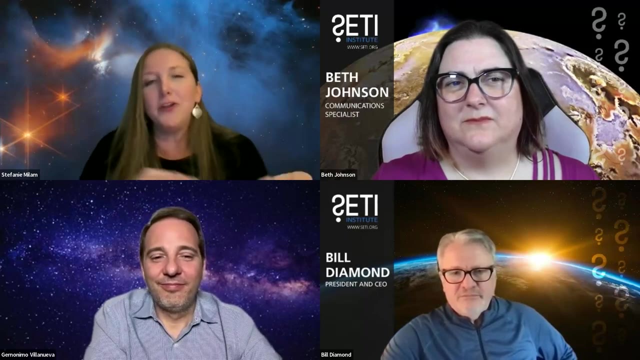 completely disintegrate them into nothing but atoms and dust? Or is there some molecular remnant that actually survives and gets carried on to the next new star forming region or new planetary system? So the discovery, the discovery, space is out there. and and all of this is, you know, I'm a chemist. So, following the 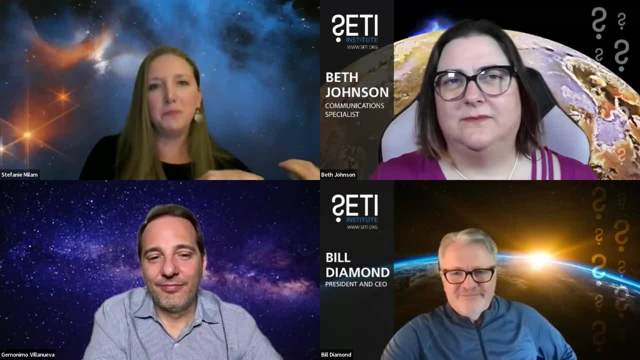 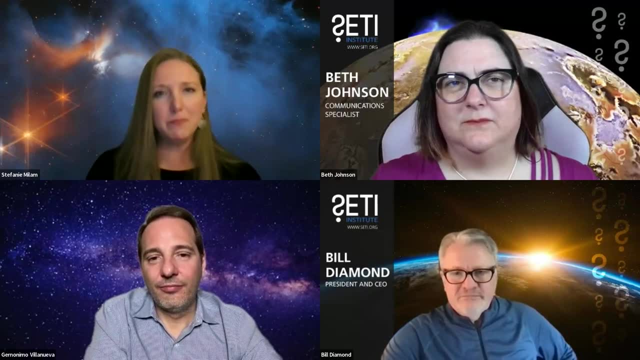 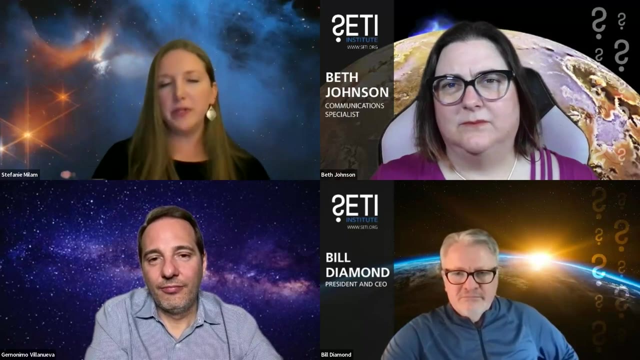 chemistry is sort of what I do, But it also means that you know if, if we find things like amino acids and meteorites, that means that some of that preliminary material from the early solar system, when all of the planets were still forming, we didn't have oceans on Earth, we didn't have 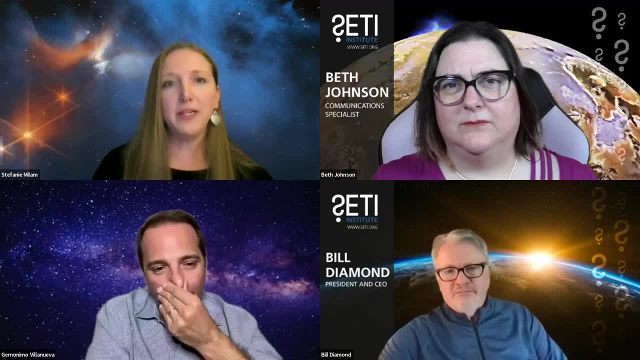 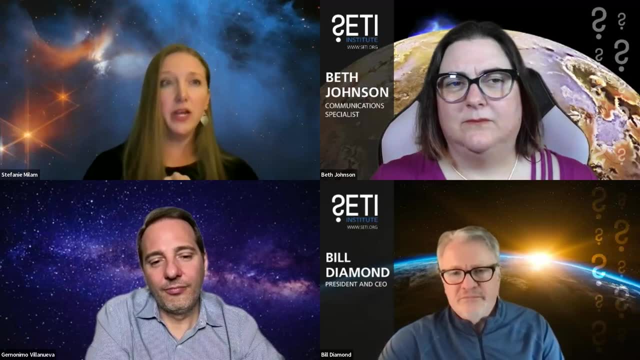 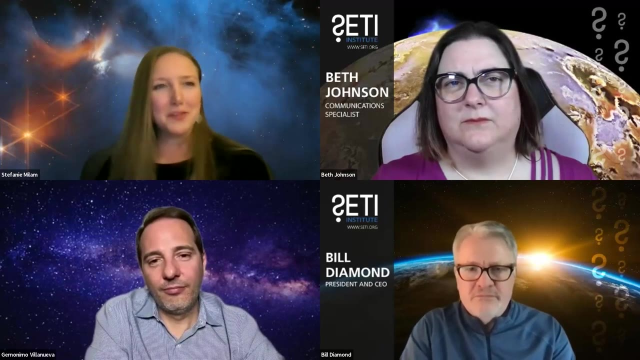 you know, the satellites around our giant planets. all of this is actually little bits of information that's telling us that that chemistry was much more evolved than what we can see remotely, And so, if we can put that into context of other planetary systems that are forming, that, 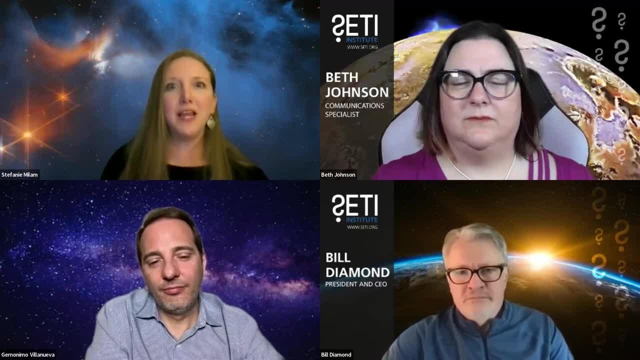 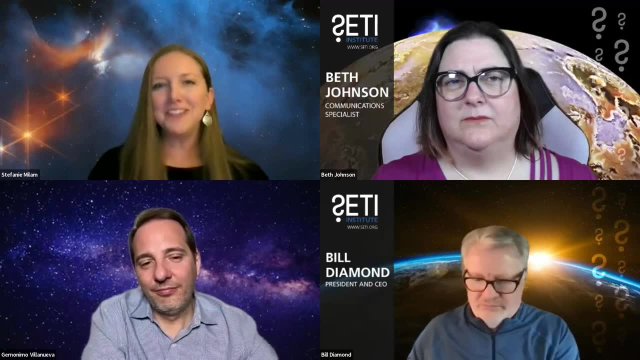 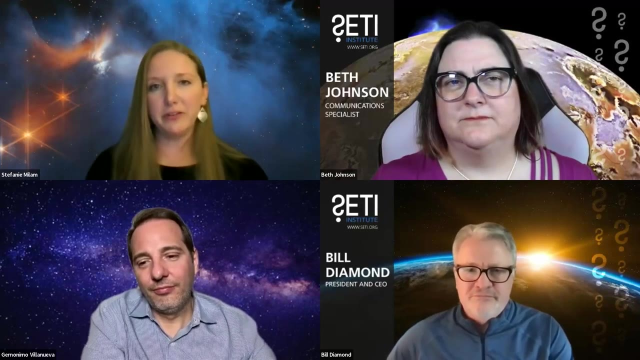 means that that chemistry is ubiquitous. It's going to be the same in any one of these systems which suggest that maybe these seeds, these prebiotic molecules, the simple chemistry that maybe collectively becomes something more complex, can actually rain down on other atmospheres. 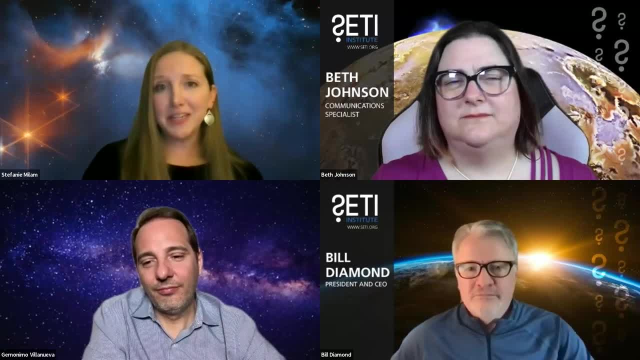 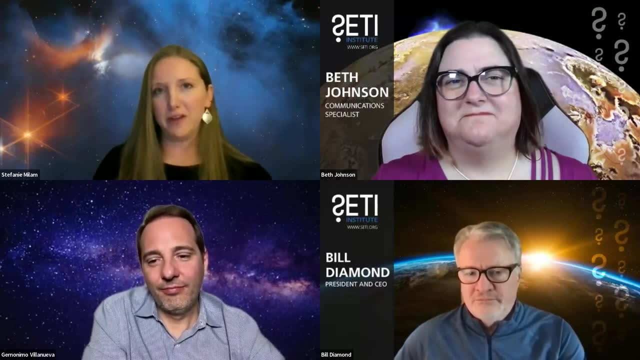 Other terrestrial planets and maybe that's going to initiate life somewhere else. And that's the kind of you know path that we like to follow, to see if we can follow that evolution and understand how the chemistry evolves, how biology could evolve and potentially, how life could evolve. 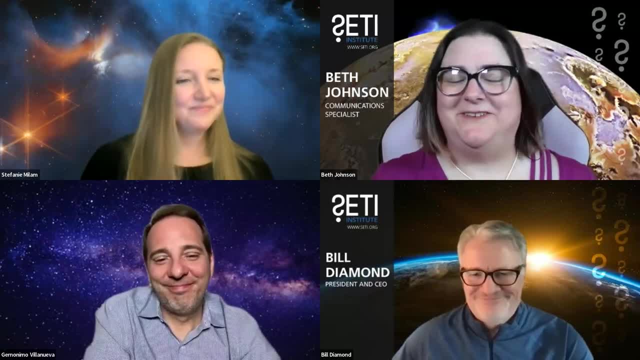 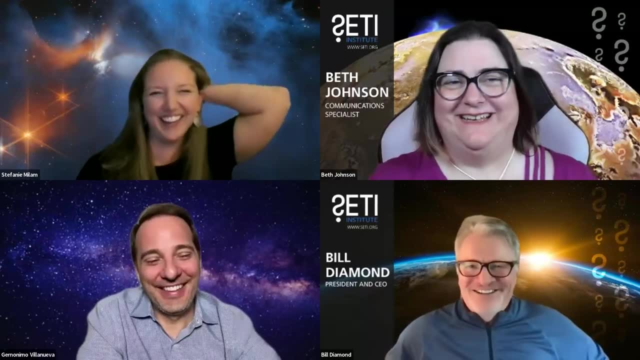 Wow, Thank you, Geronimo. do you have anything to add to that amazing answer? No, that was inspiring, Thank you. All right, Ben, do you have anything to add to that amazing answer? No, that was, that was inspiring, Thank you. 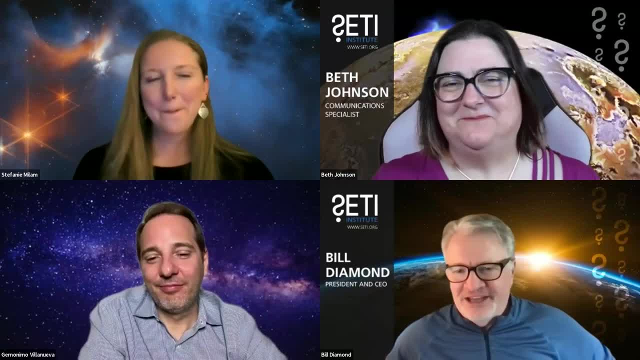 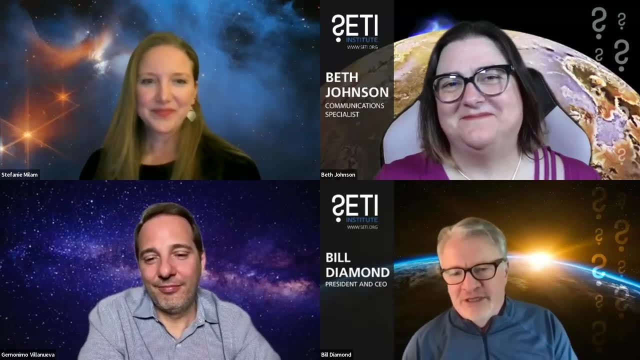 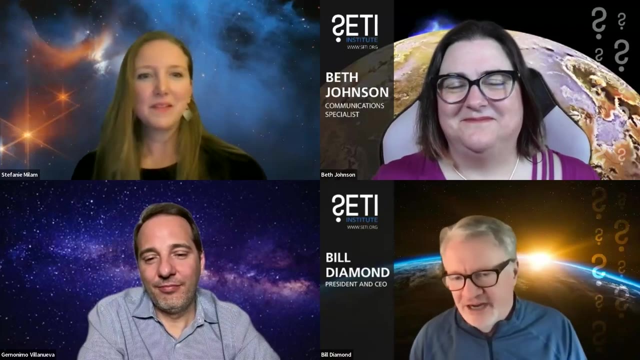 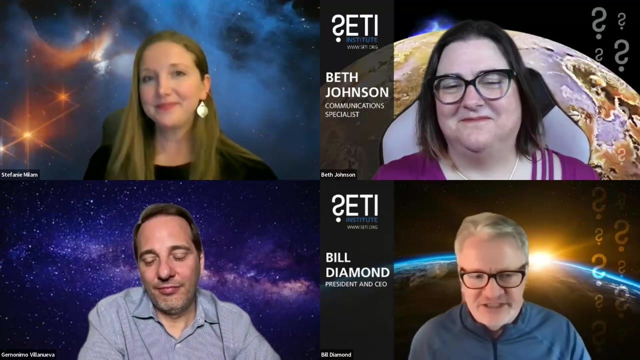 Bill over to you. Great. Well, thank you, Beth, And thank you Stephanie. Thank you, Geronimo, That was absolutely fantastic And you know, I think that what's so exciting about James Webb, about the work that both of you are doing and your many colleagues, is, you know, SETI, as an endeavor looks for signs of technology that nature doesn't produce as a proxy for life and intelligence. 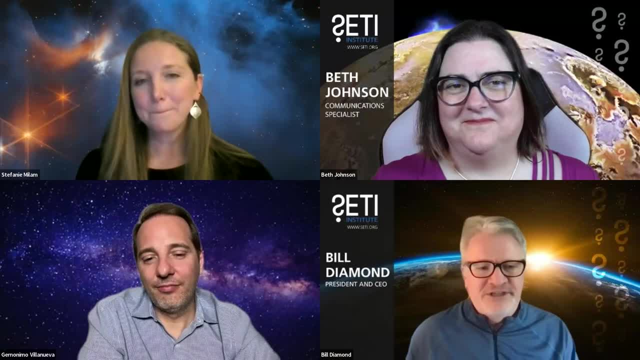 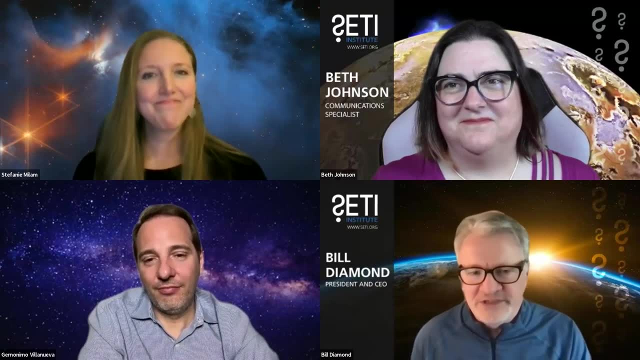 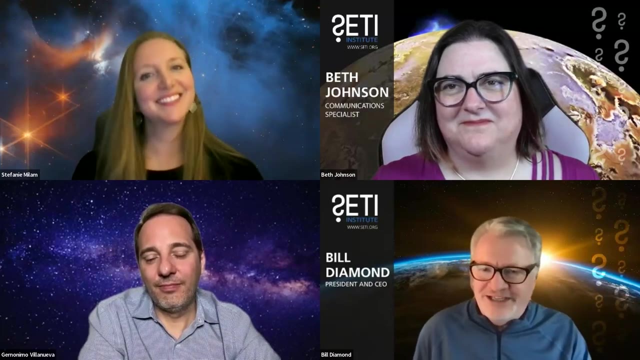 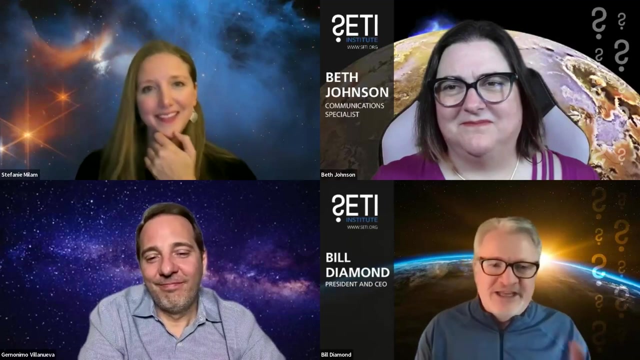 It's sort of a definitive technique, should it yield results, Astrobiology doesn't. Astrobiology, which we also undertake at the Institute, really looks for life in its most basic forms, And I think the study of life, or the potential for life, in our own solar system is so fascinating because if we find examples of life in different parts of our own solar system, particularly with a unique biogenesis you know, to me that suggests, in terms of the question of 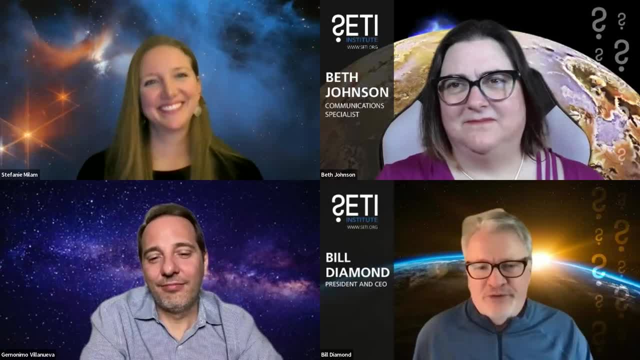 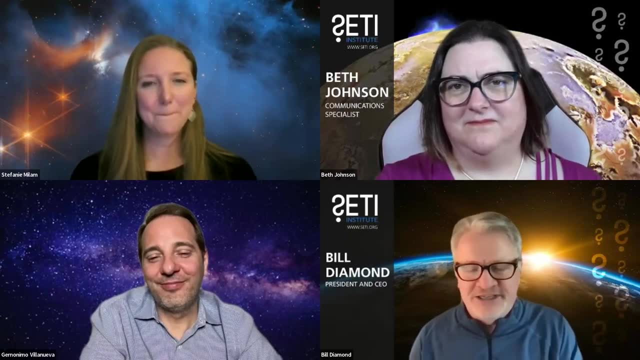 are we alone in the universe is sort of game over, right? I have a quote that I'm known for saying that someday I will be born out on this. But my quote is that I think the most remarkable thing about life may be that it's not so remarkable after all. 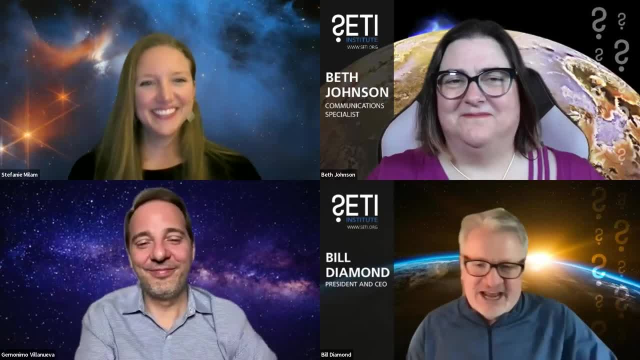 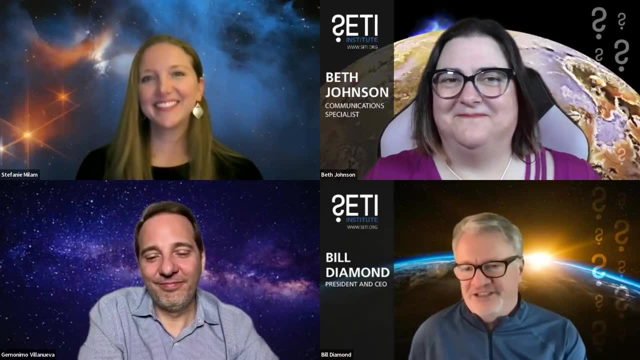 That life may be as natural a phenomenon and as natural a byproduct of the formation of planets, as the formation of planets is a natural byproduct of the birth of stars. So who knows? But it's so exciting the work you're doing. 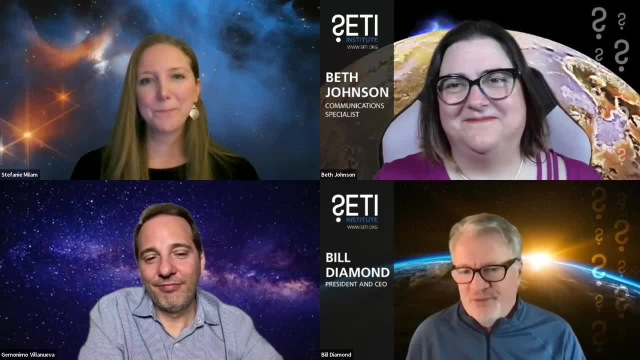 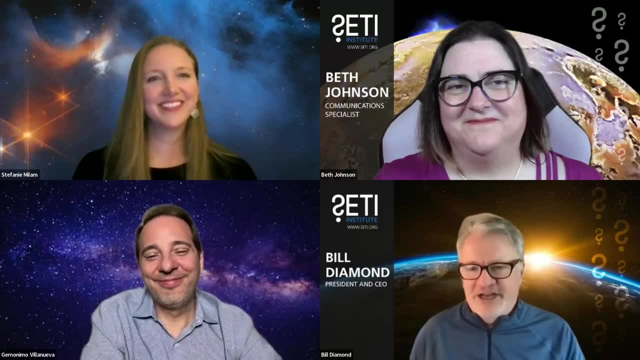 And you know you both did such wonderful jobs explaining what you're doing, explaining the science, explaining the capabilities of your work, The capabilities of James Webb Geronimo. I thought your visualizations and animations were fantastic. I mean, spectroscopy is such a powerful tool and technique. 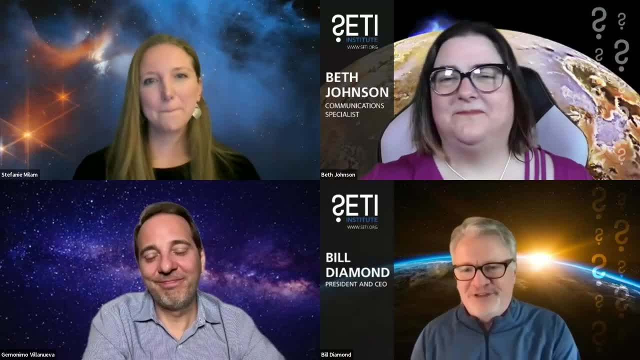 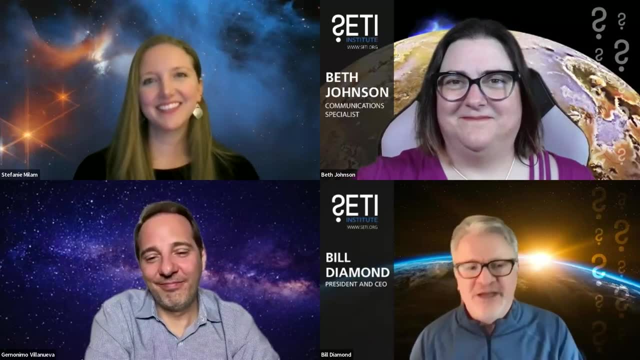 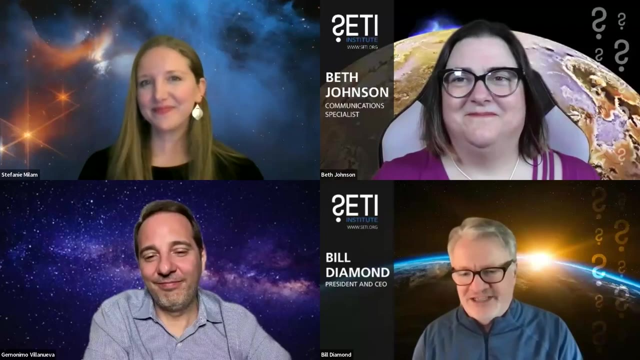 And yet, you know, it's not the most straightforward thing for people to understand how it works. But I thought your animations and visualizations did a great job of explaining spectroscopy and how much we can understand about. you know even distant worlds and environments through that technique. 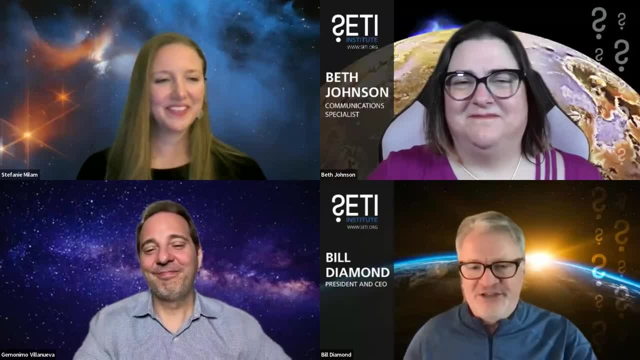 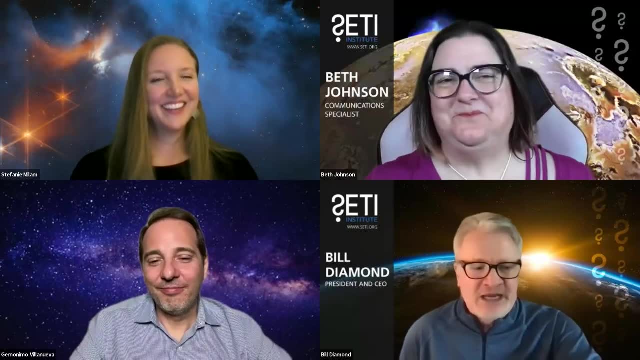 So, And again, you both just did a spectacular job. I did have one question that I'm going to take advantage of my spot here at the end to ask you. It's a question you know. I've been working, actually, with Jim Green, who's the former chief scientist at NASA. 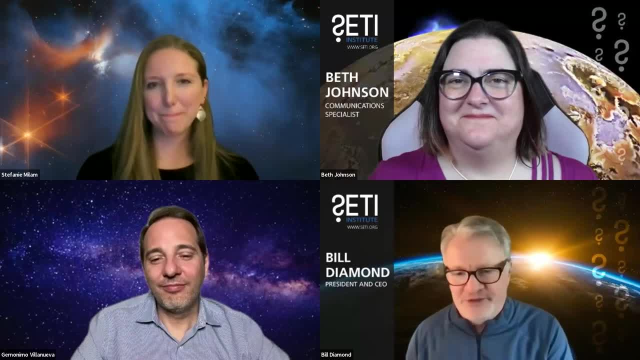 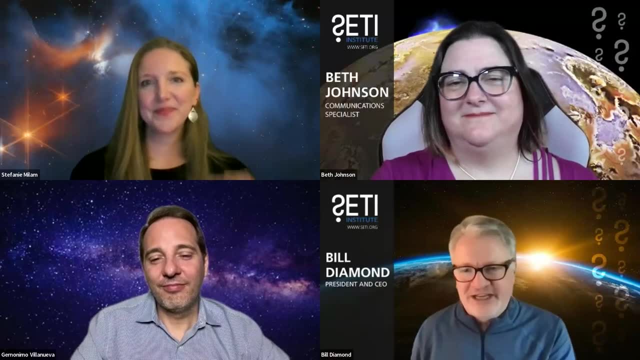 He's now retired and he's doing some talks and we were going over some of the different ways of looking for life in the universe, you know, in situ, sending instruments to places, or remote sensing like James Webb or SETI. Look at that. 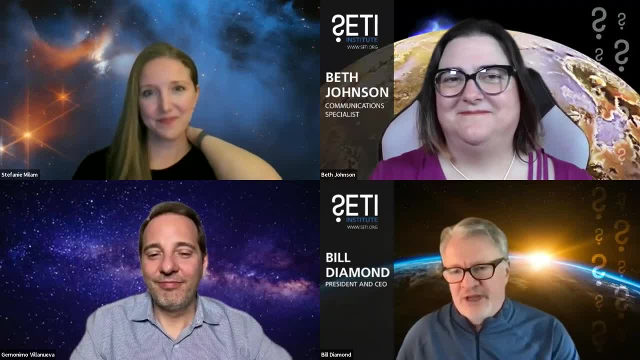 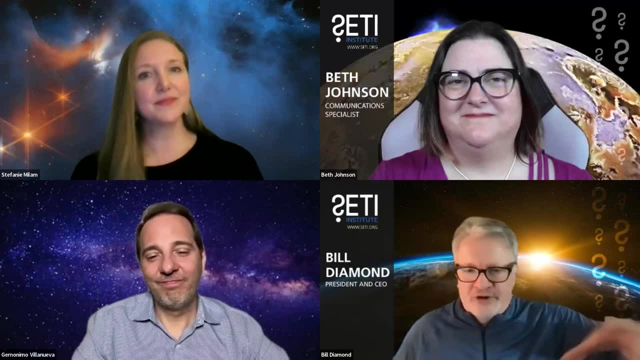 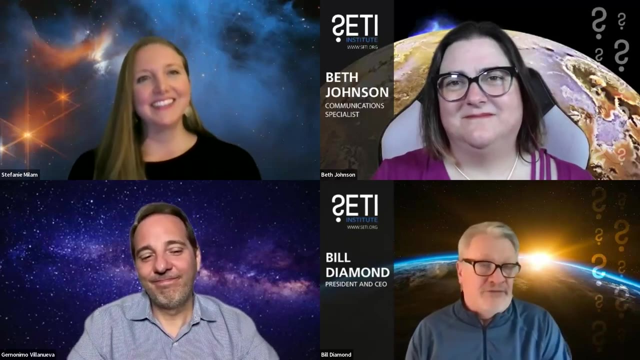 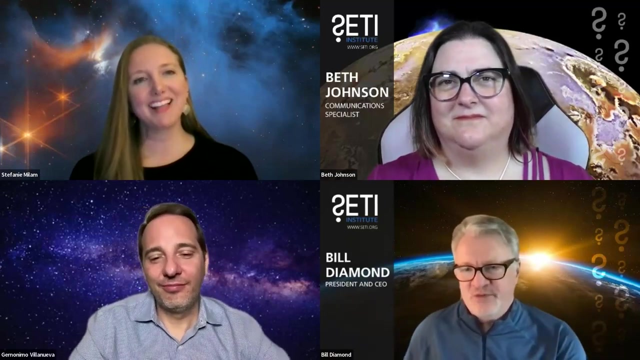 He's looking for science, of technology And, in terms of James Webb and its ability to probe exoplanet atmospheres, about how far out in light years from you know our own solar system, can that technique be effectively used And if you know the answer to this, you know roughly how many candidate planets might there be in that parameter space for James Webb? 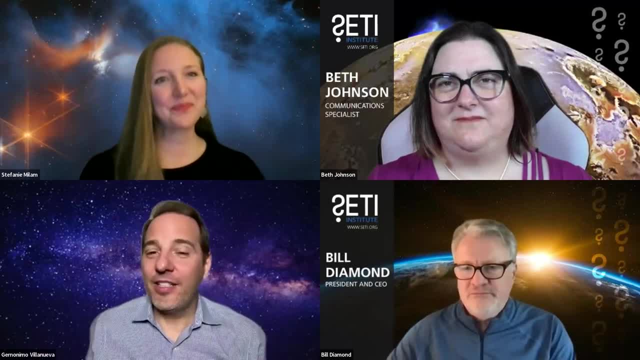 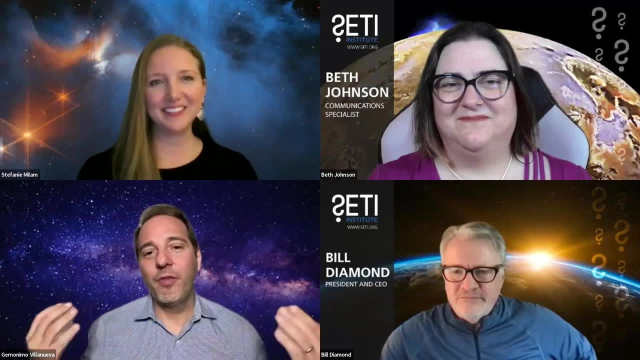 Yeah, So that's again I can tell that's the toughest question. So we always normally- I mean, I'm not an expert but I can say that normally- we always focus on the 50 parsecs And you know, that is kind of our, but it's still within our confines- 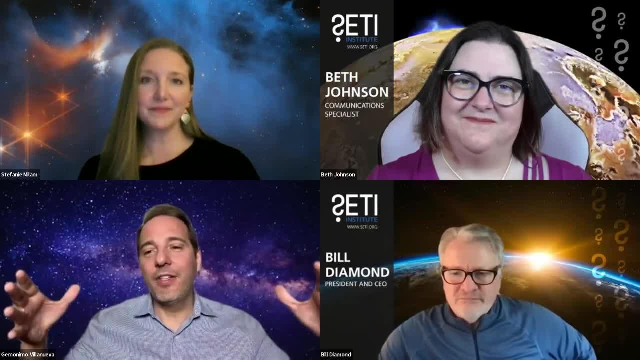 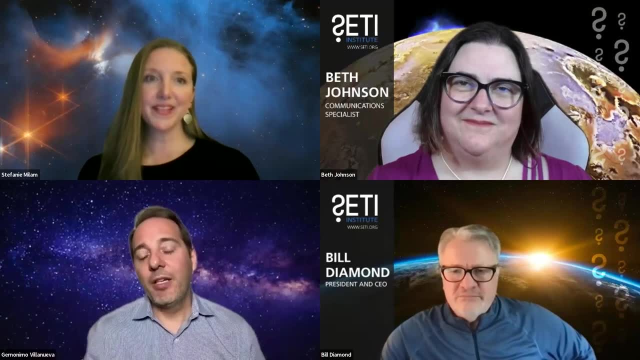 And normally, you know, normally that is a definition where we can do spectroscopy at a certain sensitivity that we can see molecules perhaps. But then, for example, when you're thinking about something like coronagraphy, even with the future observatories, even if we build habitable wars in 2040, something, 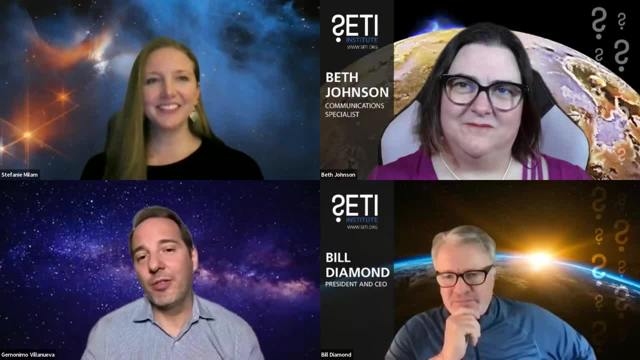 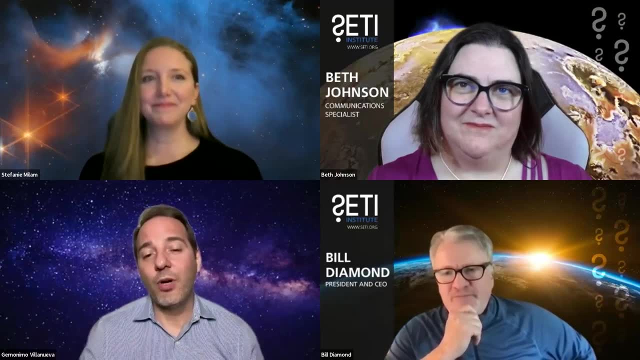 We are heavily focusing on the near neighborhood, which is even shorter, maybe 20 parsecs or even 10 parsecs, And then your number of candidate planets. for doing that, it becomes very restrictive, But that's why we are working a lot on the future surveys. 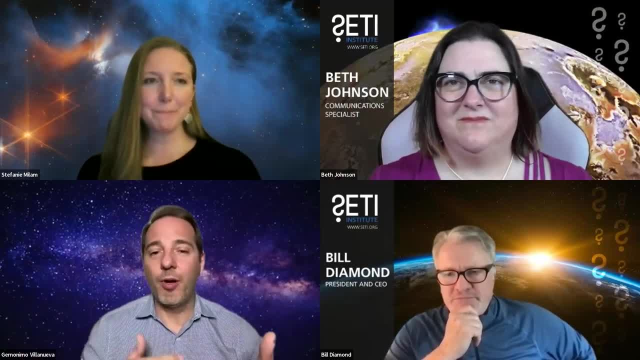 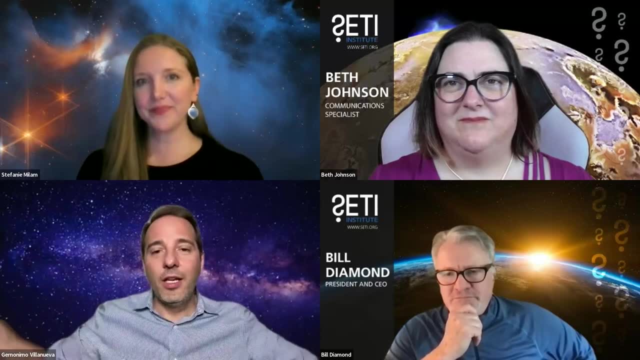 I mean we, you know we have right now we are. every time we learn more about planets we are getting more sensitive to do radio velocity but also transverse spectroscopy, So getting bigger surveys, more coverage in the sky, so we can increase the survey of more available planets. 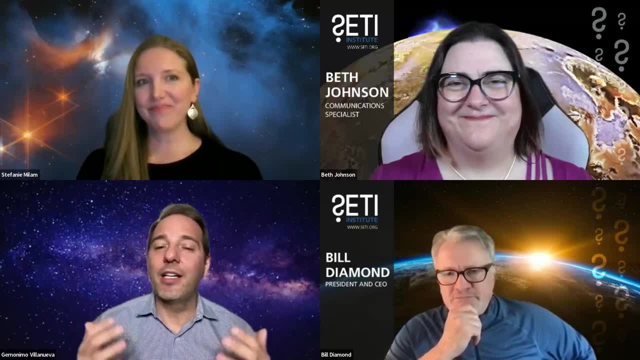 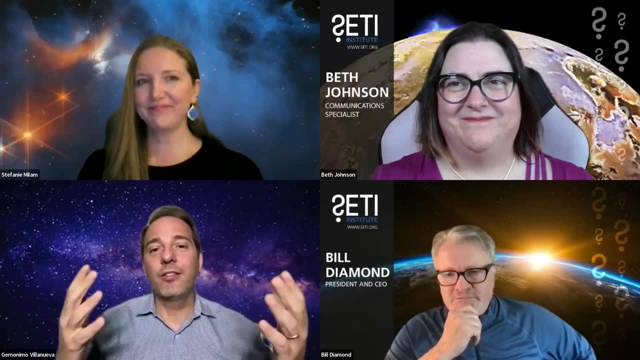 So there's a lot of hope that we can detect more planets and include that survey. But yeah, it's going to be restrictive in the amount of photos we can get And also the. you know, coronagraphy requires certain distances so you can mask the light in the right way. 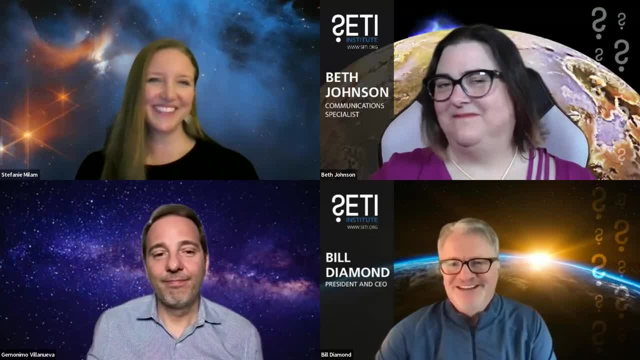 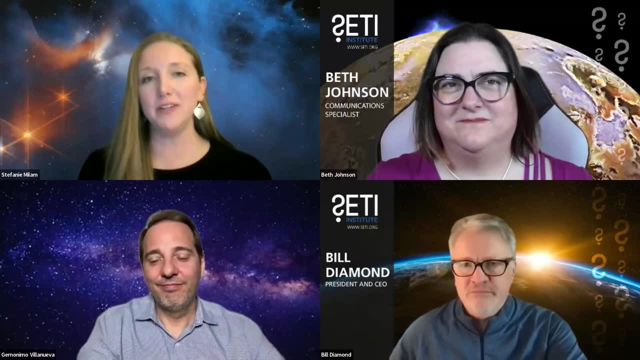 Yeah, yeah, Great. Thank you very much, Stefan. I don't know if you had anything to add to that, but Yeah, I just wanted to say that I think your first point was actually why we do what we do in parallel in the Planetary Science Division. 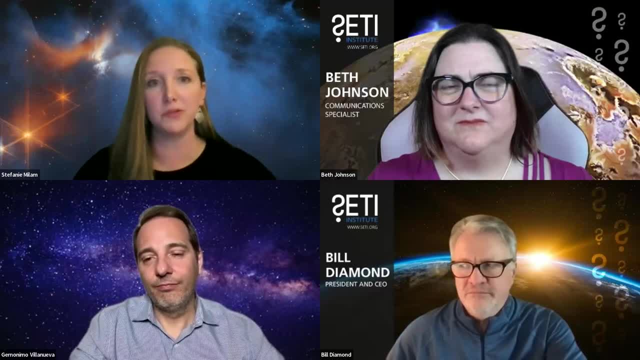 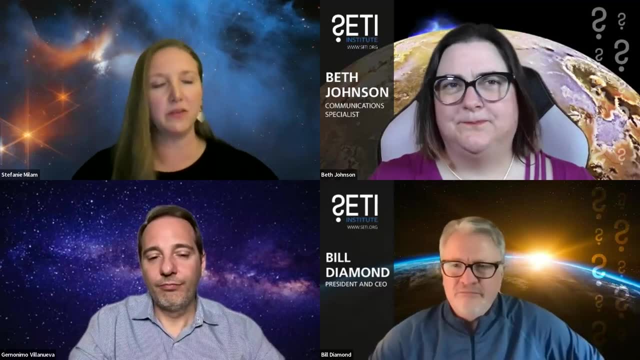 And that's what we're doing actually. We're doing exploration as best we can closer to home, Because once we find that first evidence, that is the smoking gun and it means that it's going to give us a lot of insight into what we should or could be looking for elsewhere. 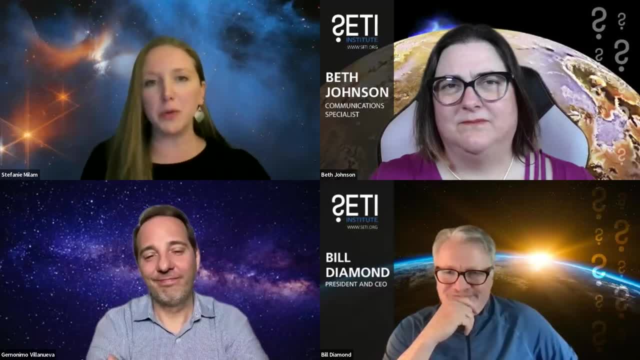 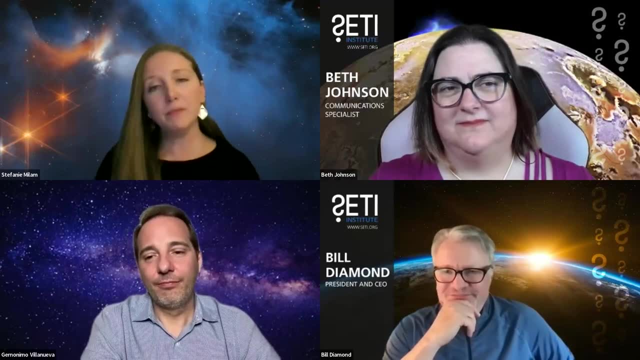 Right now we are. we're very biased on what we're looking for. We're looking for Earth 2.0.. We want water, We want methane, We want carbon monoxide, carbon dioxide- But who's to say that's the environment that we will. we will actually have life in. 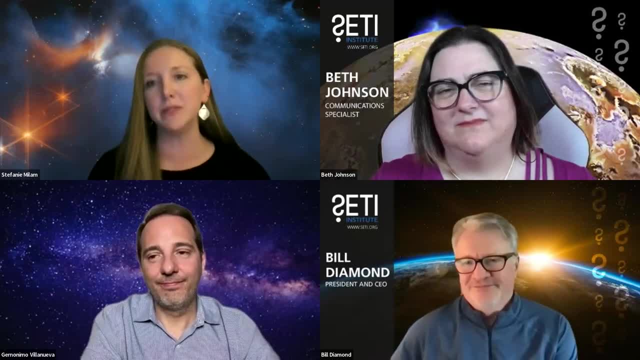 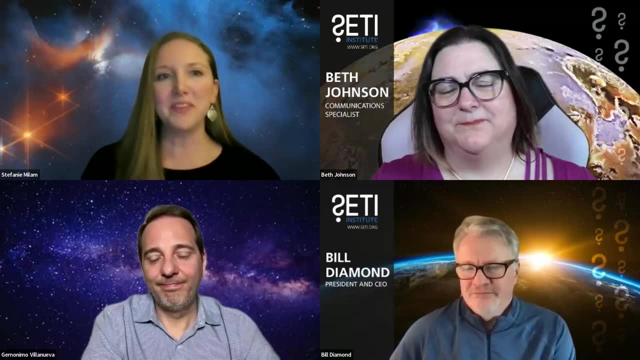 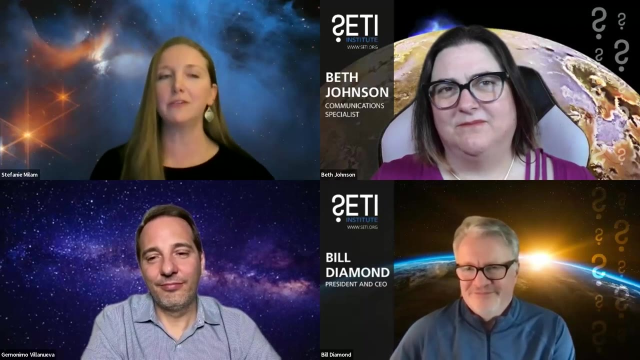 So I think the diversity that we have across the solar system And the environments is going to be very revealing And you know, we even find that here on Earth. So only time will tell. but we're definitely doing the best we can to enhance and enable exploration across the solar system, but also peer deeper into planets around other stars. 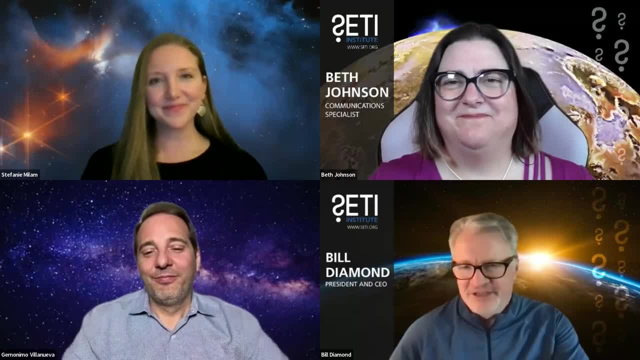 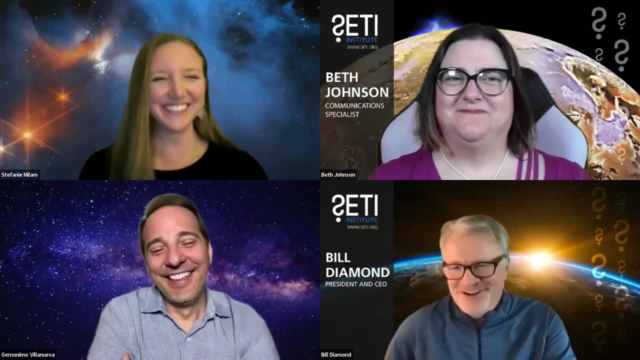 Yeah, yeah, Well, you know you said earlier. as a chemist, you know you follow the chemistry right. So bankers and investors follow the money, Chemists follow the chemistry, Biologists follow the biologists, Physicists and spectroscopists follow the light. 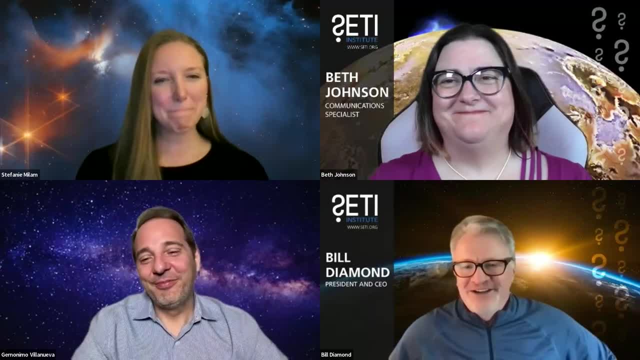 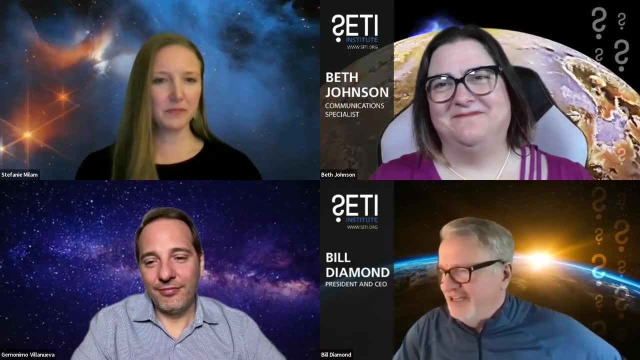 So anyway, but I think what you're saying is absolutely right. Well, again, it was really really marvelous. We had an interesting question that has popped up a couple of times. Somebody named Utsav- and I'm sorry if I'm not pronouncing that correctly- has asked a few times what science groups are needed for the study of astronomy. 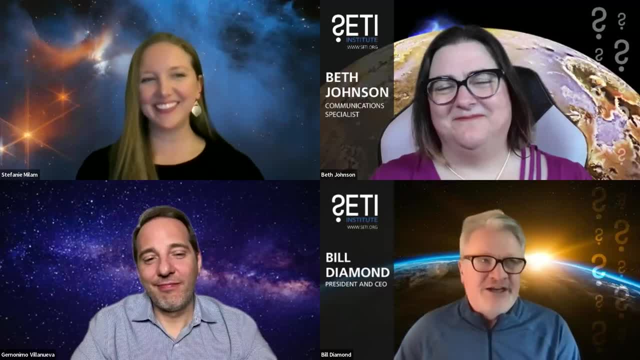 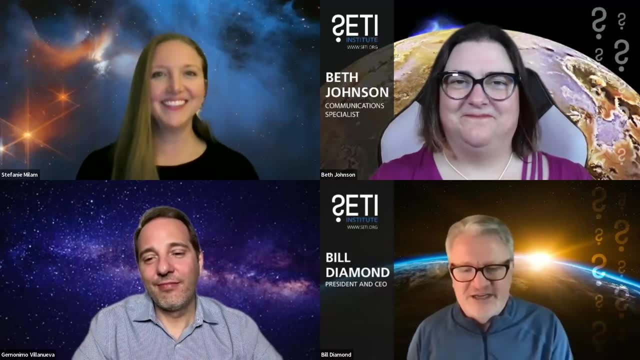 I mean it's a great question from my point of view. You know, the answer is a little bit like a cross section of the science at the CEDS. It's a cross section of the science at the SETI Institute. We have over 100 scientists and affiliates at the Institute who cover 23 separate disciplines of science. 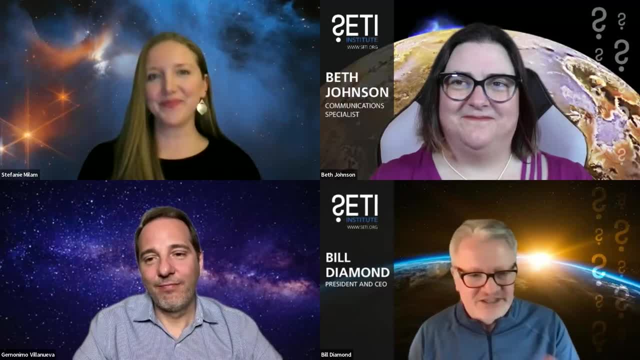 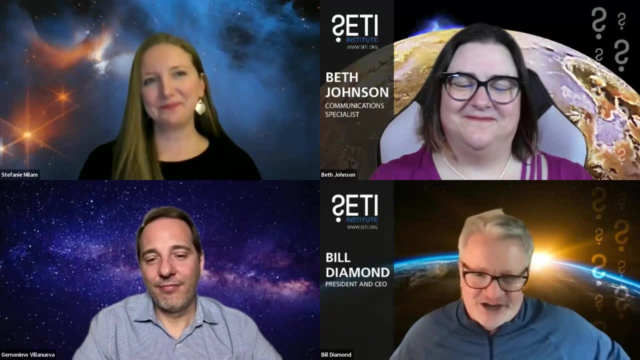 And the same is true, of course, for NASA and elsewhere. you know from chemistry, physics, astronomy, astrophysics, cosmology, biology, microbiology, planetary science, geology, geophysics. you know, on and on and on it goes. 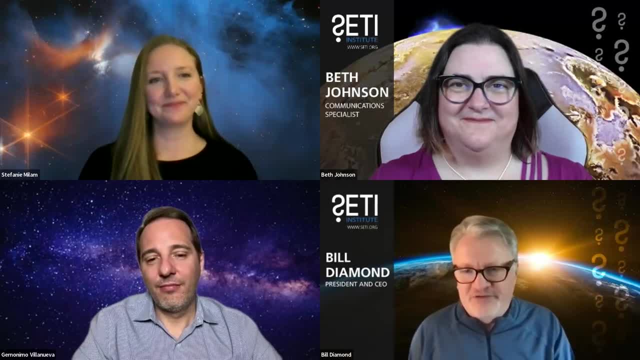 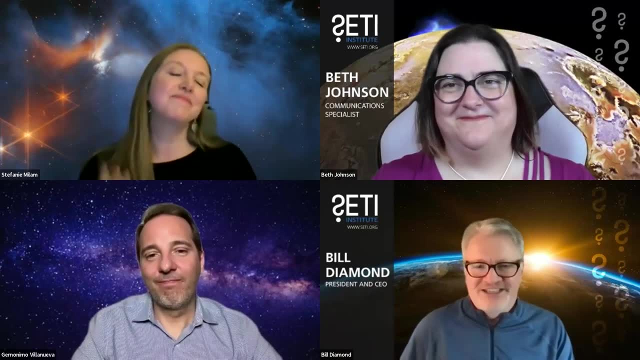 And you know when you're trying to answer a question as big and profound as you know: is there life elsewhere in the universe? Well, I think the answer is yes, there is life. There are all aspects of the natural sciences, and probably some of the unnatural sciences and humanitarian sciences, to answer these questions. 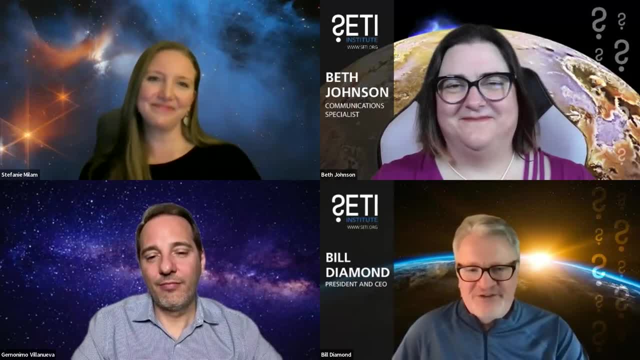 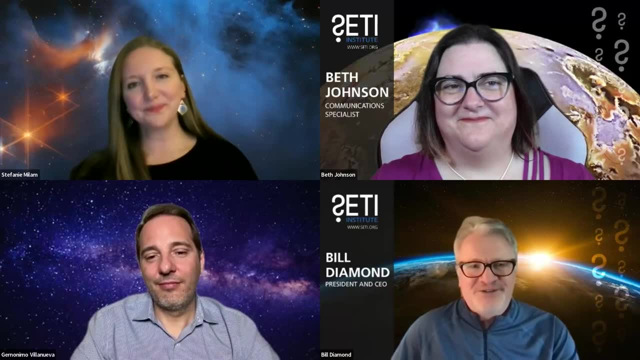 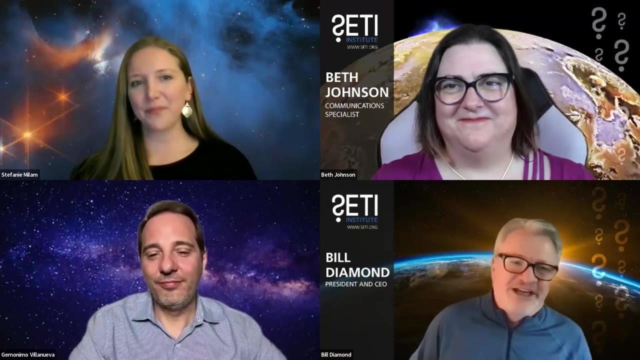 So it is a good question, but there isn't one part of the natural sciences that isn't exploited in some way in this pursuit. So, but lots of great questions from the audience, And we did have people, as normally form, from all over the place watching us tonight. 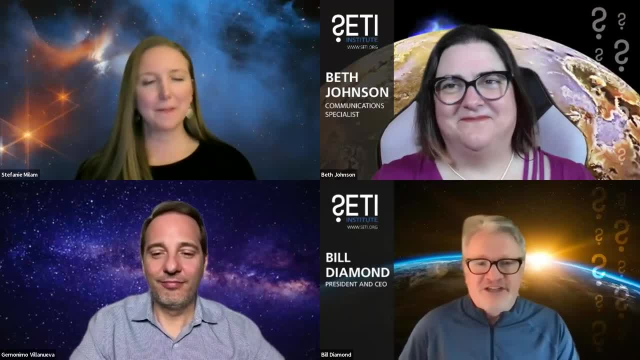 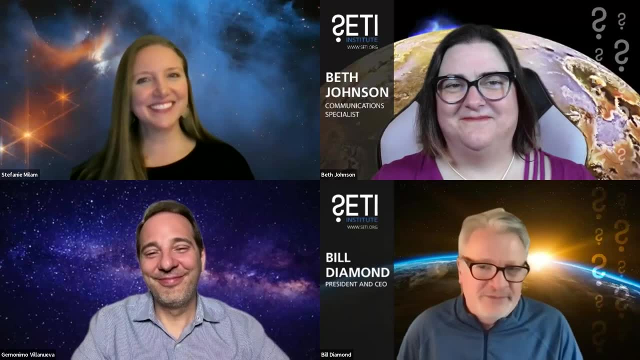 In terms of countries. I think there's a lot of questions, but it's a great question, Thank you. We had folks from Mexico, Canada, the US, Australia, India, Japan, Spain, Argentina. probably, Geronimo, some of your family. 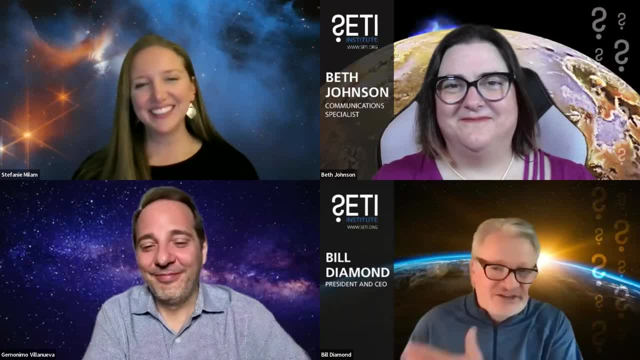 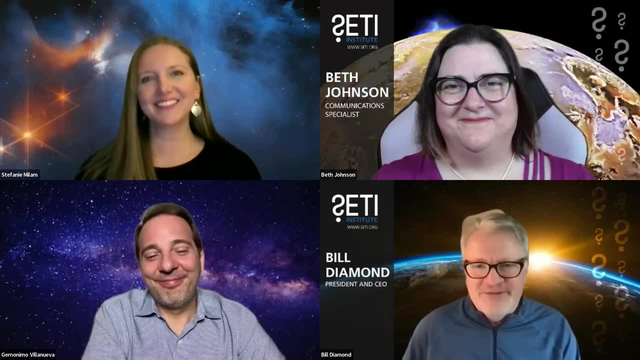 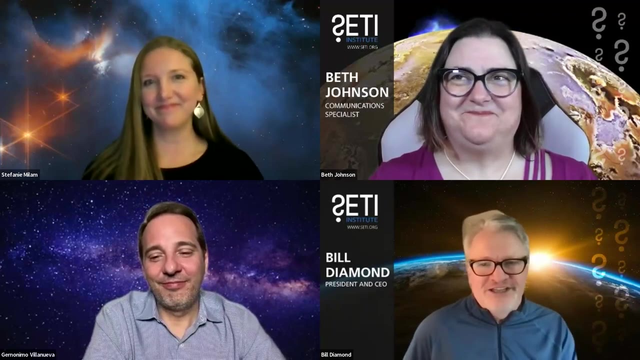 I don't know, And in Chile someone who was actually from watching from the Atacama, And I've been to the Atacama with our own NASA Astrobiology Institute team And I have to say it's one of the most spectacular and stunning and otherworldly places on this earth. 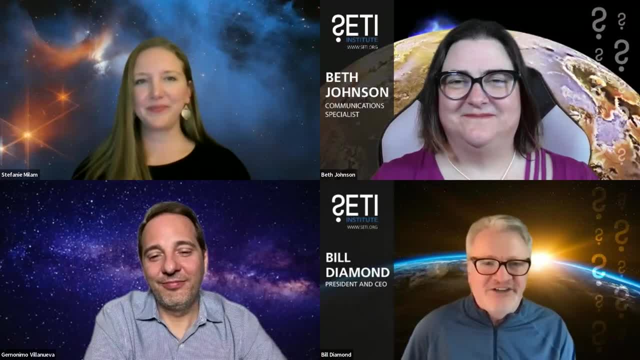 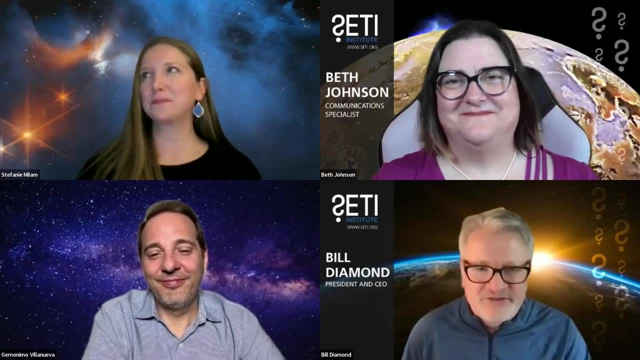 We've had friends from Brazil And Greece And the United Kingdom And from the United States All over the place: California, Arizona, Hawaii, Indiana, New York, Texas. Actually, somebody from Texas said they were watching from Houston. 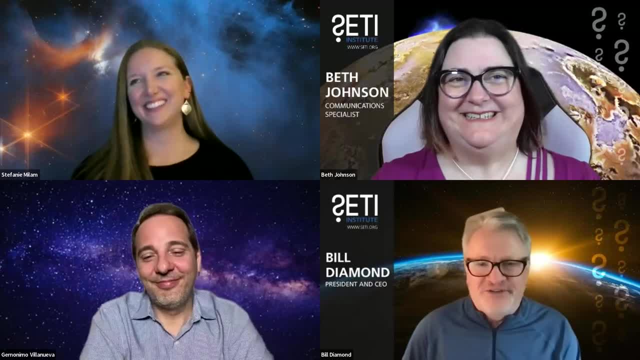 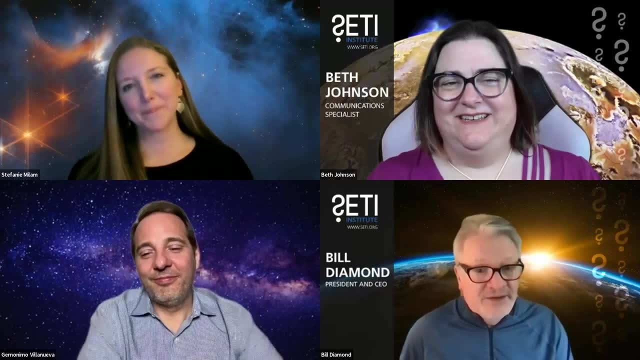 And there wasn't a problem, which was good: Colorado, Pennsylvania, New Jersey, New Hampshire, Washington, Illinois, Vermont, Oregon, Minnesota, New Mexico, Wisconsin, Florida, Georgia And Louisiana, And if I didn't mention where you're watching from, it's probably because you didn't say. 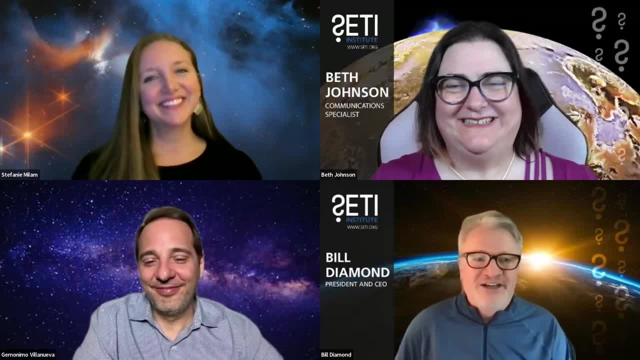 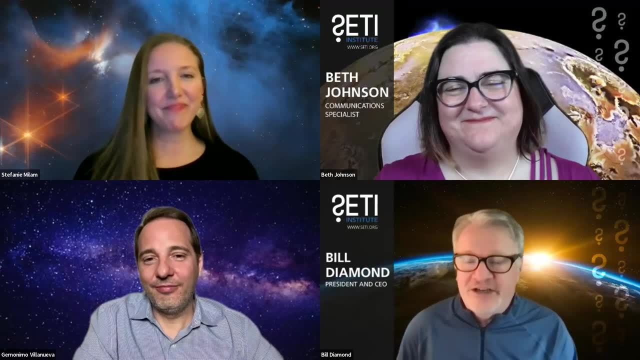 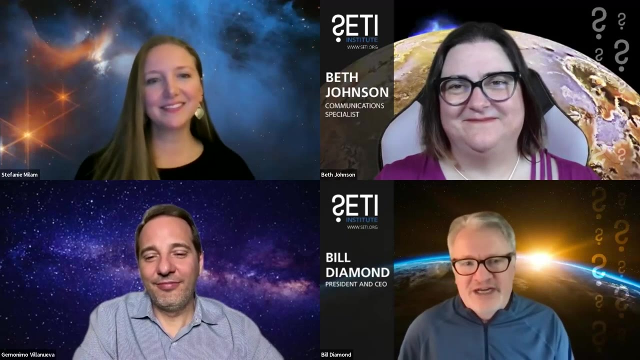 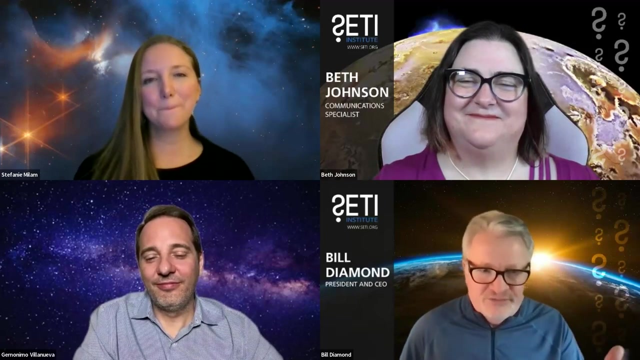 So next time do let us know where you're watching from. We always like to understand Who's watching and where you're from. But before closing tonight's event, just a reminder again that the SETI Talks is a production of the SETI Institute, where nonprofit research and education institution and our mission is to lead humanity's quest to understand the origins and prevalence of life and intelligence in the universe and to share this knowledge with all of you, with the whole world. 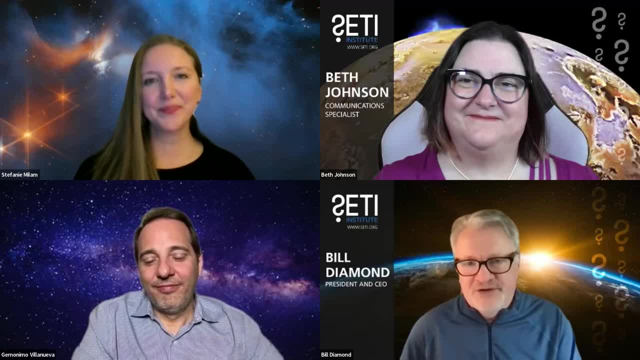 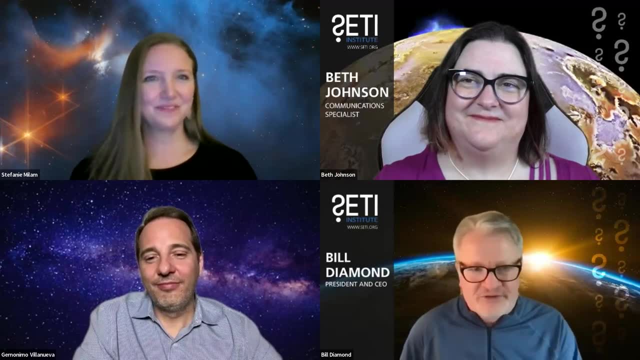 Our SETI Talks lecture series is supported in part by donations from the public, from friends of science like you. We bring these lectures and other events to you at no cost, but we're always grateful for any kind of donation that allows us to continue bringing the stories of extraordinary science and exploration to you. 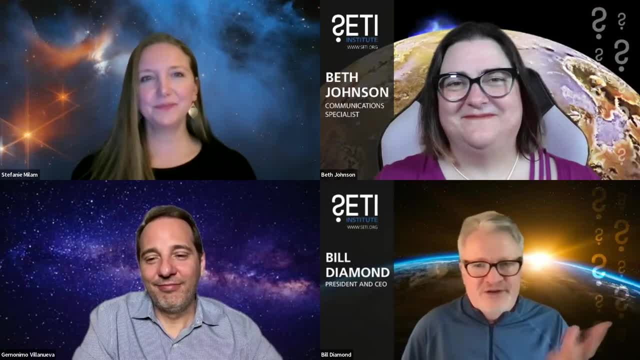 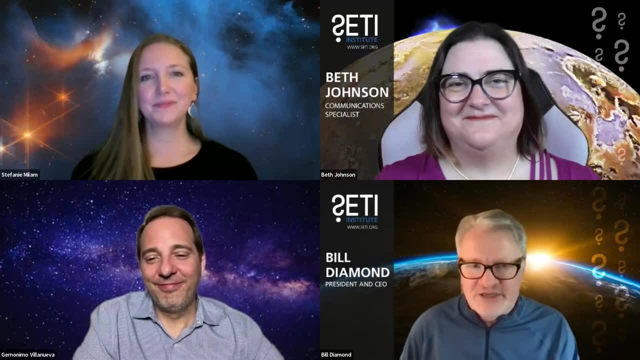 So again, visit us at SETIorg for more information about that. You can sign up for our newsletter, You can make a donation if you're inclined, or just peruse our website, where there's loads of stories and information about the wide-ranging and extraordinary work we do every day to answer one of science's most profound questions. 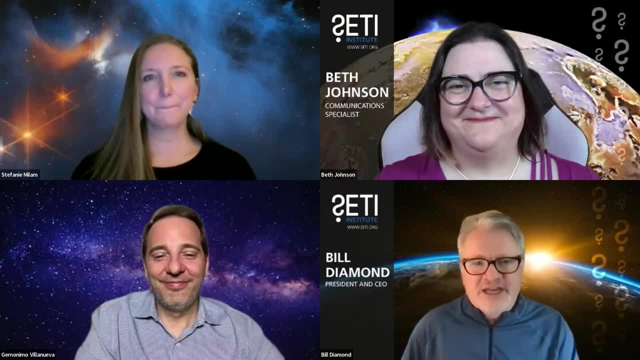 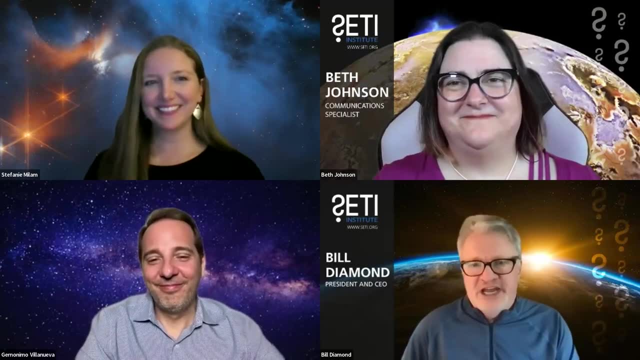 Are we alone? Are we alone? Are we alone in the whole world? Are we alone in the universe? So thanks again to all of you for being with us tonight, And thanks again to our moderator and tonight's amazing guests. I also want to thank Rebecca Lee, Jasmine, Frank Simon here at the Institute, all of whom make our SETI Talks series possible. 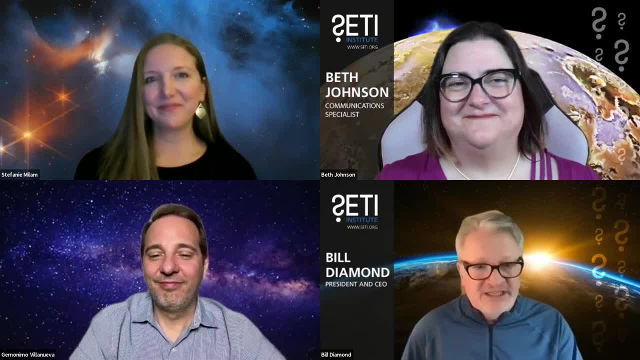 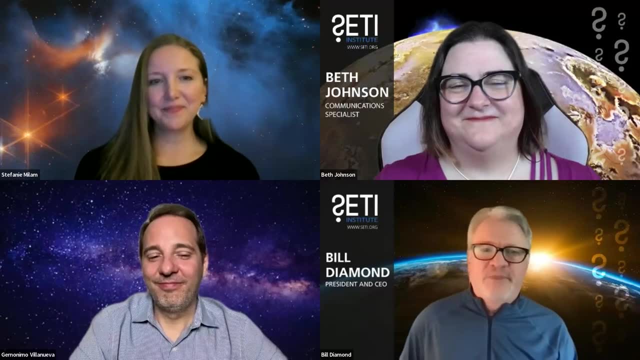 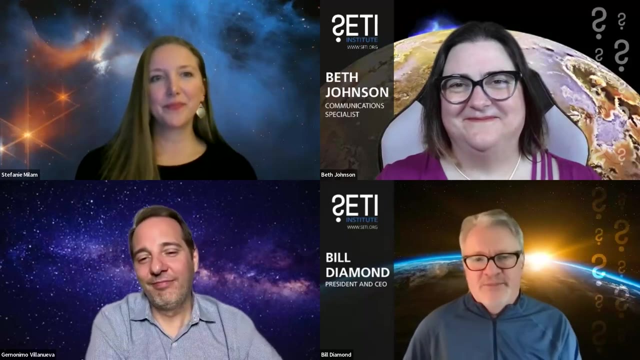 And all our SETI Talks, lectures and panel discussions are on our YouTube channel, along with vast amounts of other amazing material. So do take an opportunity to visit the SETI Institute's YouTube channel. You'll find all kinds of amazing talks here. Again, this talk will be posted on our YouTube channel in a matter of days. 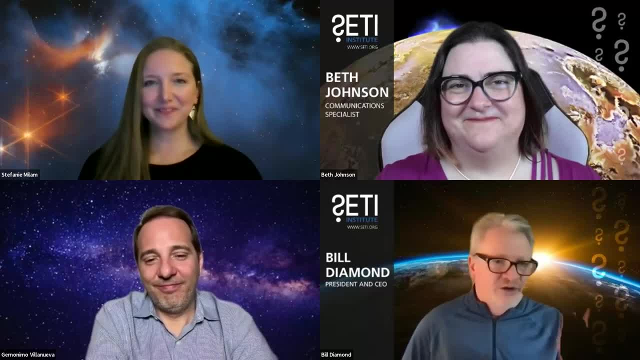 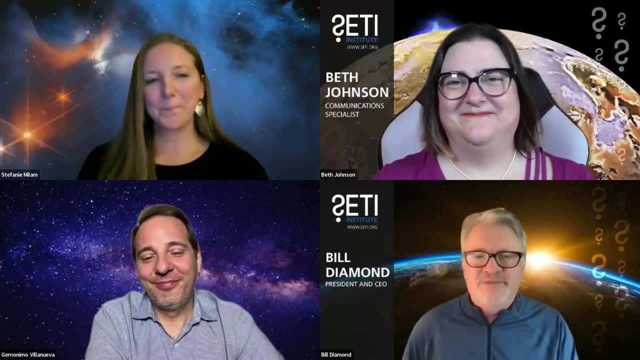 Remember that the work we do at the Institute is for all of humankind. Don't just stand by and watch. Come on and join us at SETIorg and get involved. The Search for Light Beyond Earth is a journey of ultimate discovery. We invite you to come along. 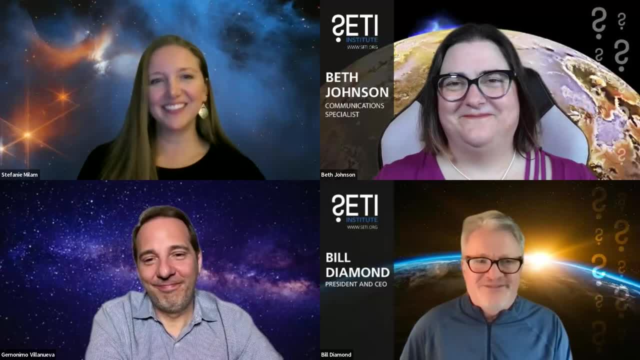 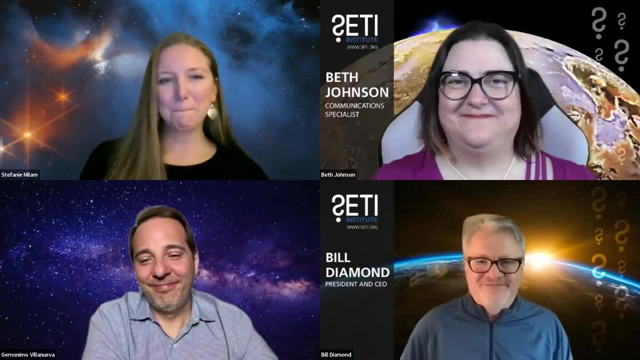 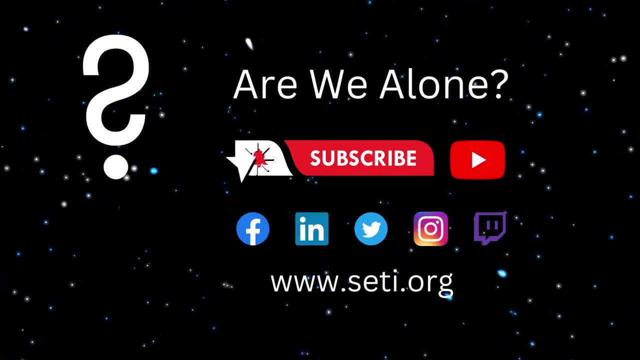 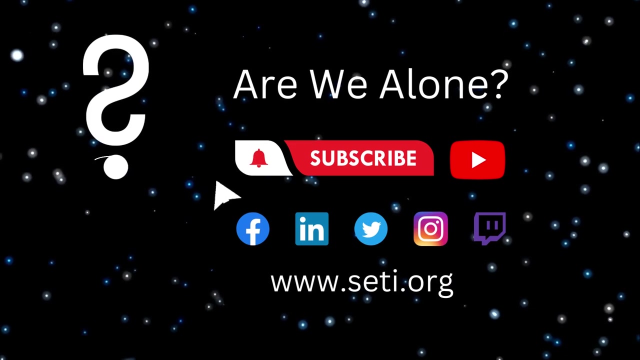 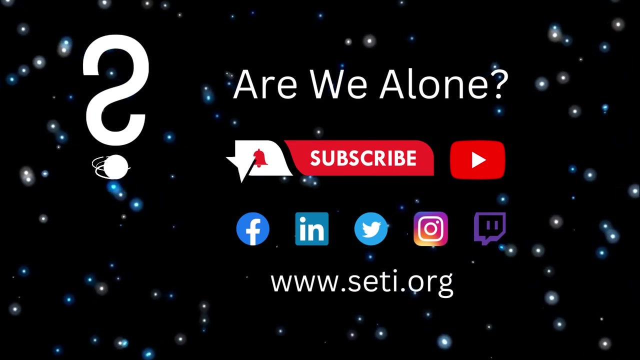 We thank you for being with us and we look forward to seeing you next time. Thanks so much. Thank you everyone. Thank you.